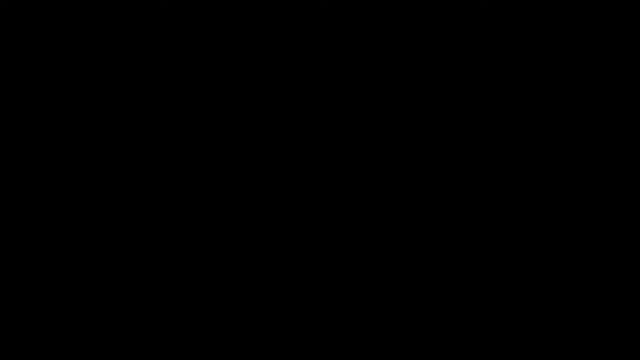 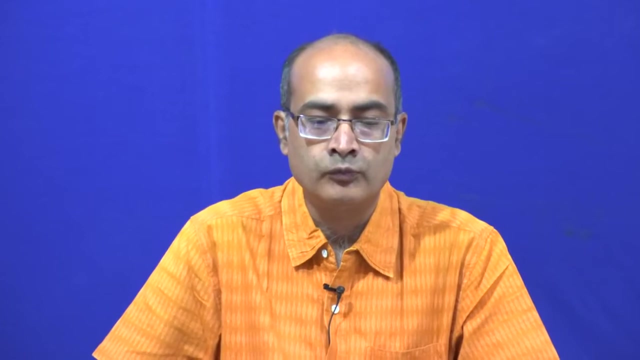 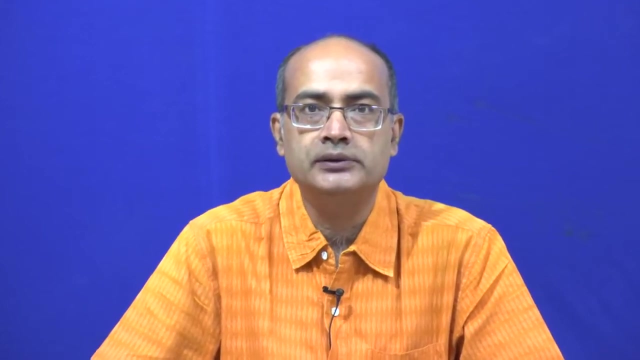 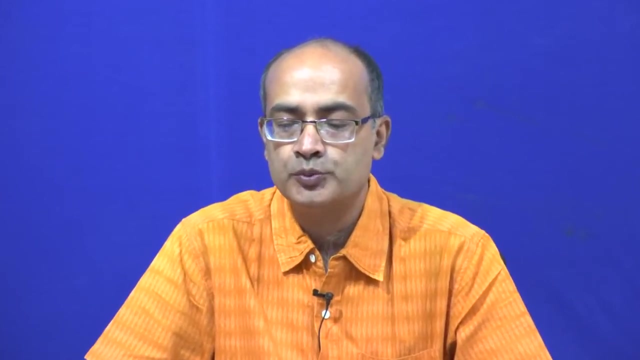 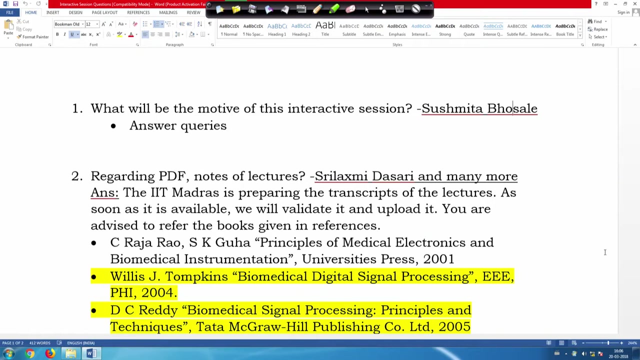 Good afternoon. So for the biomedical signal processing, that course, we have taken the first course you would like to take. it is from Sushmita Vosley that the question is: what will be the motive of this interactive session, that the reason or the motivation behind this interactive? 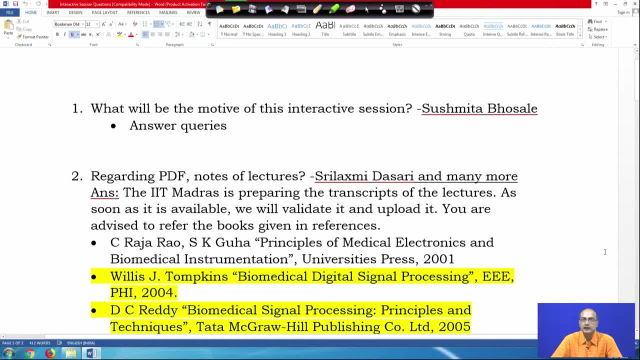 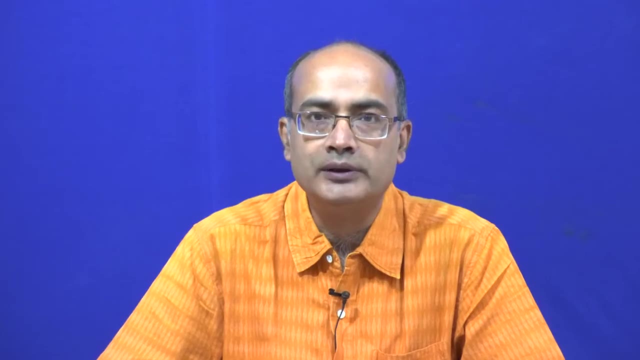 session is to increase the interaction and to understand the participants and their needs in a better way. When I take these lectures as a tutor of this course, I find very handicapped, because when I take this class in regular teaching mode then I can see the faces of 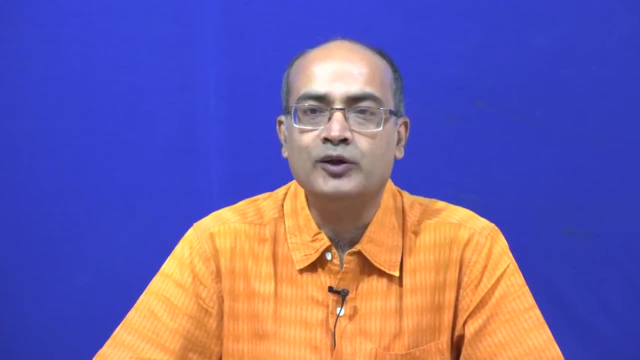 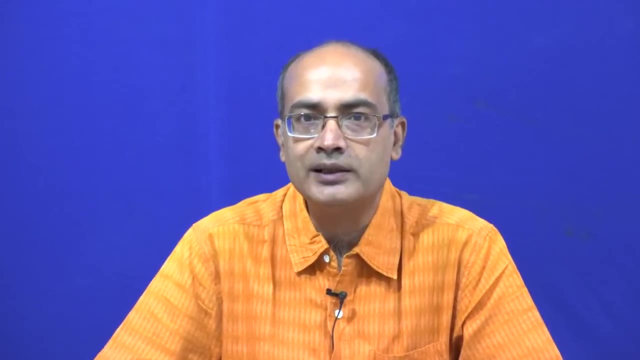 my participants and it automatically gives me a feedback that how much they are appreciating it. if they have difficulty in understanding, I need to spend more time and to explain it more. if they are getting bored because pace is low, then I can speed it up. So I continue. 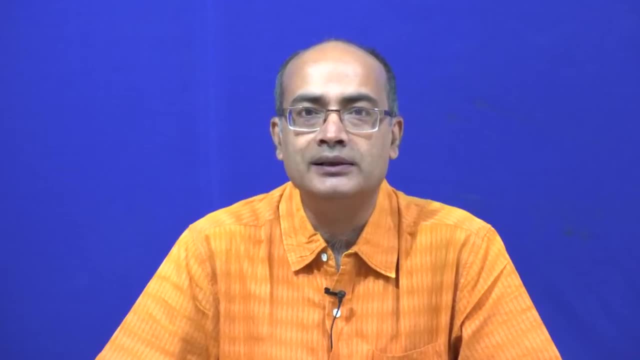 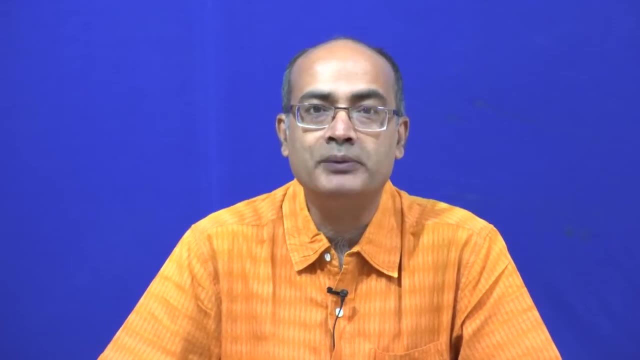 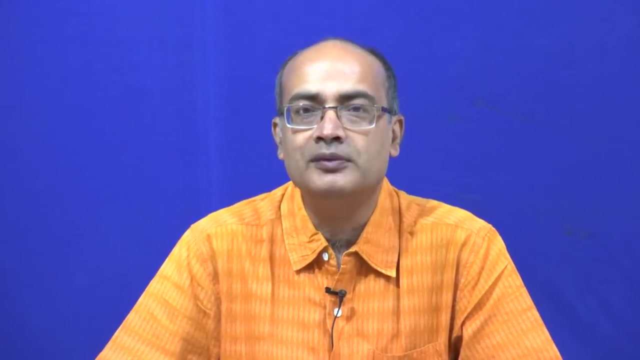 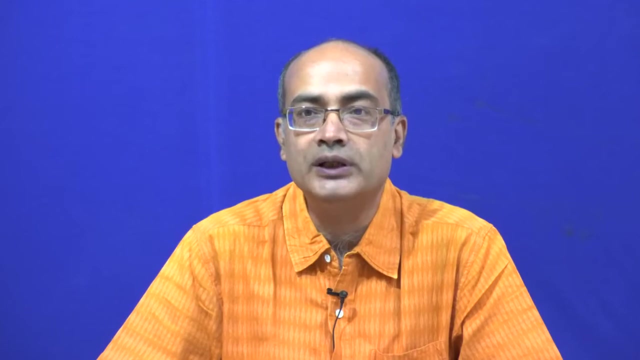 continuously keep on getting that feedback and that has become as an habit that I take it for granted. but when I am taking this online course, I could actually realize that that is not all the time which we can take for granted. We do not get the feedback that how the participants are feeling about that course. 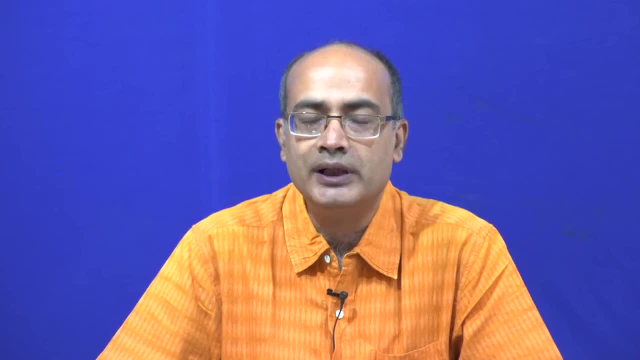 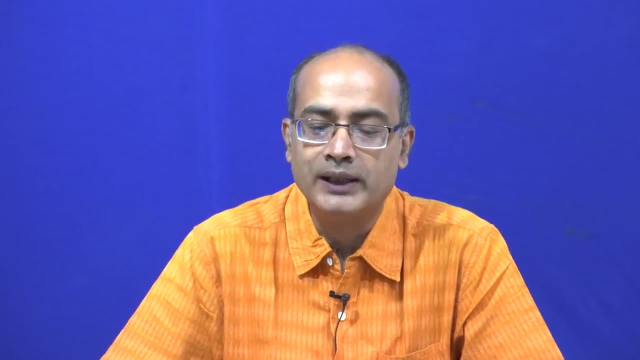 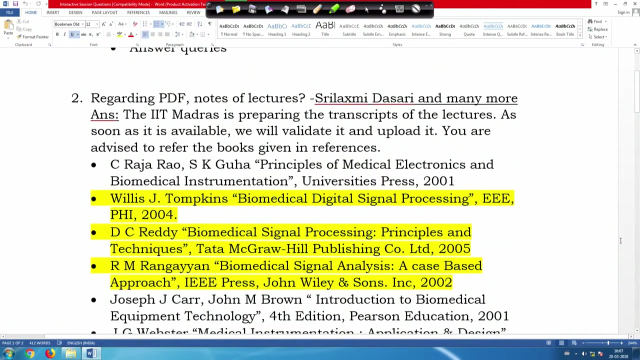 So I think it gives me an opportunity to interact with you and to reply to your queries. So that is the motive behind this interactive session. Next, I would like to go for the second question by Srilakshmi Dasari and many more people. 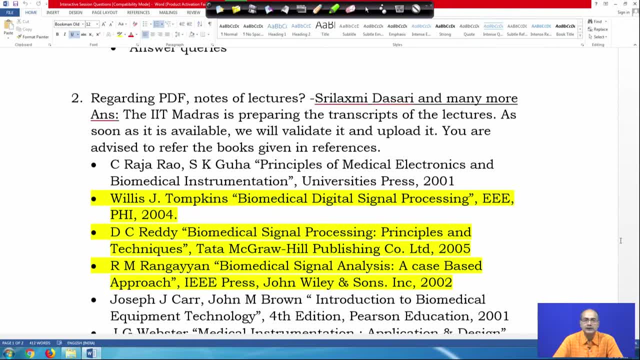 in the forum asked for that. this question That: what about the notes of the lecture and pdf Now preparing the? the transcript is in the agenda of that NPTEL team and IIT Madras it is looking for it. they are in the process of preparing it. once that is available, that. 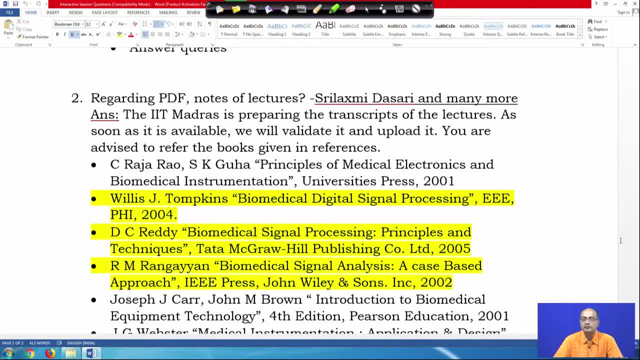 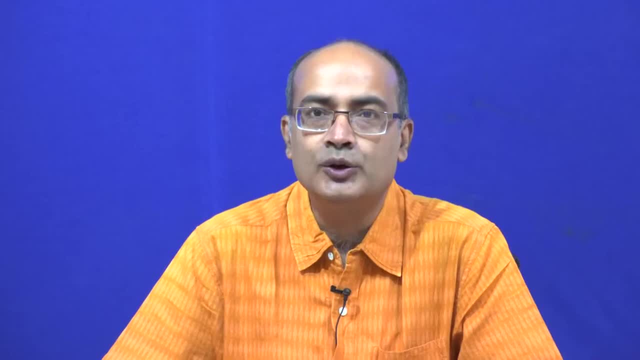 would be shared with you. but till that time it is prepared, I think that we have enough time to go through that, the class lecture or the video lecture. what we take that is just providing you a cursor to what to read and what is the sequence to maintain. 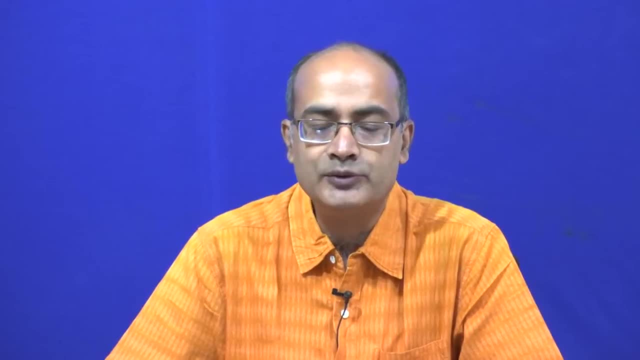 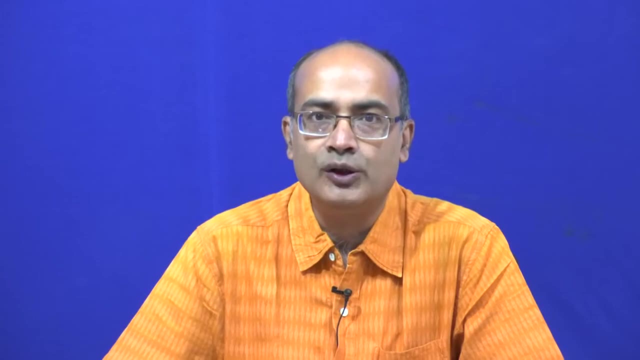 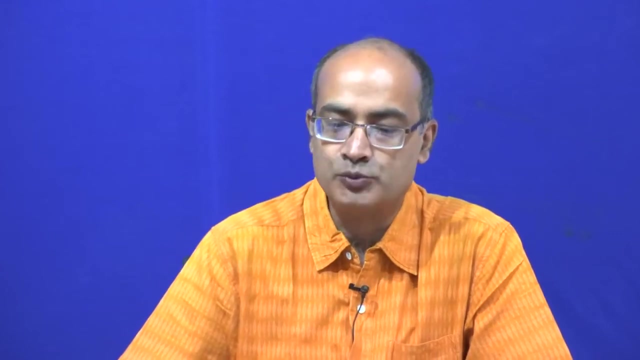 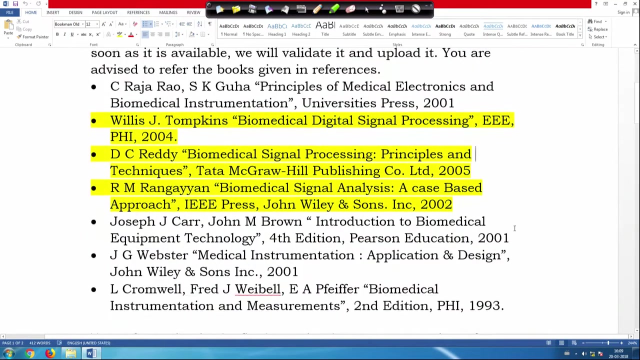 And in the beginning of the course I have provided actually a number of references. When I went for that second phase also, I have provided actually the references and added one more name. I would like to go through them once more. So if you look at this courses, that out of them, that that three books, we have highlighted. 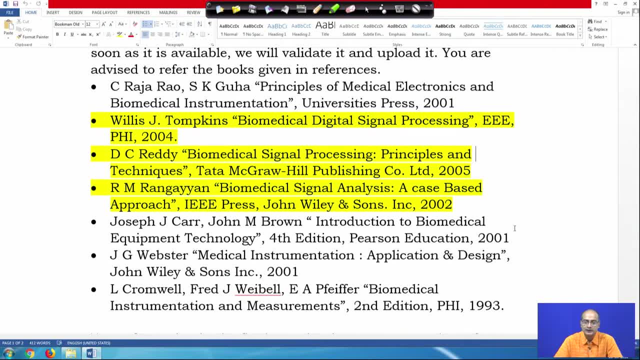 here all of them. they are on biomedical signal processing, that all three of them can actually be a text for these lecture course. So. So I think if you can get it from the library it would be the best. If you cannot get it, then I think you can buy it from the shop. 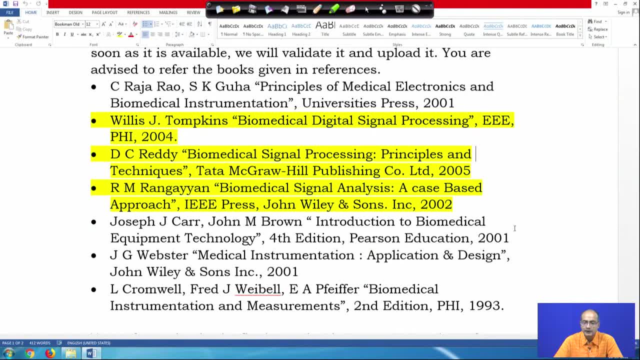 We have the Indian edition and the international edition. they are pretty affordable. So if you do not get them in the library, then I would suggest that you should try to get them one copy of one of these book which can actually provide you that the notes or 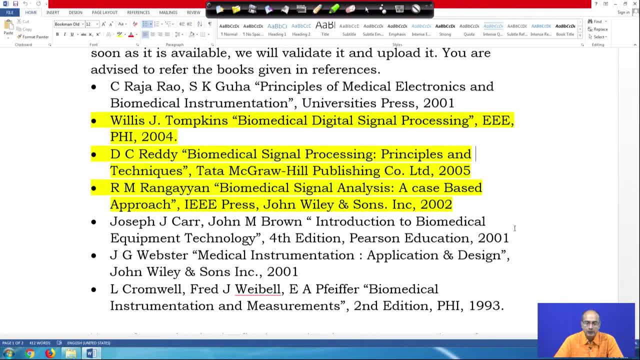 what you are looking for, The powerpoint presentation or the transcript. it can at best give you some bullet points. It cannot give you the whole story. So if you want to get the mastery over the subject, you have to go through some book. 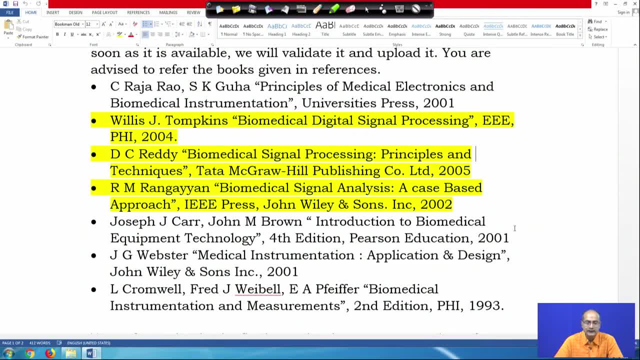 and you can get it. You can choose any one of these book and the three books I have highlighted here: one by William J Tomkin, the other one is by D C Reddy and third one is by R M Rangayan. 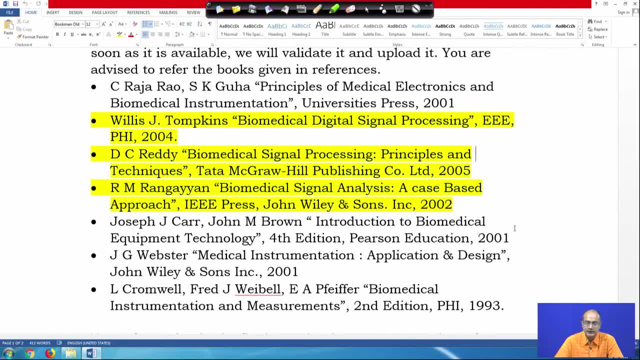 All three of them can serve the purpose of text and the other books they are. I would say they are the references. ok, So time to time they may be required, But if you have one of these three books then you can get it. 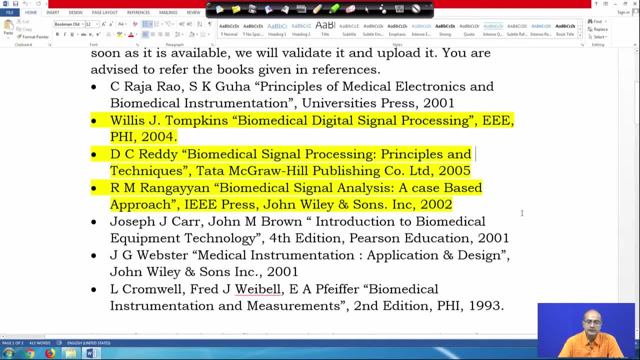 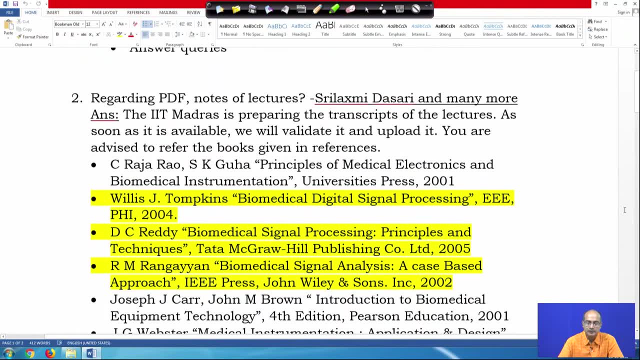 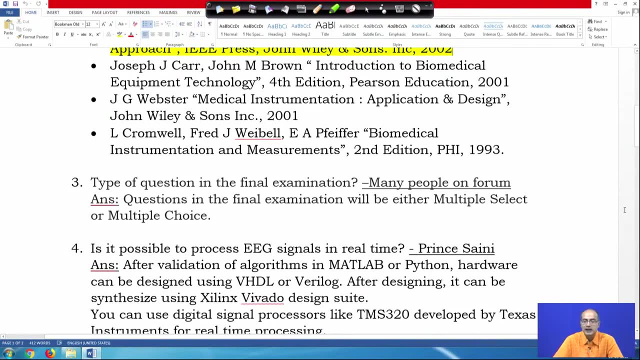 If you have one of these three books- R M Rangayan, D C Reddy or that Professor Tomkin, then I think your purpose would be solved. Next, I think many more people has asked in the forum as well as in that Google sheet. 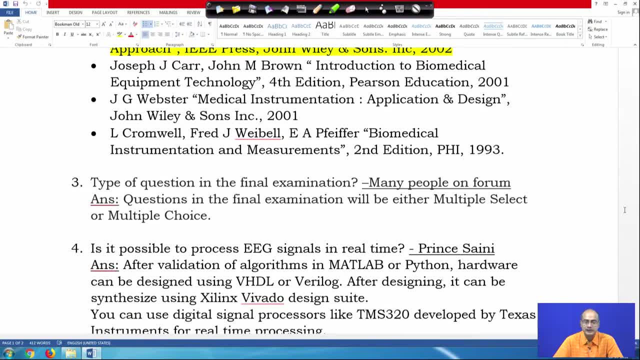 that what would be the type of questions in the final exam? It would be exactly 6.. Similar to the questions you are getting in the assignment. In the assignment you are given number of questions and all of them they are multiple selection or multiple choice. 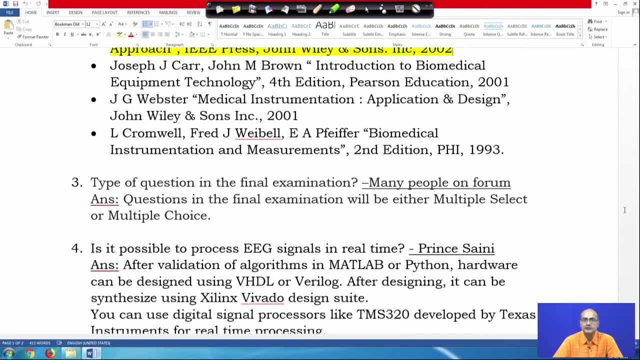 So you will get just similar kind of questions. So either from your knowledge you need to select one or multiple of them, or sometimes you need to do some small computation. 7. Using calculator to get the right number before you make the selection. 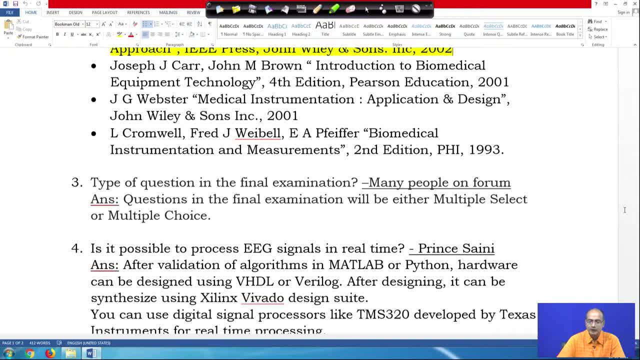 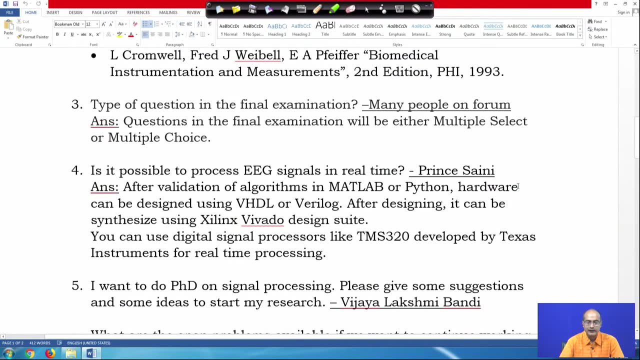 So that would be about the final exam. I am not taking the name of the that. the participant who has asked these questions, because I think there are a huge number of participant, asked the same question, 8.. Next question: 9. That 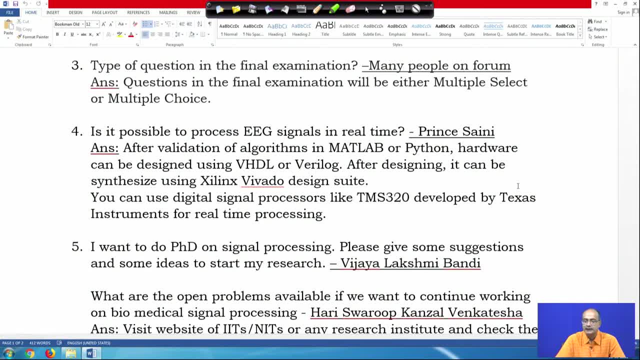 10. Is it possible to process EEG signal in real time? Yes, it is possible that there are number of techniques actually to do it. first of all, from week 9th when we are doing the, that tutorials in many place actually that I pointed out there. 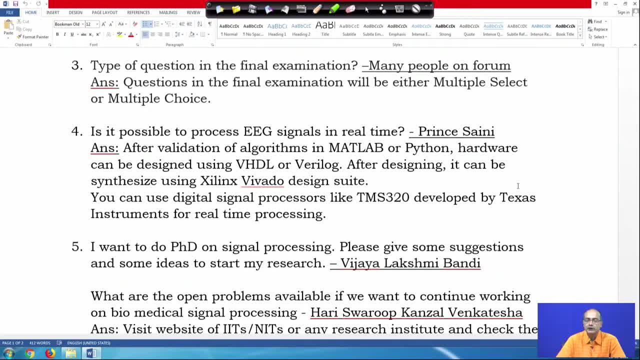 that. please look the. that filters what is used. they are integer filters. So you know that if you try to do some addition or multiplication that in your computer, that if it is integer it takes less time. If you want to have that, a silicon implementation of the same algorithm, it takes less space. 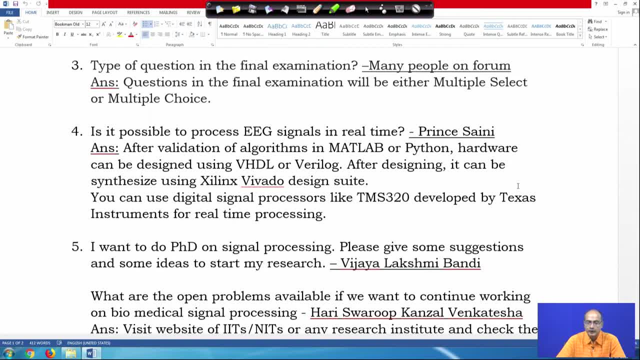 and less actually that the computation 10.. So if you can do the processing with integer number, that would be the best. The first step towards it is: first you implement it in MATLAB or Python. So check the functionality of it and you get an idea about that how much time it takes. 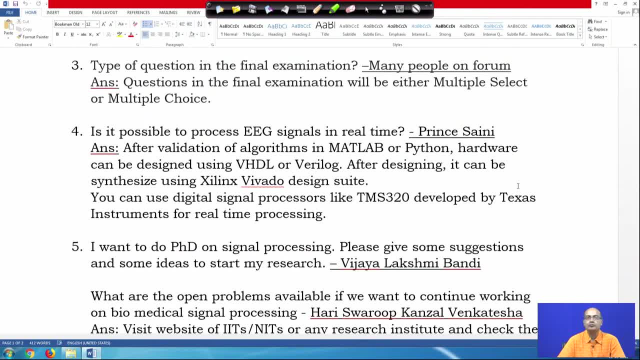 Next, you can choose an appropriate platform. it could be an embedded processor like ARM, or it could be 11.. That a actually that FPGA for which you need to do that VHDL programming. or it could be a DSP like TMS320- from text as instruments for real time processing. 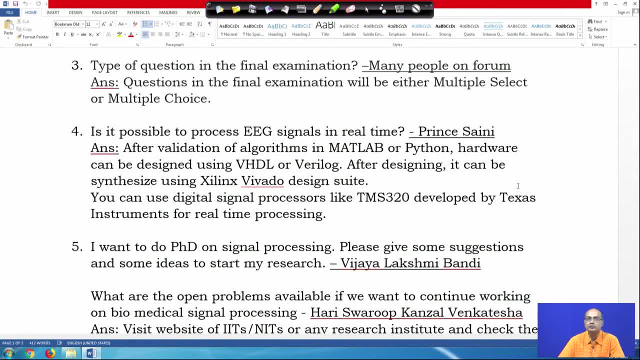 So, depending on that, how much computation you need. or, to be more precise, that when you are talking about real time, that means you have a constraint over the time, over process. That may be you can just wait for the next sample to arrive. So within that you need to compute the that whole process and be ready to take the next. 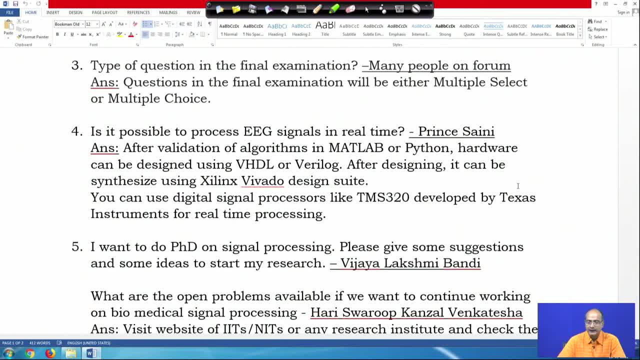 sample. So for that you have to choose appropriately that what platform you would take, and if I want to actually name one of the 12.. So if I want to name one of the real time application that nowadays those, the pacemakers- 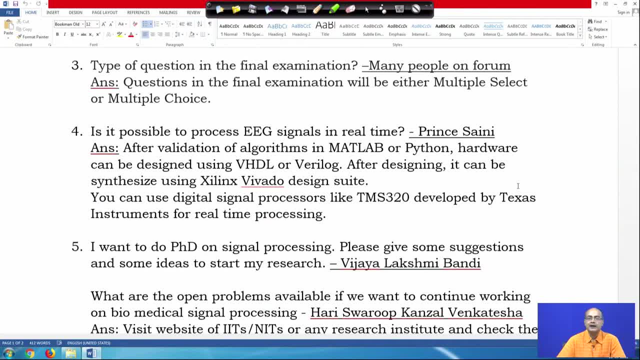 are there. they are actually supposed to give a bit because the hard bit, the signal, comes from the SA node. it may not be coming all the time, So pacemaker is supposed to provide that bit 13.. Now initial 14.. 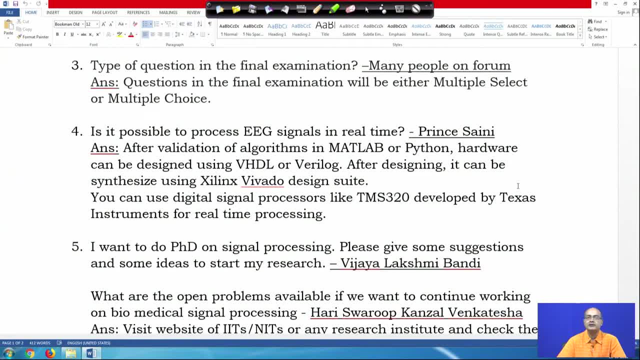 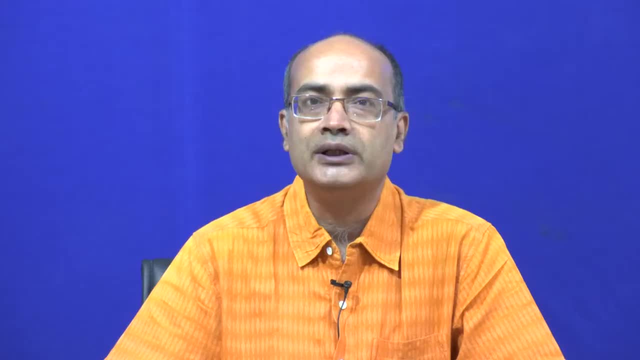 So the prototypes, or the initial days, the first generation, the pacemakers used to all the time provide that bit. So whether SA node is working or not, it is continuously working. Now the effect of it is that it would need actually a bulky that battery and still the 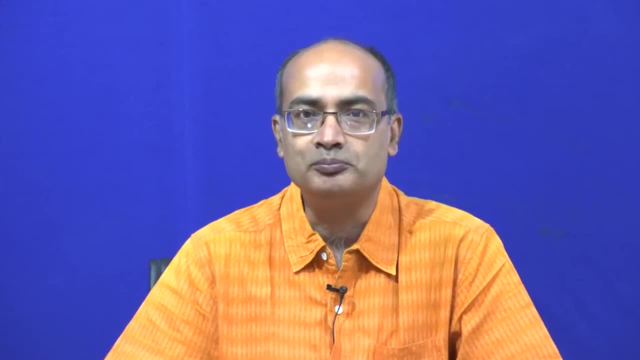 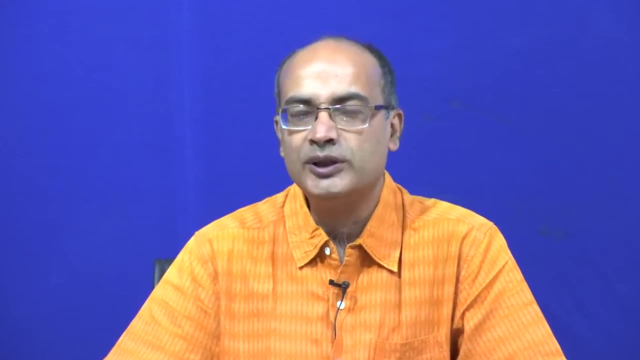 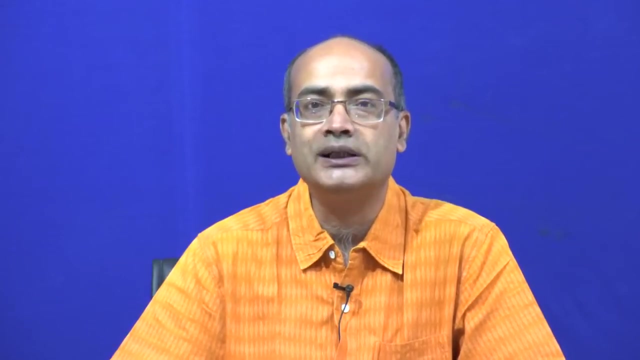 battery will get drained because it is working all the time 15.. In fact that the researchers- they found that SA node is not that bad here. some problem is there for a particular patient. So they are not working all the time, but most of the time they work. 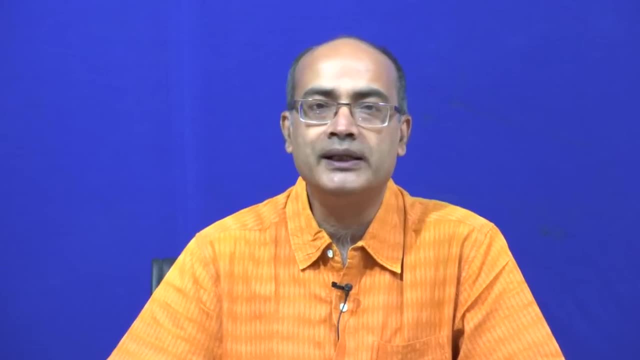 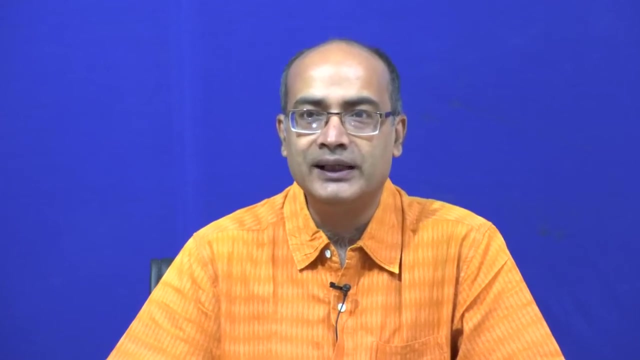 Sometime for some problem. they do not actually give the bit in time and the patient suffers for that 16. So they made the pacemaker 17. So intelligent. So it would be waiting for the SA node to act and if they find that SA node has missed. 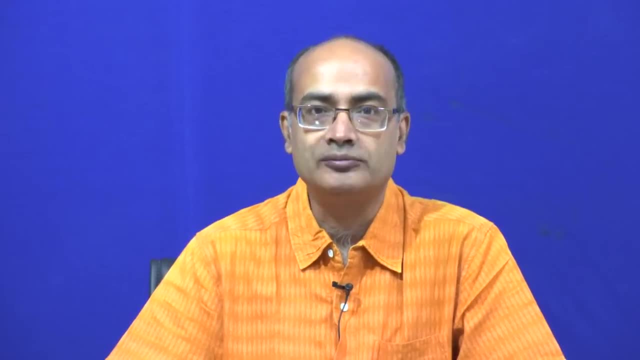 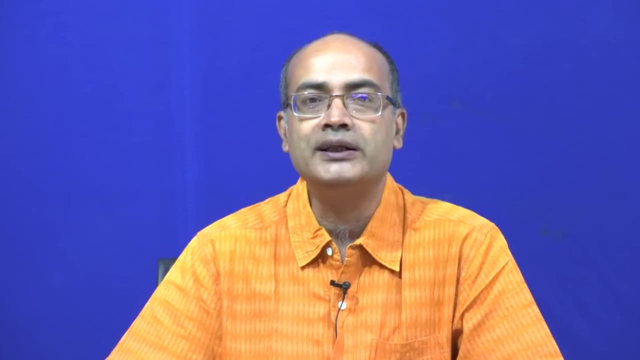 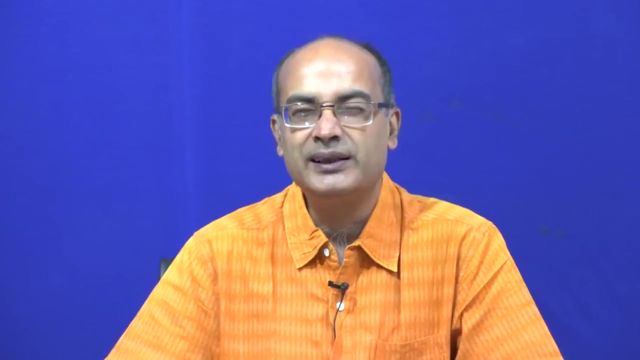 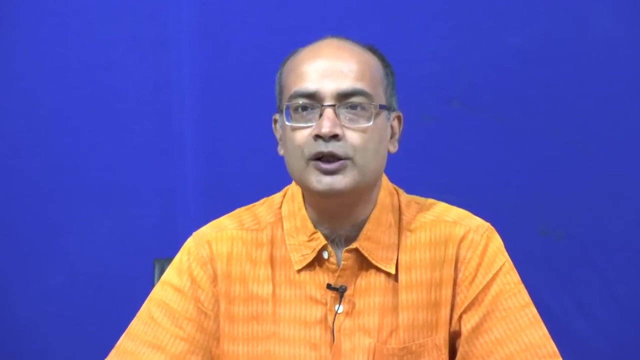 the bit, then it will take over and still it will again keep and watch whether the SA node have actually taken up its job again. If the SA node again started giving the bit, then there is a chance that you can have actually that ectopic bit, because two signals or two commands are coming. 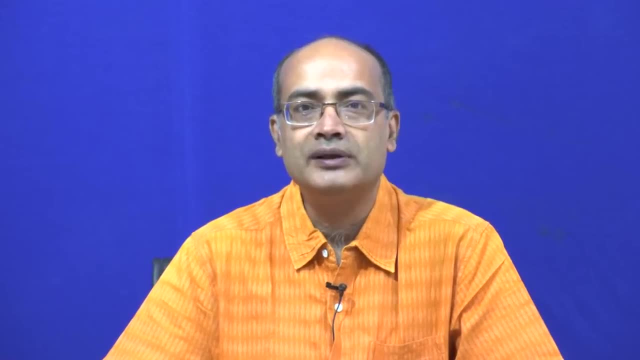 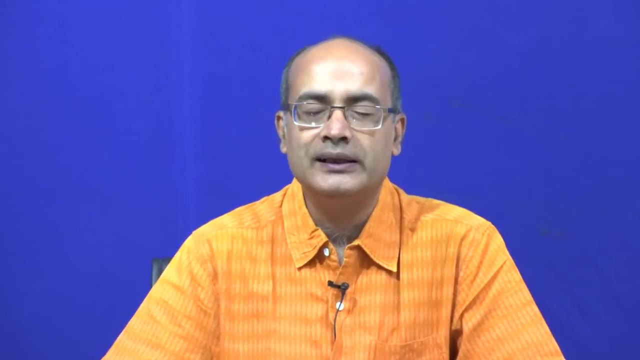 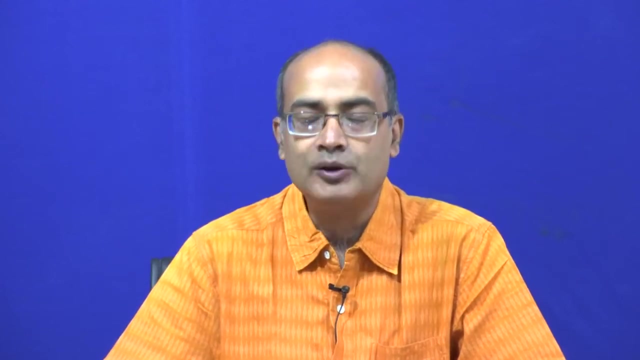 So the pacemaker again will take itself in sleep mode or listening mode and allow the SA node to work in the normal way. So that is completely in real time. it does the job. So there are lot of applications for which the biomedical signal processing you will. 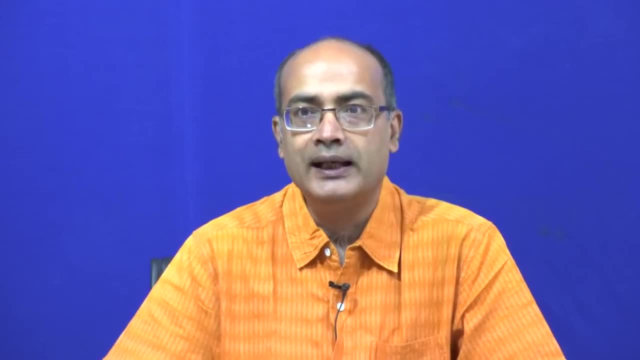 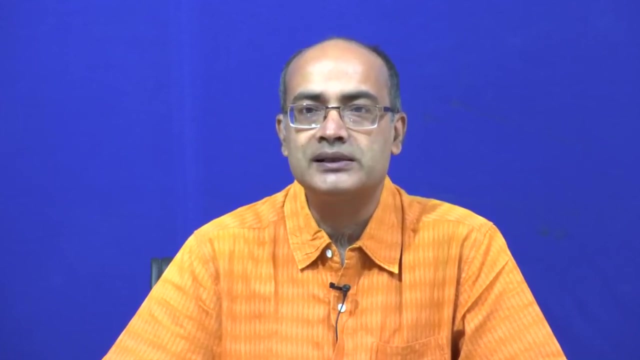 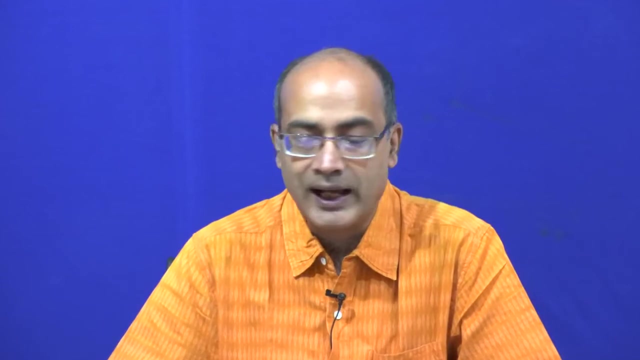 find that it works in real time: 18. And I would say that it is not a that big a challenge because that if you look at the signals, the frequency of the signal is much less compared to the that the communication signals. So it is highly possible to actually that process them in real time and it is done in. 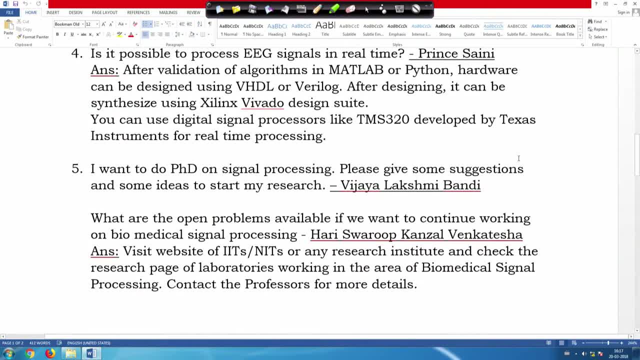 real application 19.. Next question: I get that that we have clubbed actually number of questions. one from Vijayalakshmi Bandi. that question is: I want to do PhD on signal processing. please give some suggestion and some idea to start my research. that next, that along with that in similar line, what? 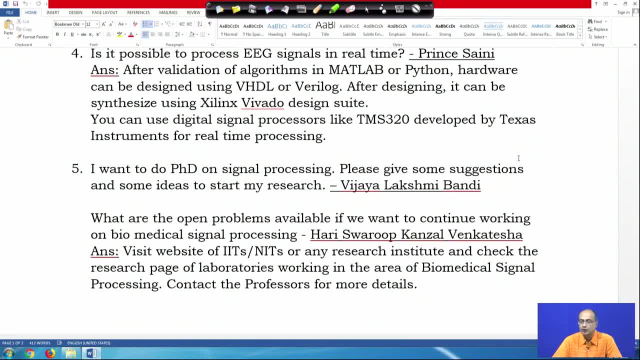 are the open problems available? 20. If we want to continue working on biomedical signal processing- this question has come from Harish Haroop and that I would say that such question should be taken one on one basis. that means you should ask the question on personal level to any faculty you can go through. 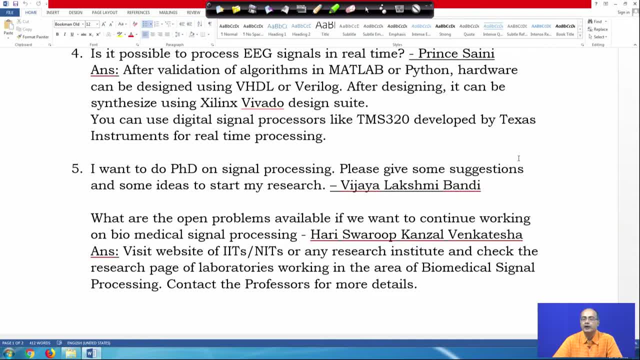 the web page of IITs or NITs. 21. And find out that whose interest are. 22. And find out that whose interest are actually matching with yours. there are number of actually good researchers in India who are working in biomedical signal processing at present. 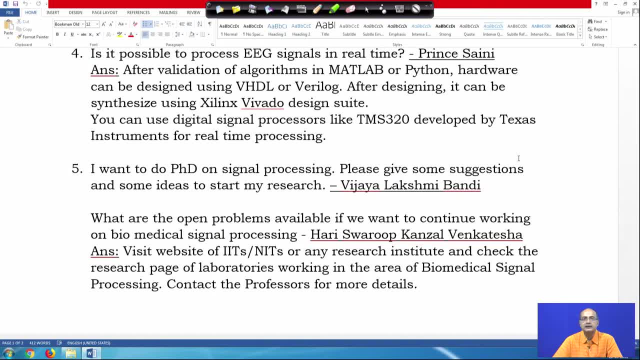 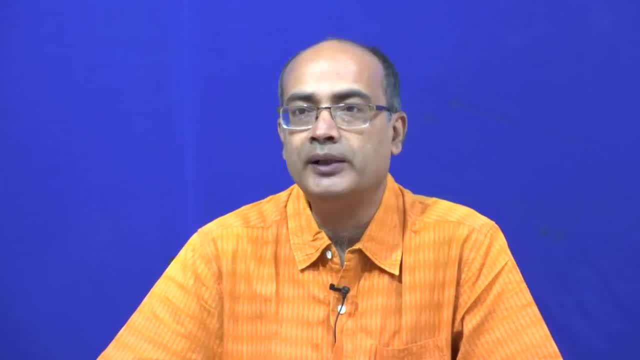 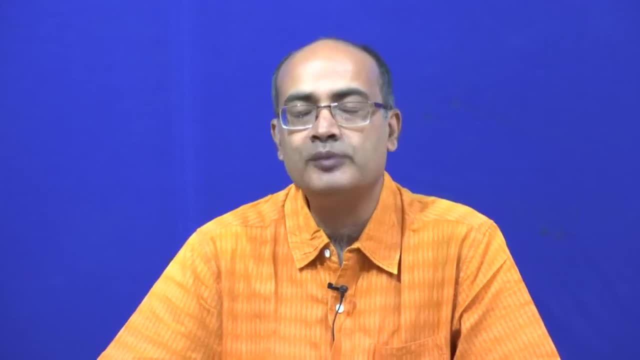 I look more towards that, that image processing, medical image processing, rather than the signal processing. anyway, you can contact in any one of them and it would be the best to get the suggestion from them. 23. And there are number of open problems. 24. 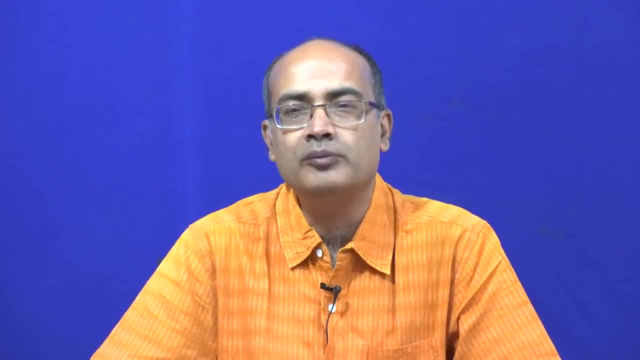 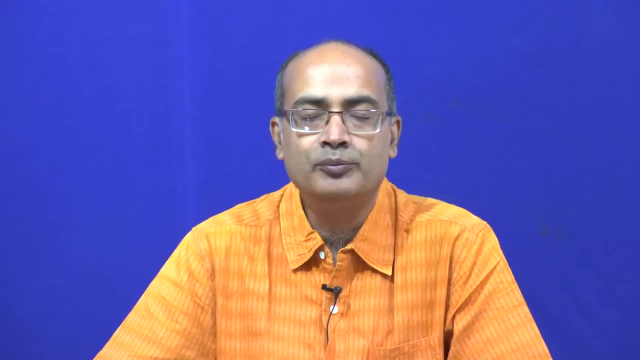 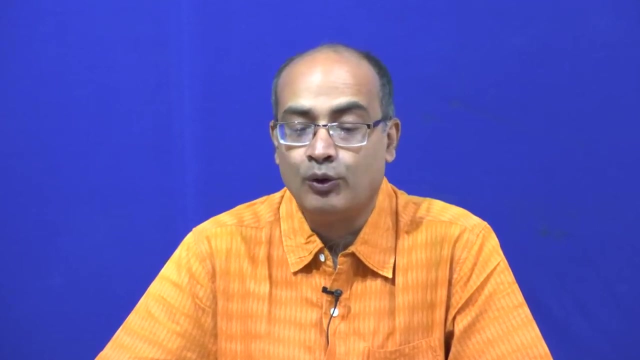 And they are working on them, and all of them could be very good use for the mankind and that it can help to the people of our country as well as throughout the world. and one more point: that all such applications, they are for the peaceful purpose which we sometimes 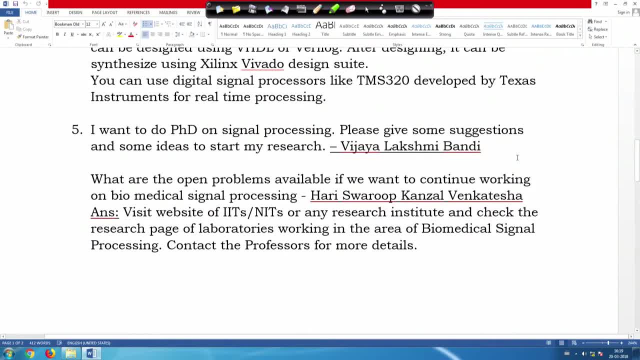 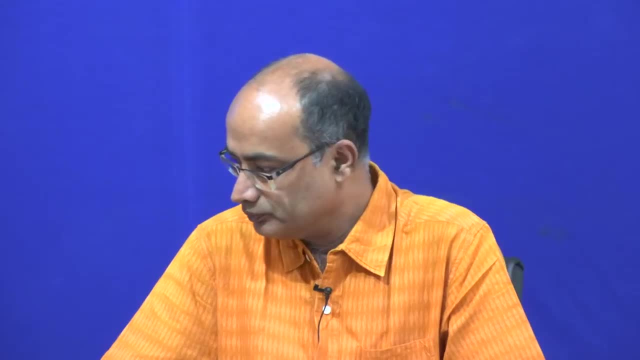 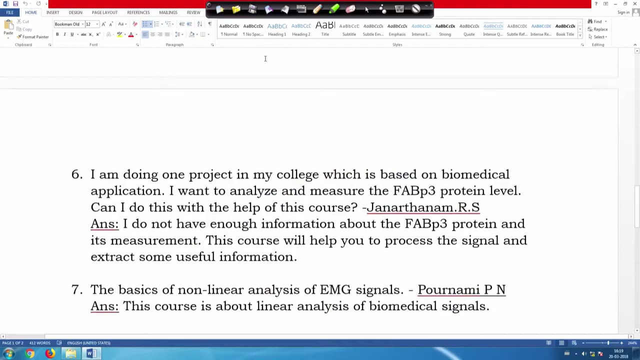 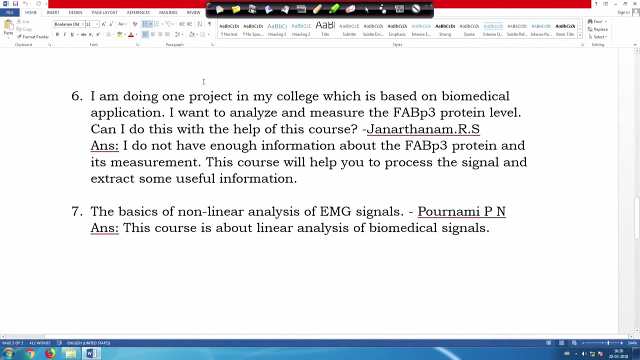 we miss for the other technology, ok, 25.. So you are most welcome to do the research, but I think such question should be asked in person to one expert with whom you would like to work. so ok, we have some more questions already given in the Google sheet. 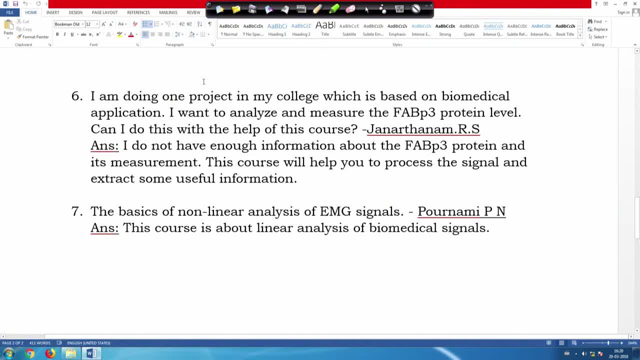 26. From 27. J R S. I am doing one project in my college. what is based on biomedical application? I want to analyze and measure FAB p3 protein level. can I do this with the help of this course? I am very sorry, I do not know enough about that FAB p3 protein now, if you share some. 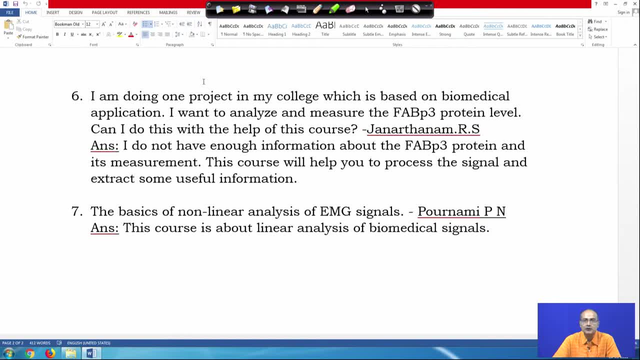 information that how it works or so Then we can try. So this course is primarily for that: biomedical signals and how that signal can reveal the internal physiological process going in the body and thereby you can get that whether those physiological process they are going in a normal way, as they are expected to go. 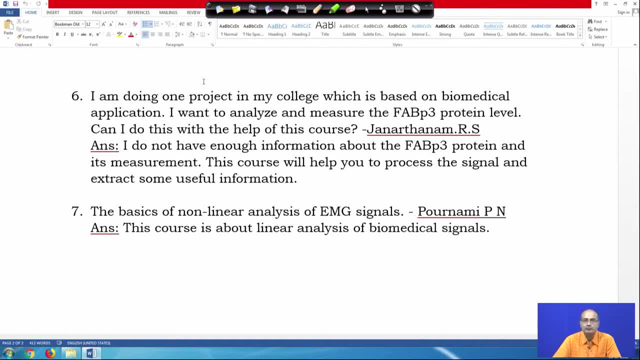 or they are facing some problem 28.. So sorry, I could not help you at this moment. next question is the basics of non-linear analysis of EMG signal. this question has come from Purnima P N in this course. primarily we are looking for the that linear actually processes, linear signal processing. I would 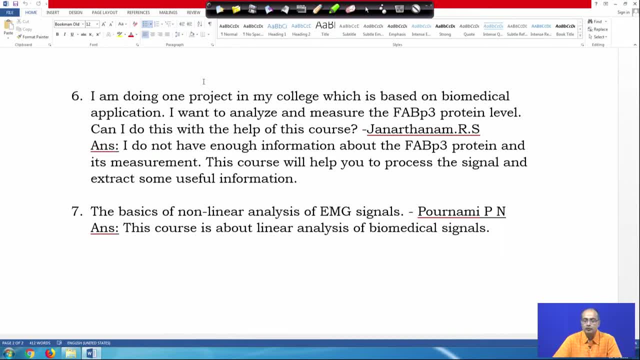 say: And we have not gone for the non-linear models. however, if you have any non-linear model in mind, yes, they can be tried. we will have used them for different kind of biomedical signal, because linear signals always cannot actually express the complexity of that signal. the 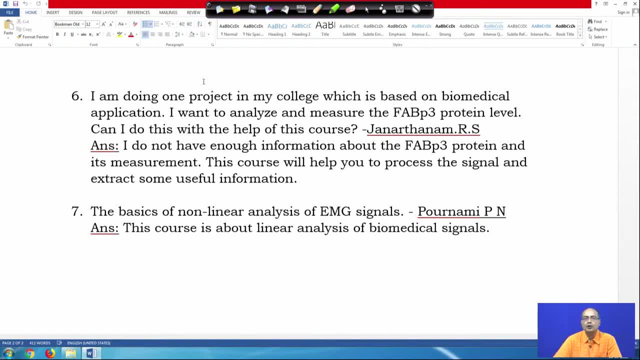 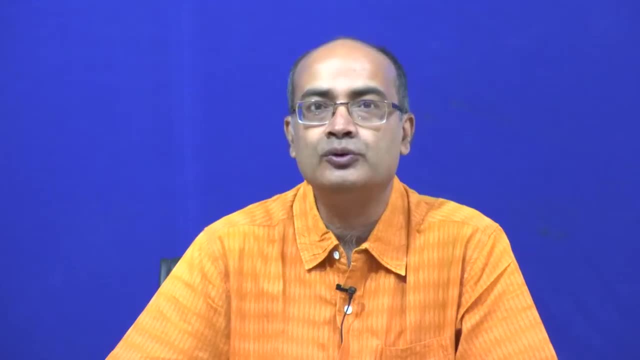 other way you can look at it, that all these signals- 29. Are basically non-stationary in nature. so another alternative to the non-linear system is that linear time invariant systems. that is also another alternative you may explore. however, in this course we cannot go up to that, so we restrict ourselves for within the 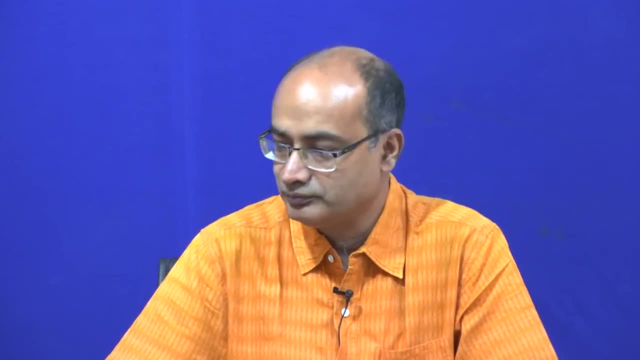 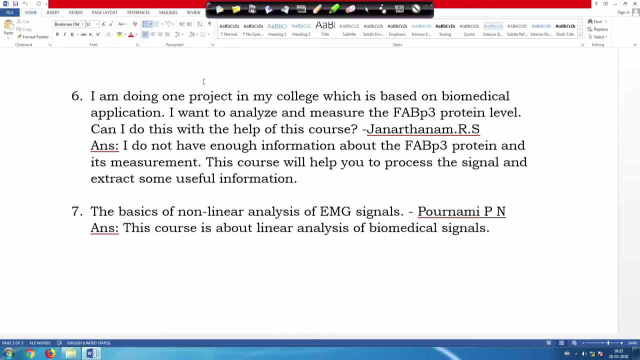 boundary of linear signal processing- 30. Now let us. we got just one more recent question for by Sivamshu Tyagi. the question is: what makes biomedical signal analysis more difficult or challenging than other physical signal analysis, 31. So it is a very good question that, if you look at that linear signal processing, 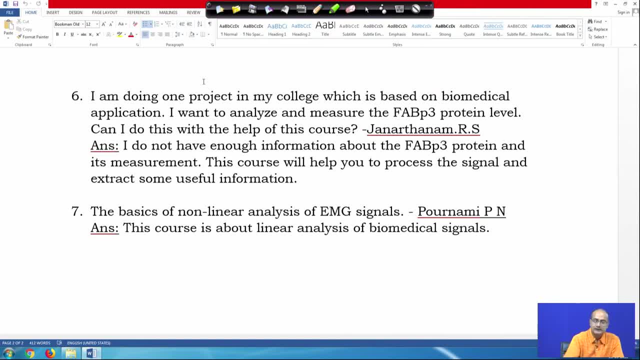 32., Yes, 33.. So in the signal processing that the two sources you can get, one is the real signal. it could be human speech, it could be some biomedical signal like ECG, EG or some other signal. other broad actually category of signals are communication signals now in communication. 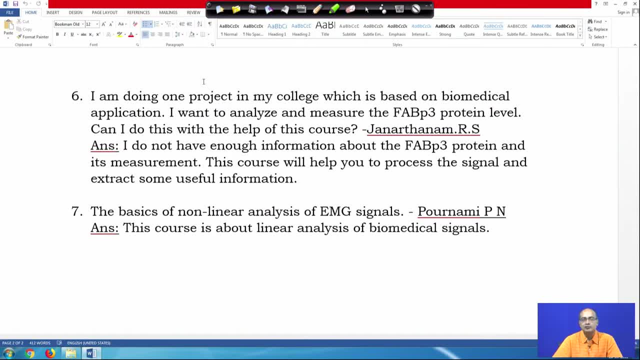 signals 34.. So in this case I would say the signals are much more well behaved because you know the source of that signal, that is, man made. however, it becomes complicated when it is passed through the channel because the deformities that comes in the channel or the channel transfer function. 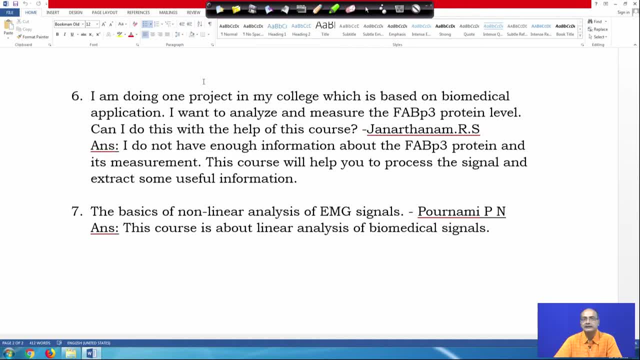 you need to really find it out, 35., 34.. However, it could be non-linear at times and there are many challenging applications like. one simple application you can look at is the ADSL modem, that is, we call the broadband access technology- those who still have that- the wired telephones. we know that we can get. 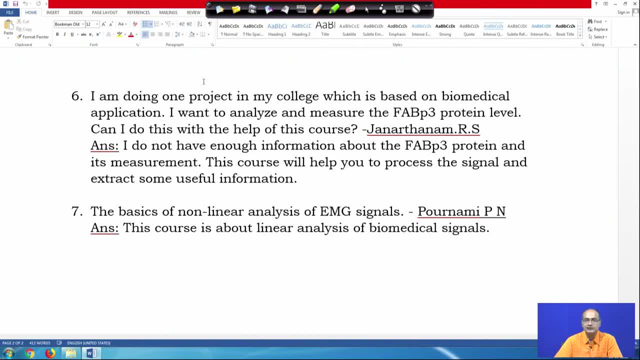 a high data rate within that And the principle of it is very interesting that only up to 8 kilohertz- that is the bandwidth that we are using for the voice actually speech, within that that we have the signal. beyond that there is a huge bandwidth for that cable but that bandwidth is not utilized primarily. 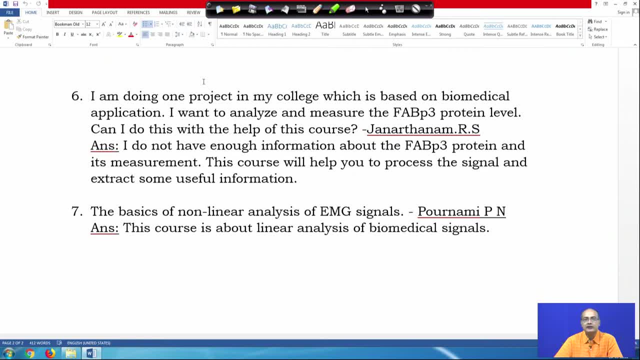 for the radio. So that is the reason that that part is very unreliable, in the sense that from one actually cable to the other, that in between, that means the from your actually instrument to the, that the exchange in between the pathway, that the channels are there, that is the cable connections. 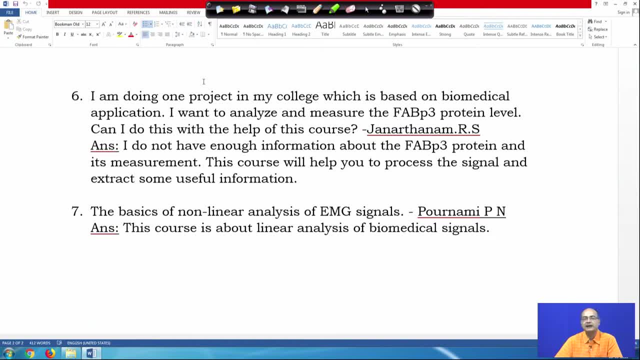 they are not same And because of that they are attached. They are attenuation characteristics in different frequencies are different, So you cannot standardize them. In case of ADSL modem, what they do? they break that into multiple, actually channels and check all of them and find out that which are reliable or strong in terms of the SNR, and they pump. 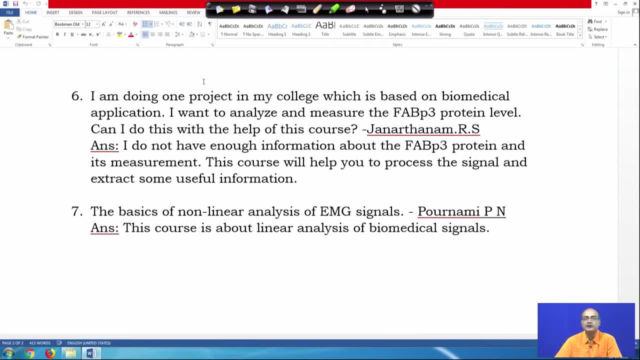 the data within that and they dynamically actually look at that, because this characteristics also changes with time. But still you know that there is a pattern that how the modulation would be done. those things are known. But in case of the biomedical signal processing, the main challenge is that the source is actually 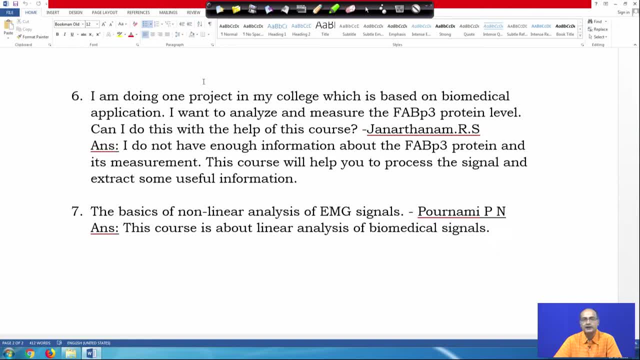 that the human physiology or the human body and each one of us is little different from the other. So signals are changing, though the overall pattern may look different. So the signal is changing. So the signal is changing. So the signal is changing. 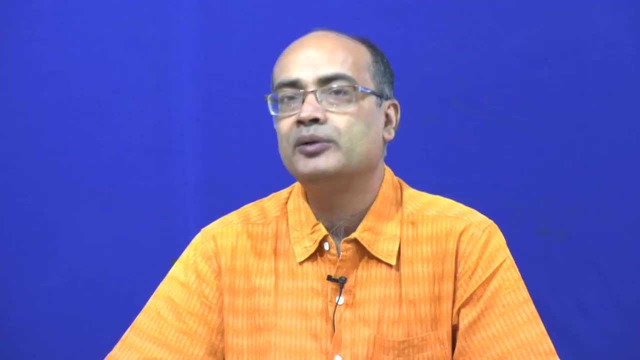 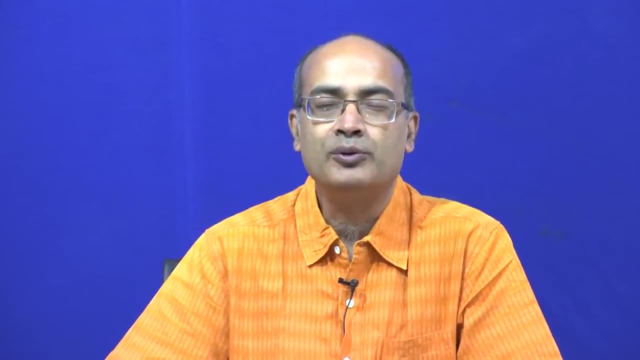 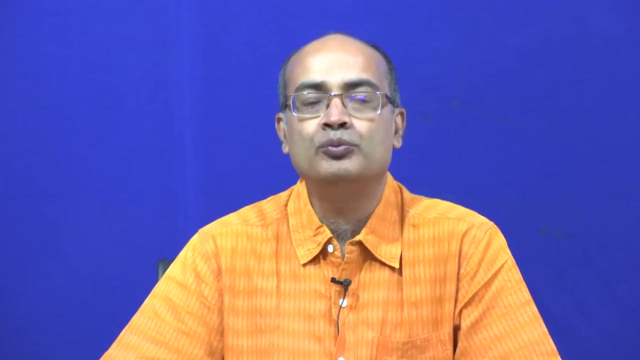 Because they are being tested to be similar, So treating them becomes more difficult and the variation is more. in that case- and what I would say? that there is continuous variation- You will get a spectrum of people whom we can tell that they are actually normal. 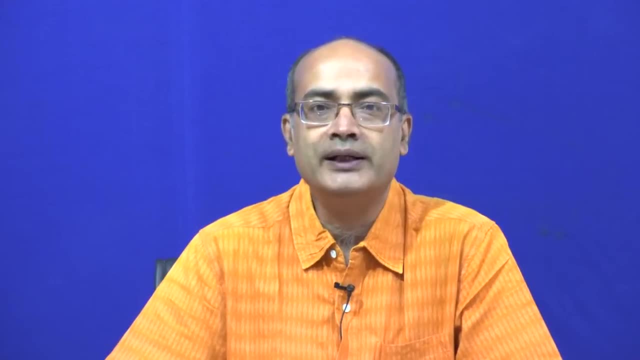 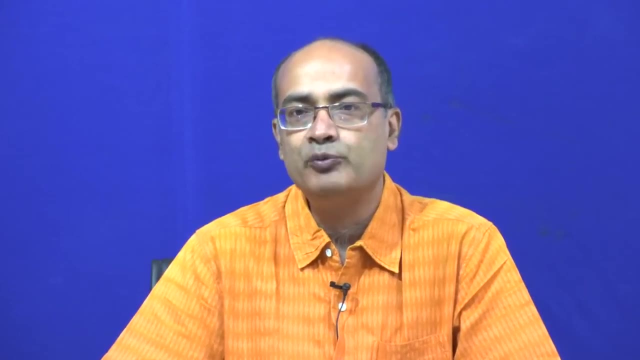 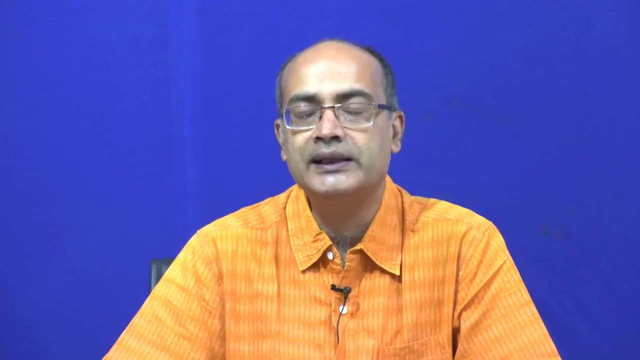 If you go to the doctor they will tell: yes, you may find it actually different from other people, but it is within the normal range And same way that those who are. we call that having abnormality or pathogenic signature. there also a lot of variations are there. 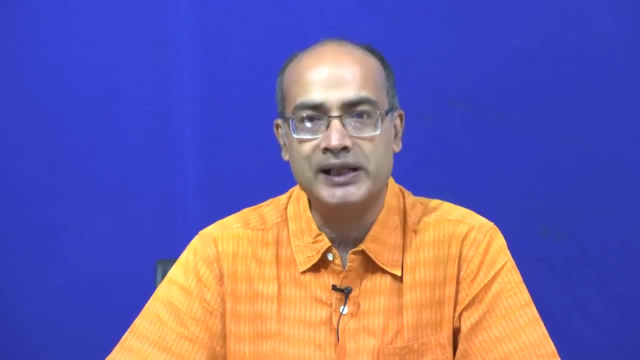 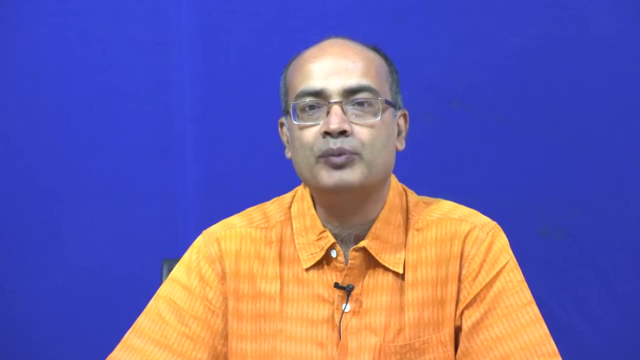 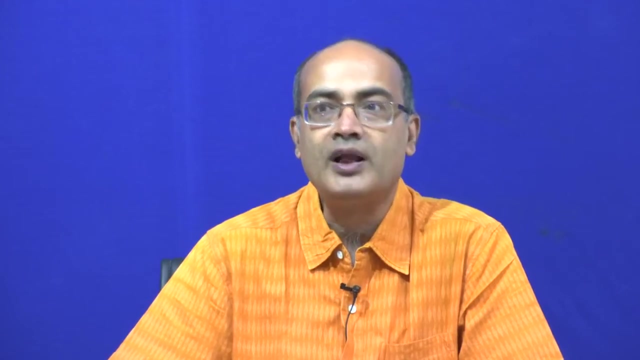 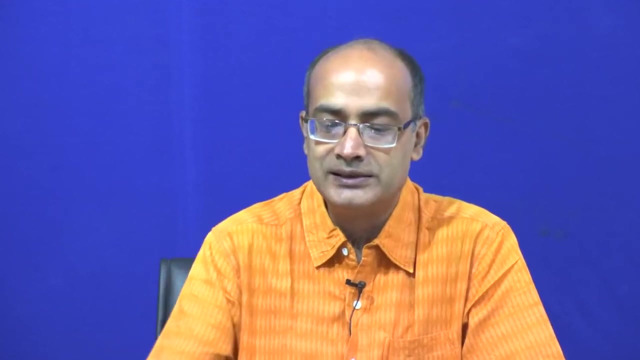 So that makes actually biomedical signal processing more challenging. but the good part of it, that biomedical signal, the frequencies are much low, So that makes the thing easier in terms of the real time implementation. However, for the analysis of the signal it is not actually that easy and it is actually 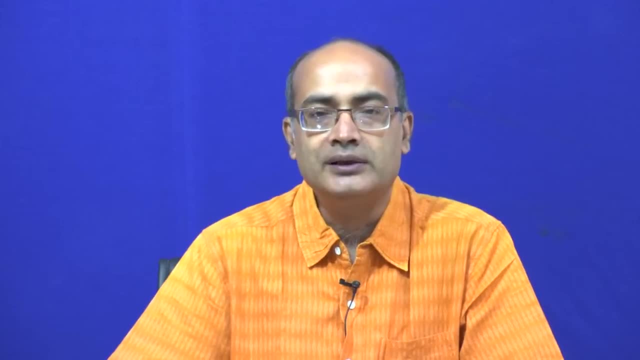 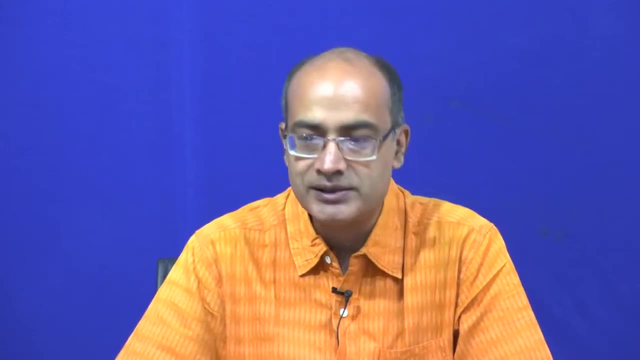 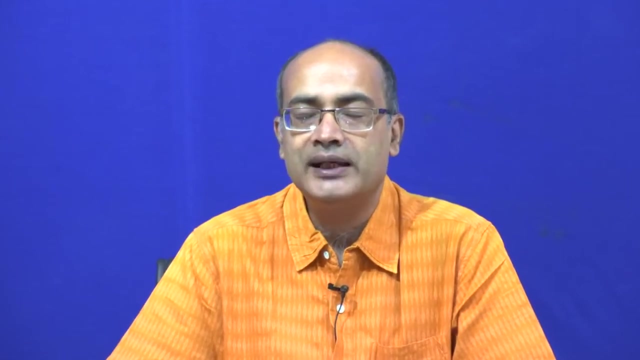 more difficult than the our. that communication signals. So these are the questions we have at this moment. If you have any other questions, you can just actually text it in the chat box and we would be ready to pick up those questions. Thank you very much. 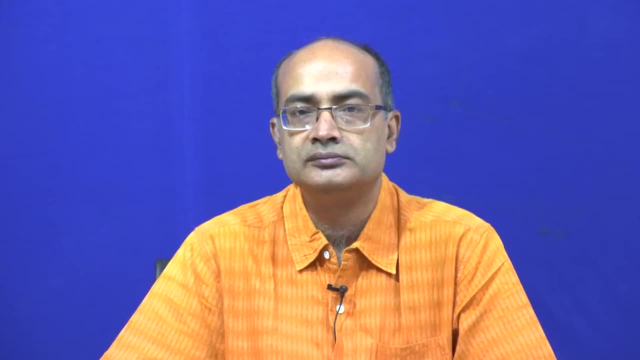 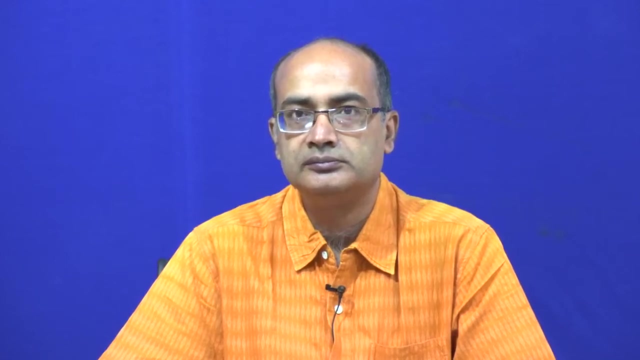 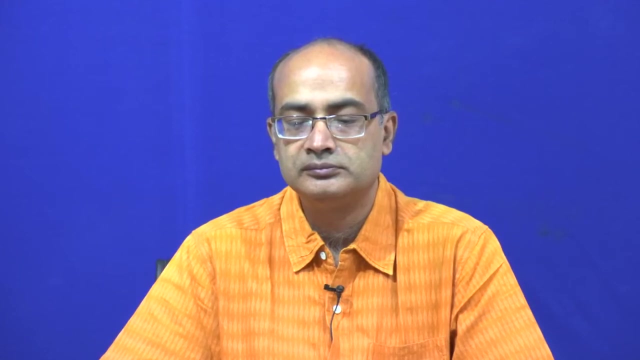 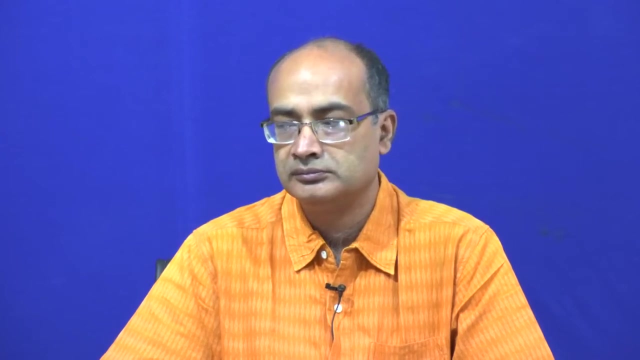 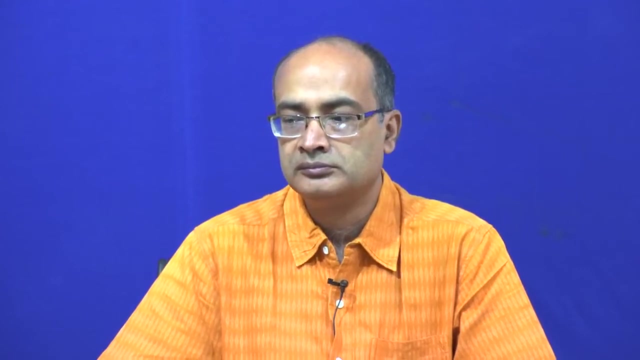 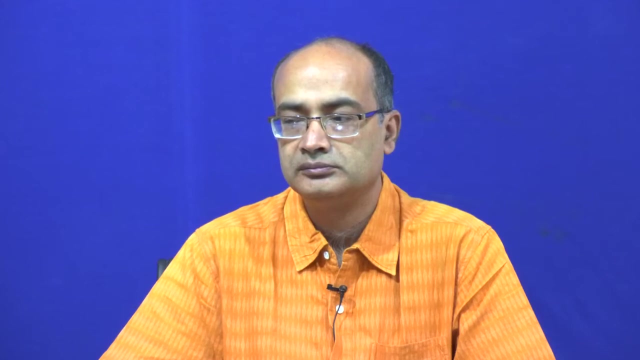 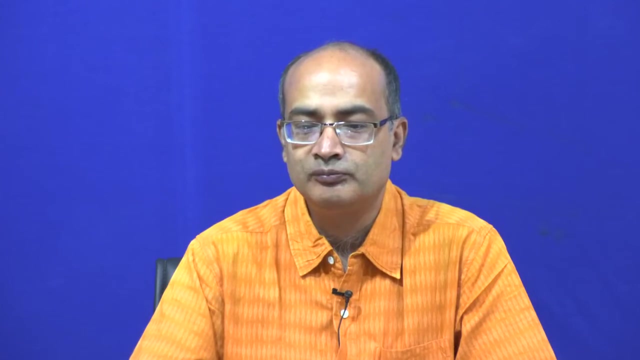 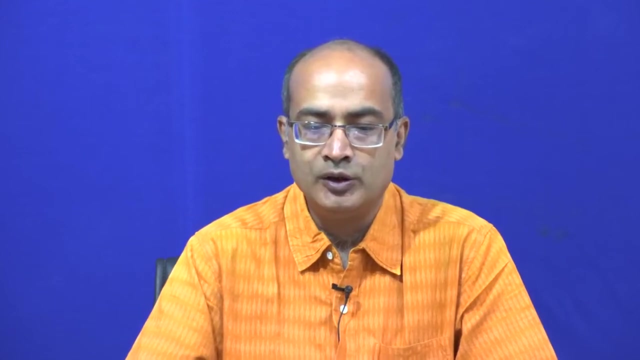 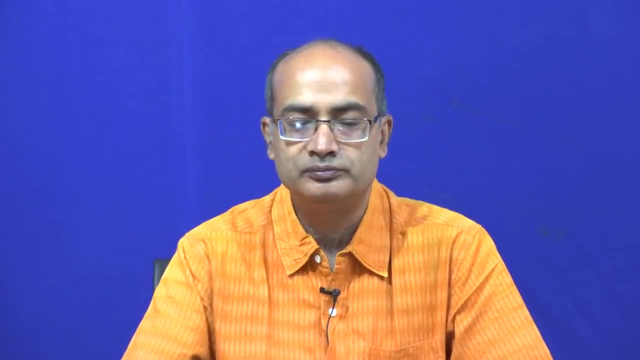 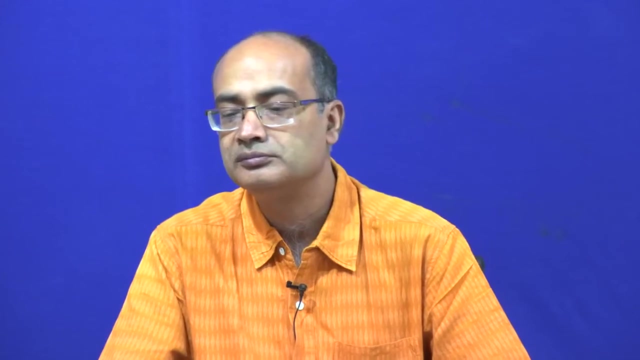 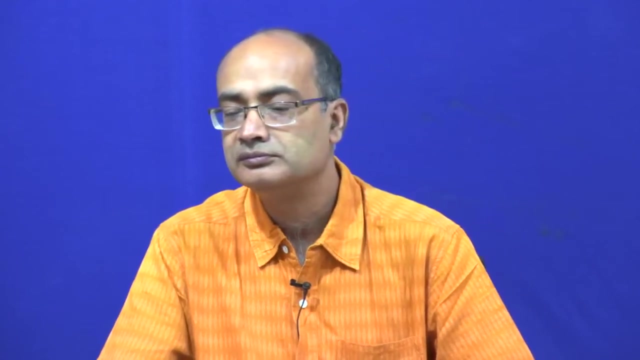 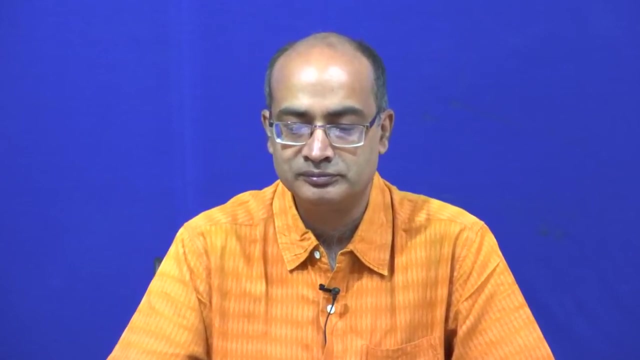 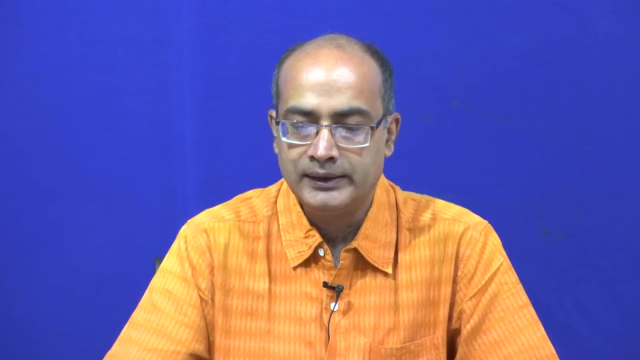 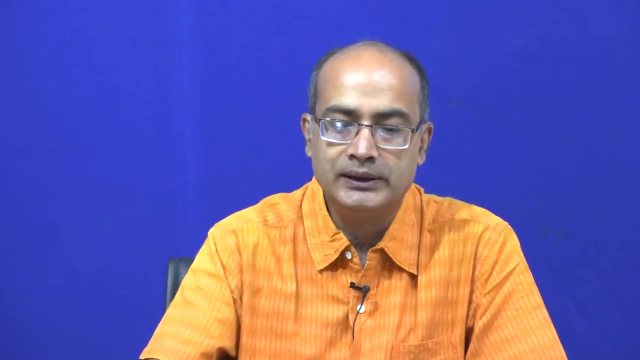 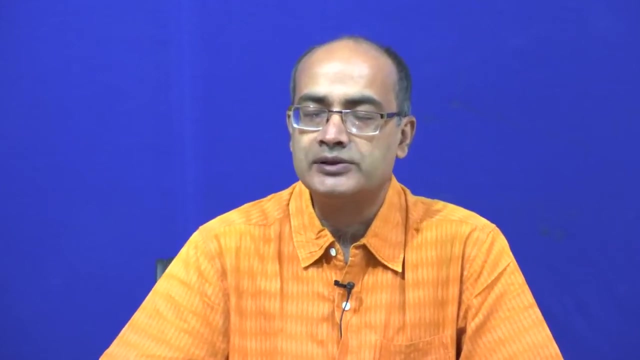 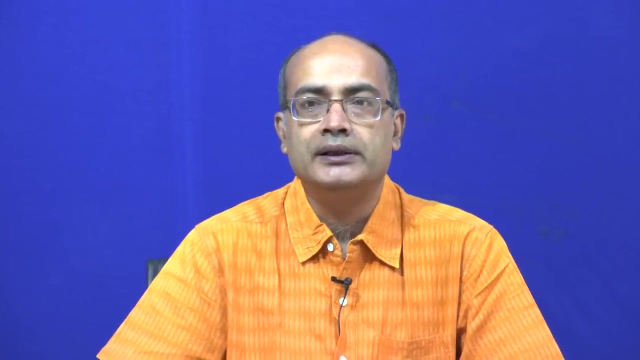 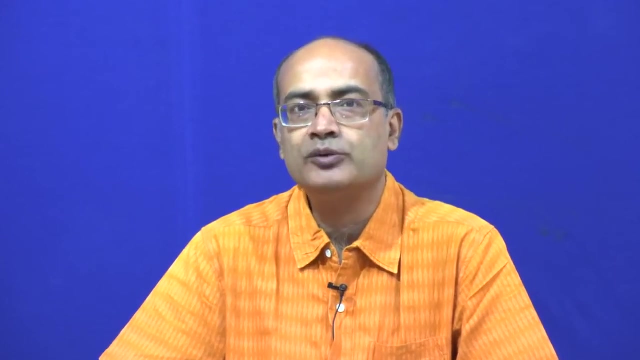 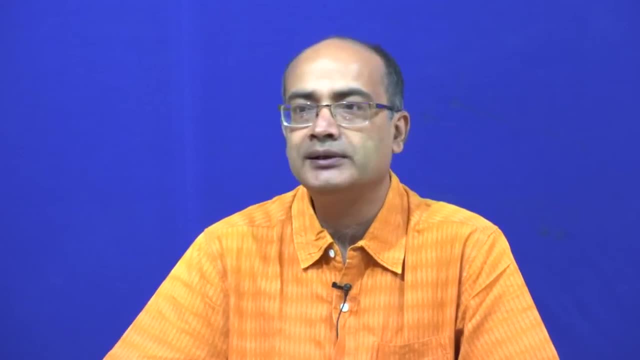 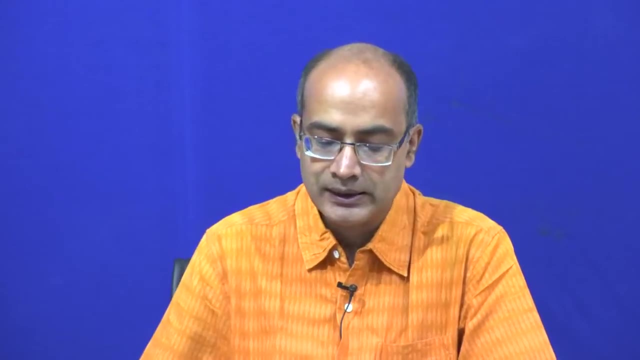 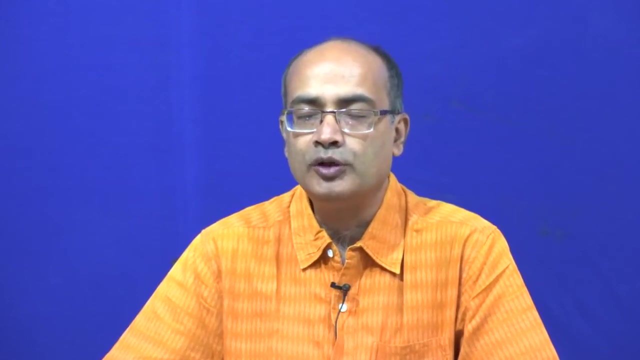 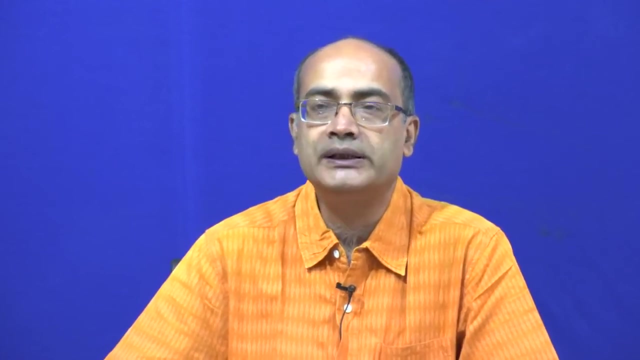 and primarily, they are introduced so that you can appreciate the that takes in a better way Those questions, that that the those questions actually, we would not be able to ask you in the exam, simply because that the MATLAB support will not be there, ah, at the time of the exam. ok, you will. 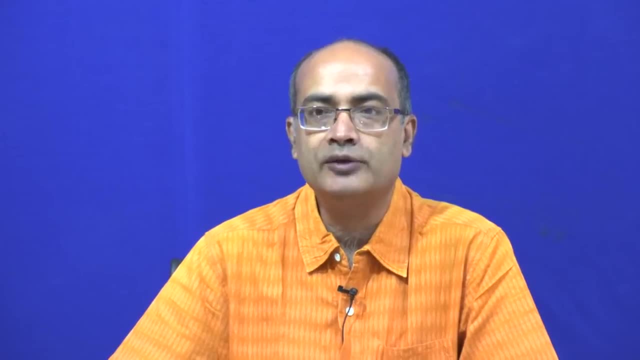 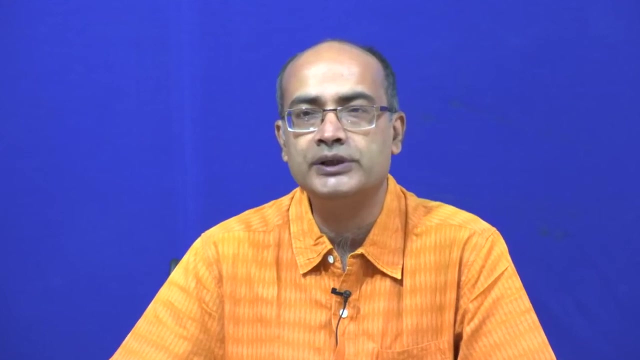 not have access to the MATLAB, So those kind of questions would not be there. However, the keeping that in mind, if there is any small computer So computation, you would keep them small so that you can do those computation using calculator. if you know the, the equations, ok, ah, 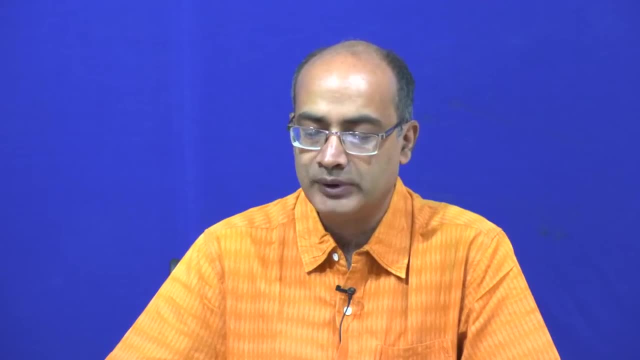 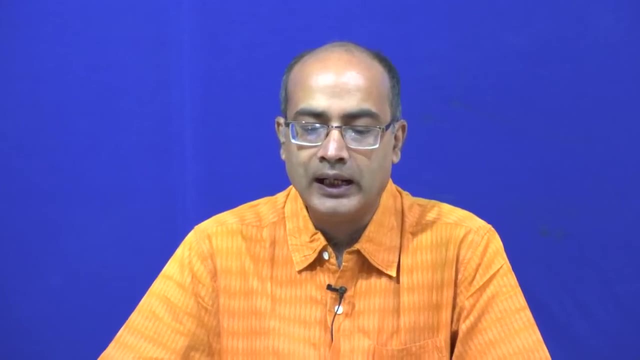 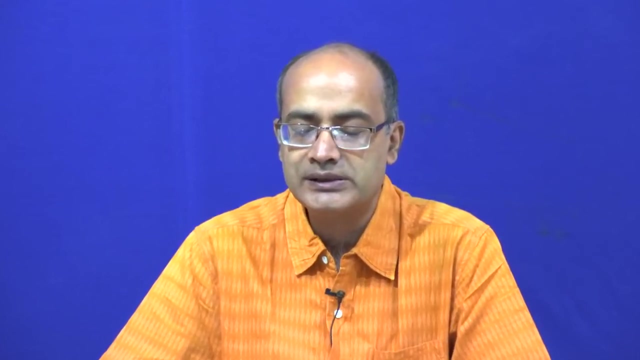 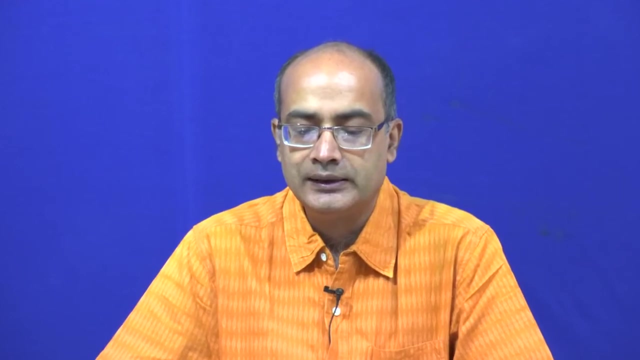 We got one more questions, so let us take that before we come back again to the the exam. How to understand mathematical equation for biomedical signals. These questions for came from Pankaj Kesari. it is a very good question, Pankaj, that when 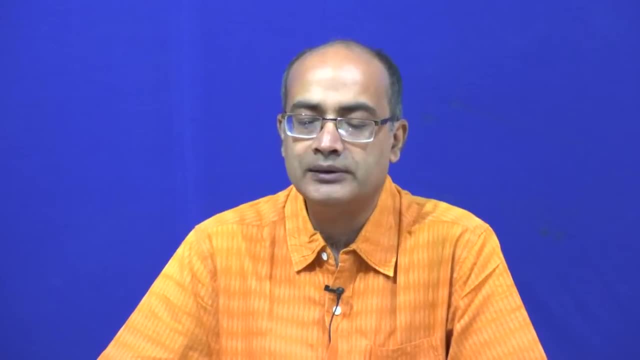 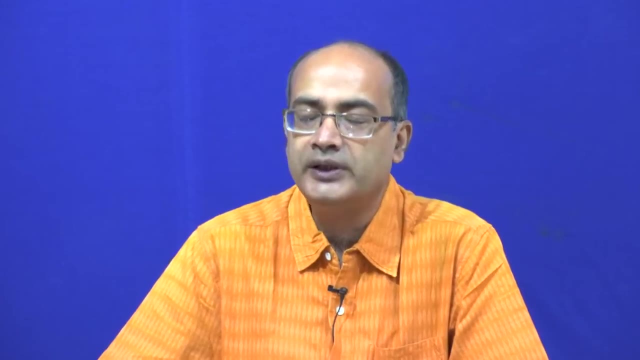 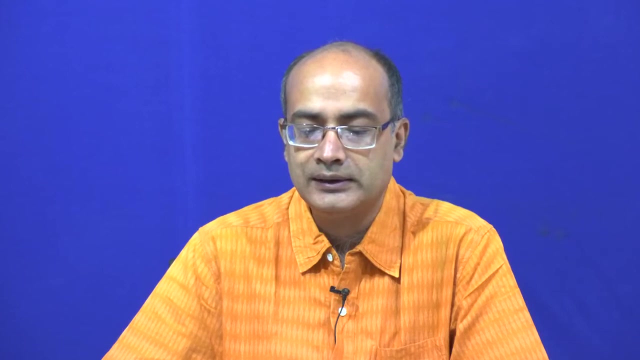 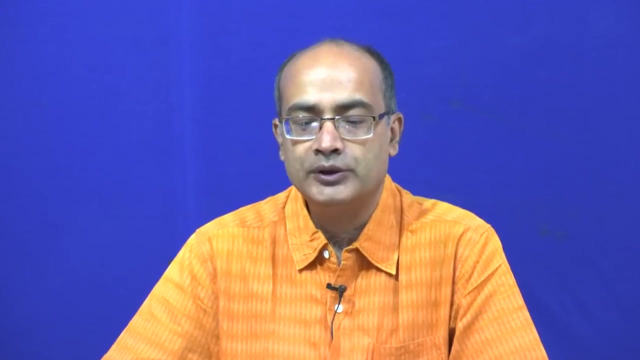 we actually teach actually biomedical signal processing. we try to go step by step to explain you that, what are the assumptions taken for that And that the way you have to be able to understand some of this. Please repeat, Ok, to do that you need to take actually those equations and try to derive it yourself And 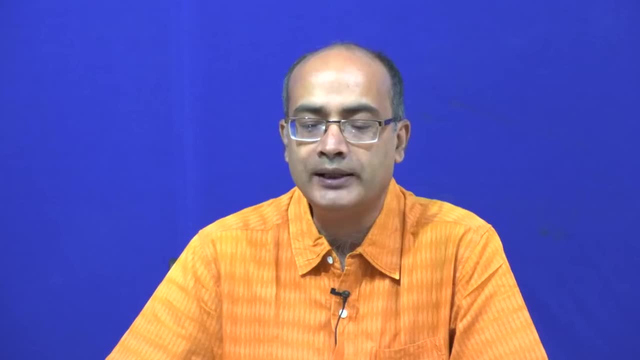 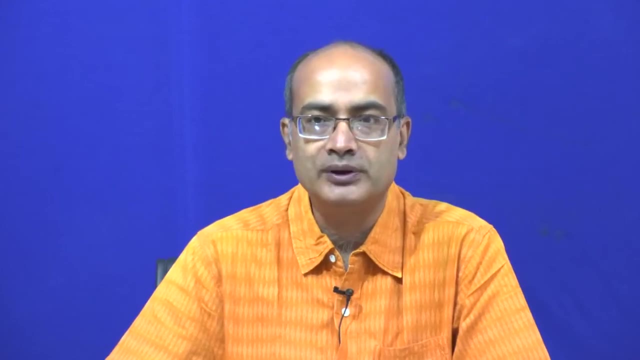 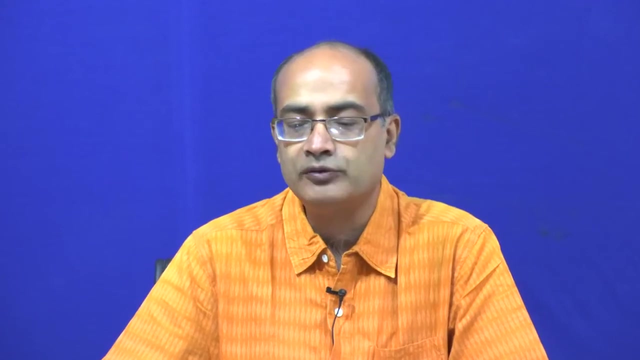 whenever you will fail. then if you cannot do that, you should look back to the book or the notes to see that how the derivation is performed. There are number of tricks that is applied. sometimes there are different formulas that is used. usually we provide them and sometimes it is from our, the basic: the knowledge of signal processing. 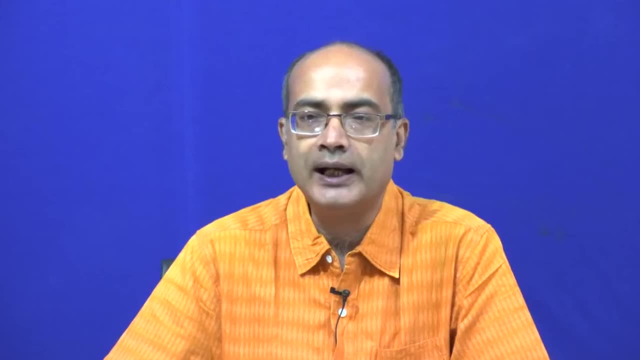 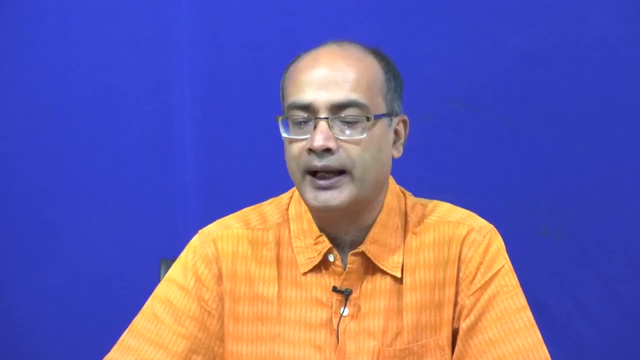 So here what we assume actually, that you have the knowledge of signals and systems. there is a must that you should have that to take this course, and if you have that background, I think that it is not difficult to go through them. The only thing you need to understand. 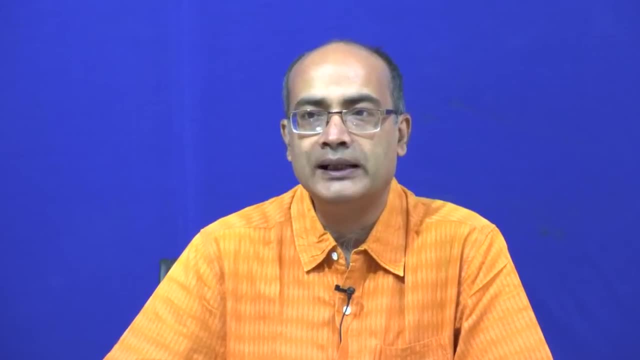 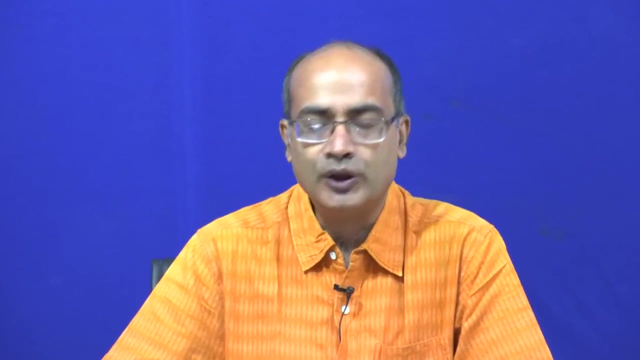 and understand is that you should patiently go through them line by line and you should try to derive them that line by line, And there is no point trying to memorize them or mark up that. that is not required. you should appreciate that. what are the tricks played? 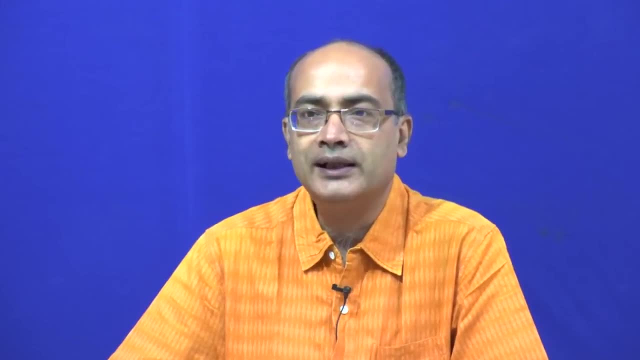 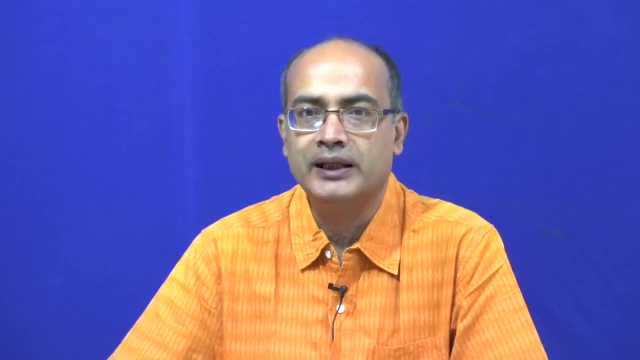 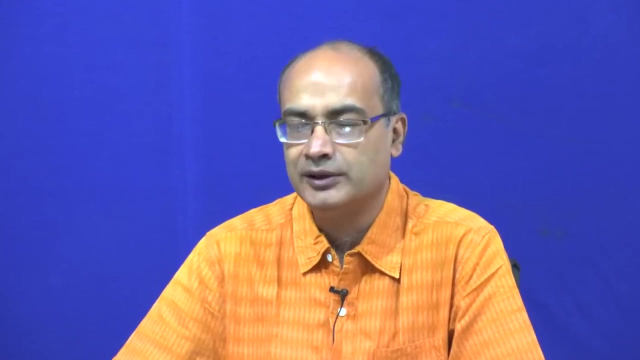 at different step to get the the desired answer. So how the manipulations are performed, how done at every step, and the best way to do that, that you do those calculations line by line yourself. If you find it difficult, look at the book or the note. see that how they. 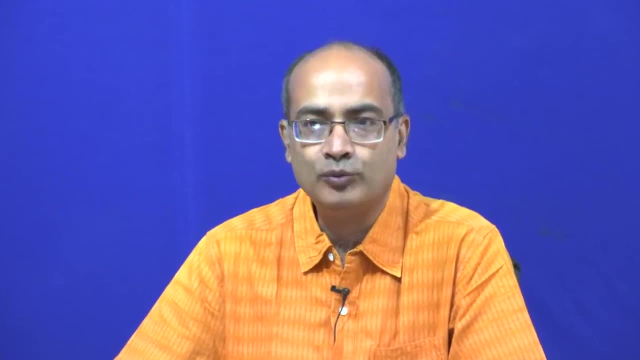 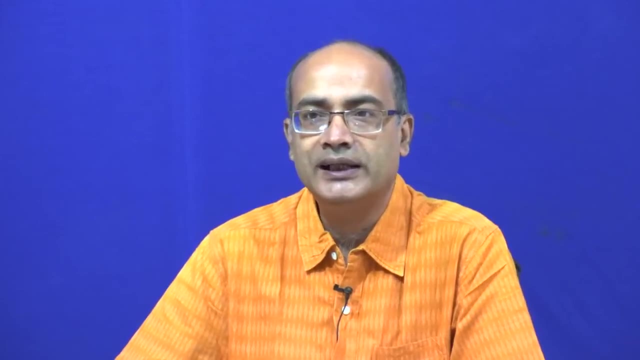 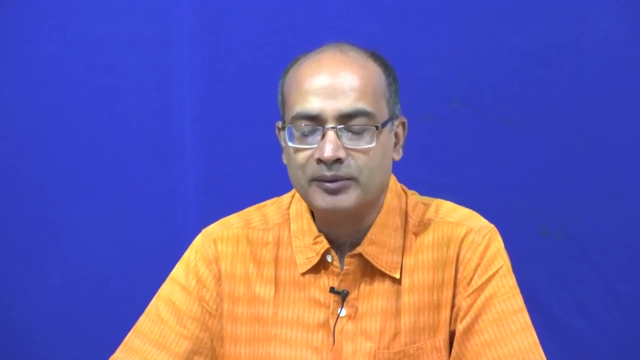 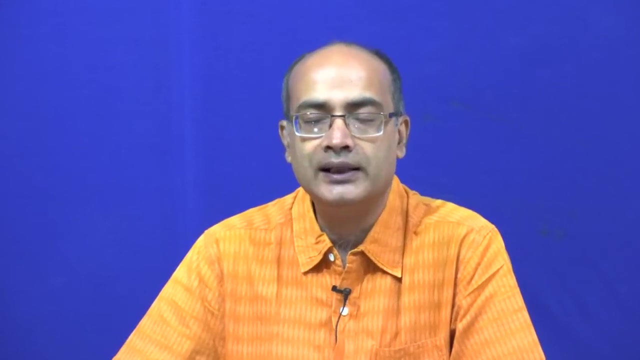 have done it, try to get that. what is the formula? they have used that to actually make that change or manipulation, and then how it proceeds. So that is the way to actually understand the mathematical equation for biomedical signals and if you have some specific question regarding, 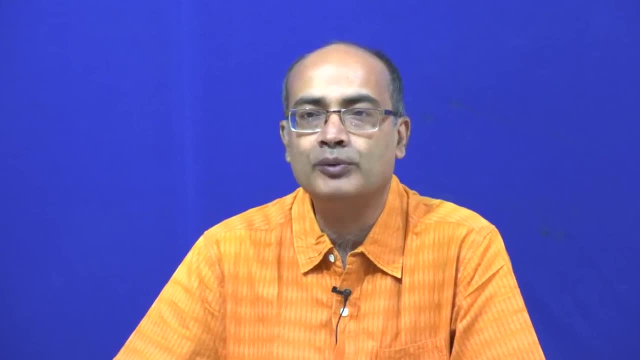 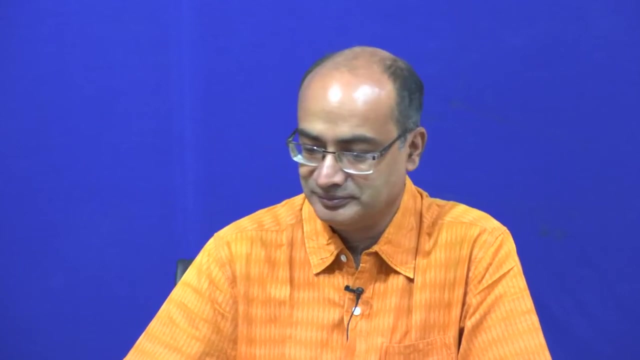 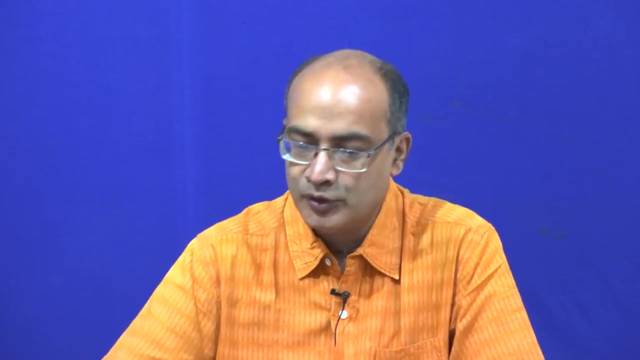 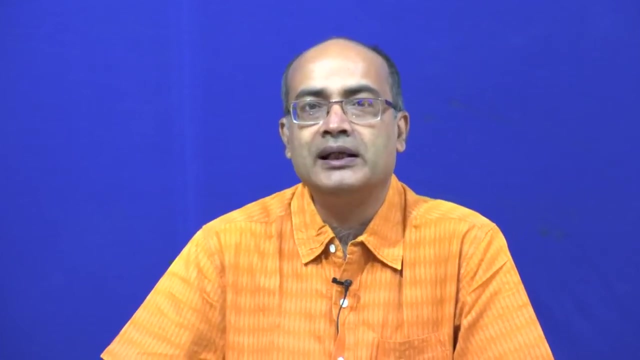 some derivation, that is, are how you have gone from line 1 to line 2.. So in that way you can make such pointed queries in the forum. we would certainly try to reply to you. So, going back to the that, the exam that we need to look at that, the whole syllabus, that 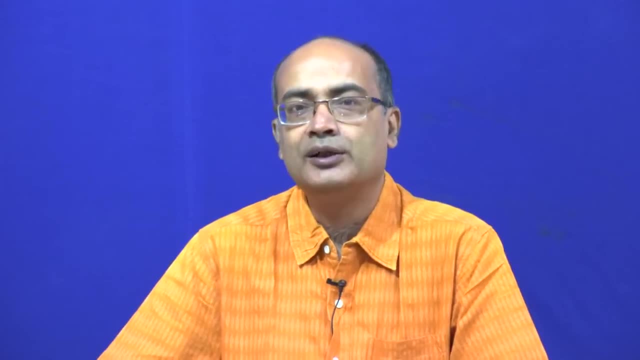 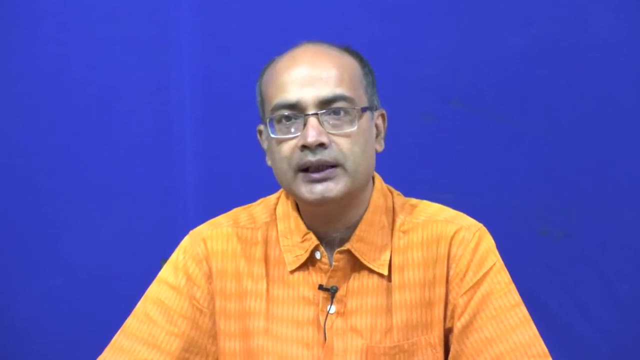 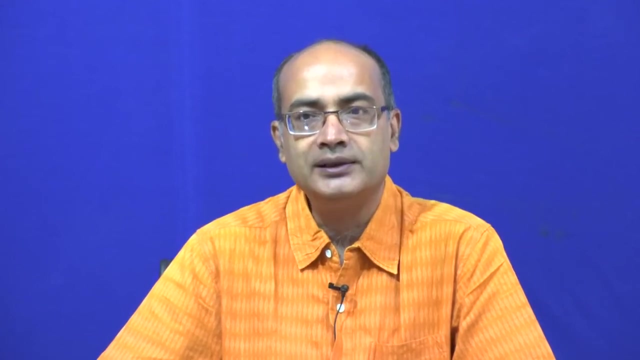 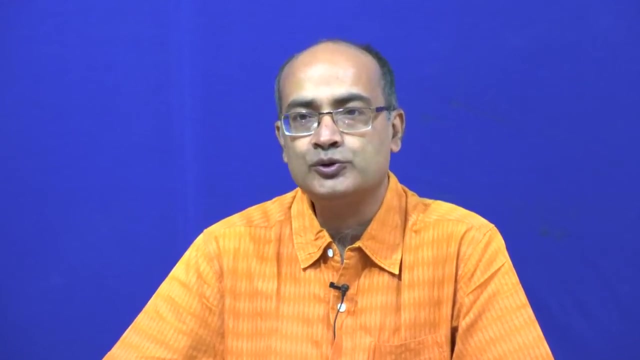 is one of the criteria to be prepared for this exam. In the first exam, In the first exam, In the first exam, 8 weeks, we have actually covered the whole syllabus and after that we are taking the tutorial So that you can appreciate those actually theory in a better way, and that also. 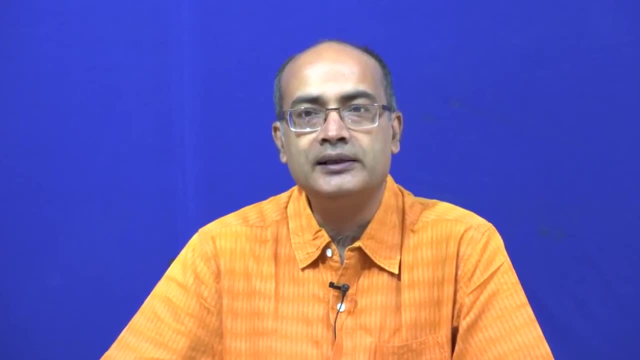 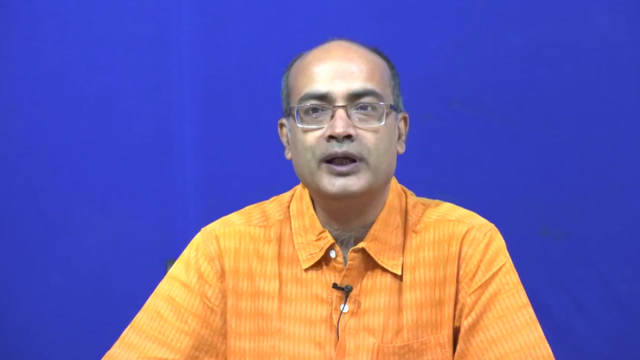 helps you to get acquainted to the real signals. Otherwise, after taking that course, if you do not know how the carotid pulse signal looks like or how the ECG signal looks like, then I think that we have not been really successful in teaching you. 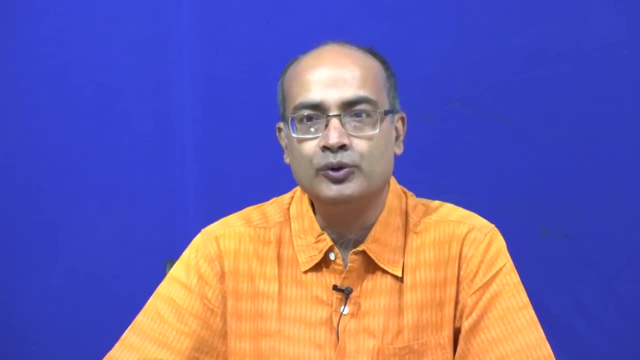 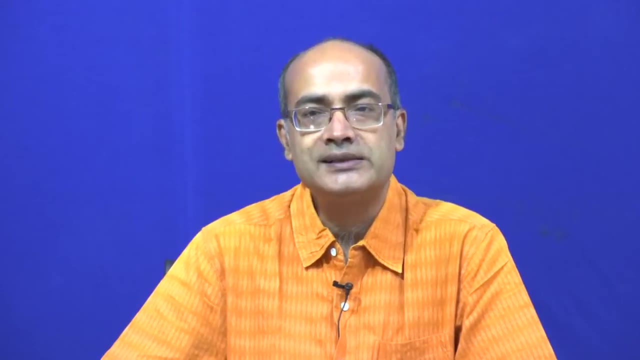 So you would get the introduction about that, you would know that, what are the specifics of that different kind of signals and at the same time you have a brush up of that, the syllabus which we have taken In the first 8 weeks. so you have gone through that, you have covered through the whole syllabus. 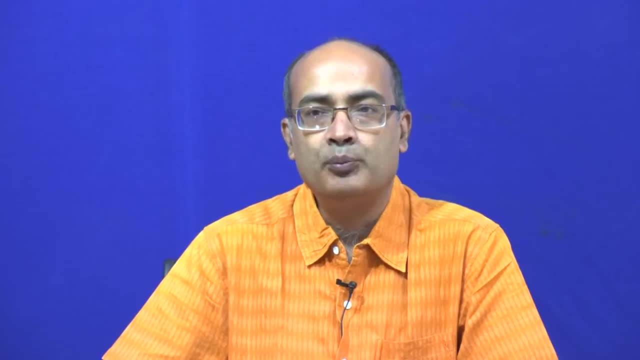 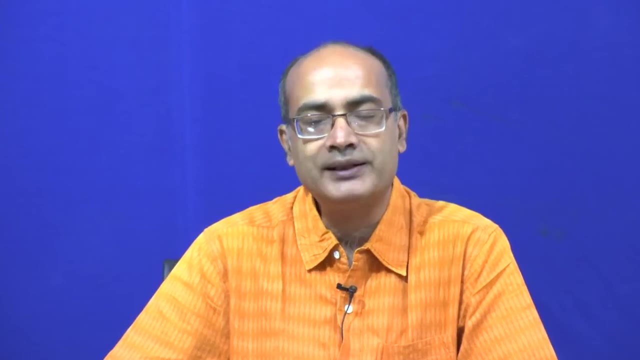 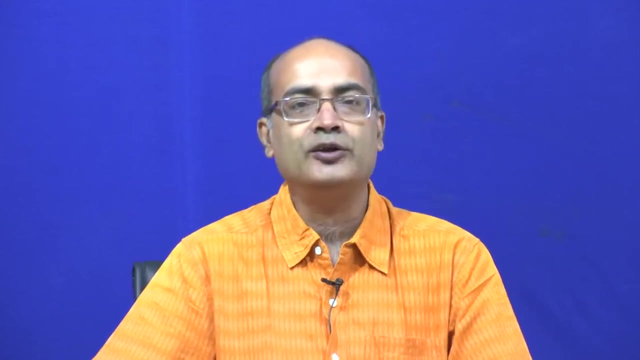 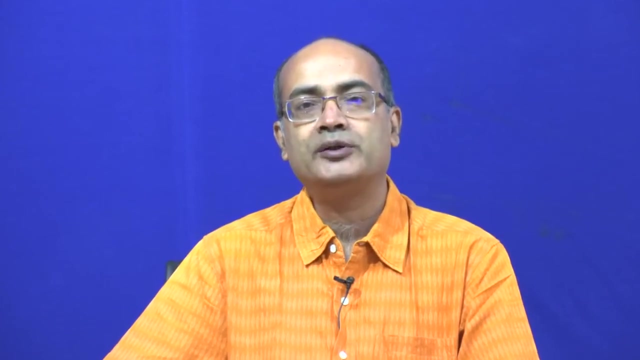 and I think you have also participated in answering the assignments of that. So that itself is a good practice, actually for the exam. So in the exam you would get very similar kind of questions, maybe a little deeper, because over the time, Over the time, you are expected to have more insight into that subject. So few questions. 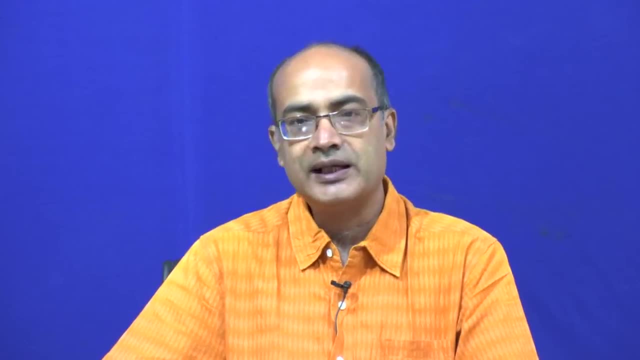 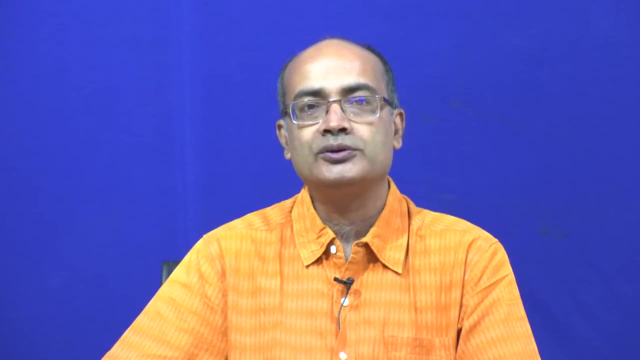 would be there which would be just like that. that assignment, very easy, some of them, if you just read through that course or just listen to the course. even you are unable to do the assignments. you should be able to answer. For few questions to answer, you need to have. 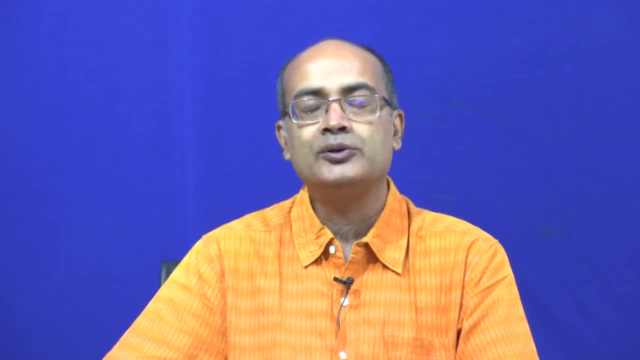 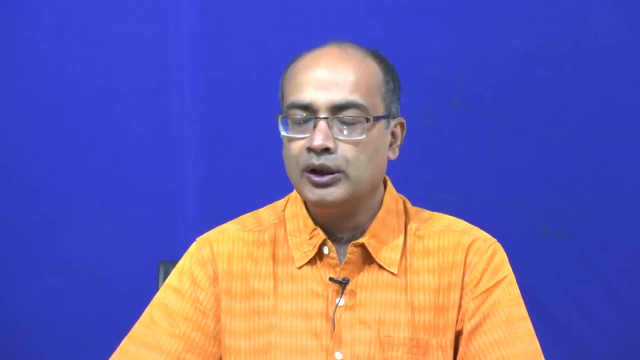 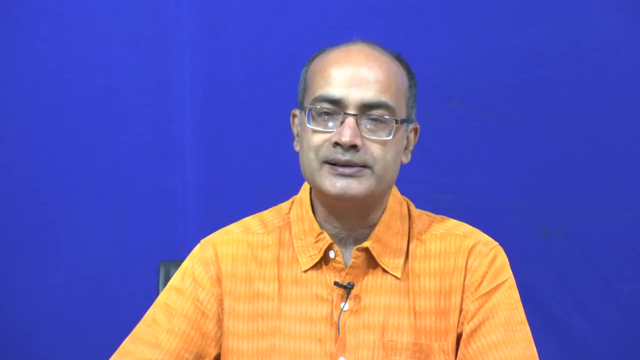 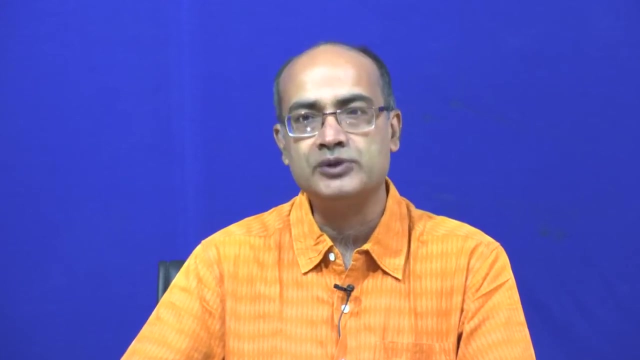 that practice. So this is of actually writing those assignments, and for few of them you need to learn a little more, you need to go through the books and to get a little more understanding. So, primarily, that the questions could be divided in this 3 categories in terms of difficulty. 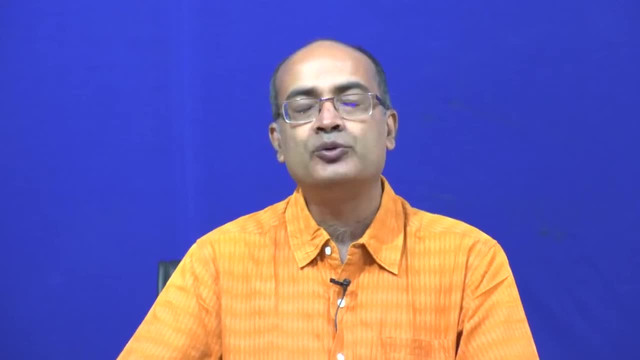 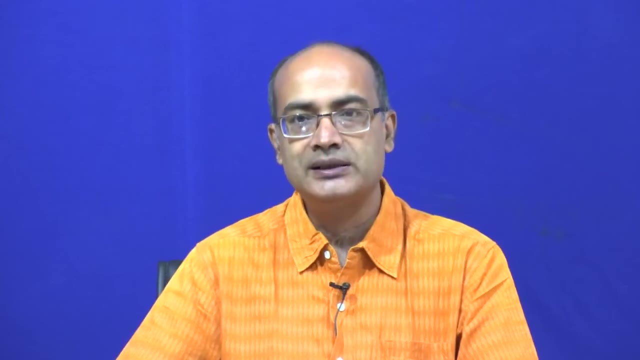 though all of them, there would be short questions There would be. each one of them would be a of 2 marks of, and you will get 50 such questions, So that you get 100 marks to answer within that time. So we will have plenty of time because they are objective type actually questions and 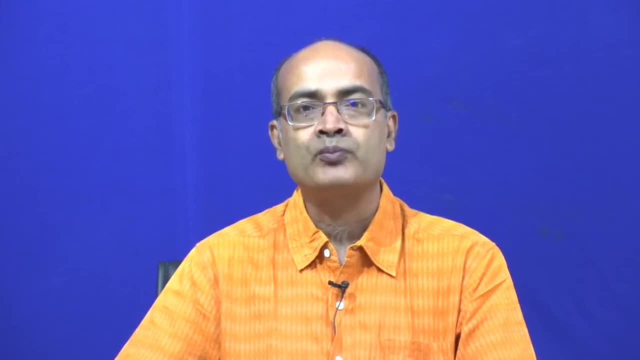 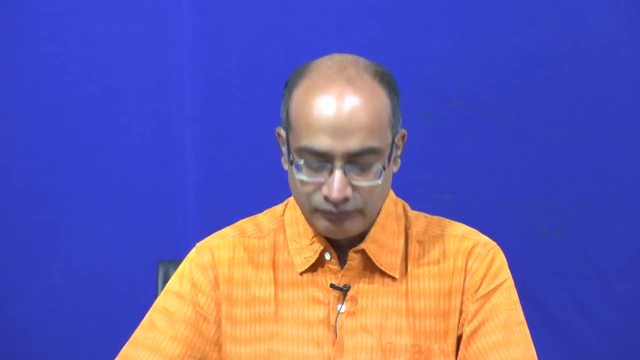 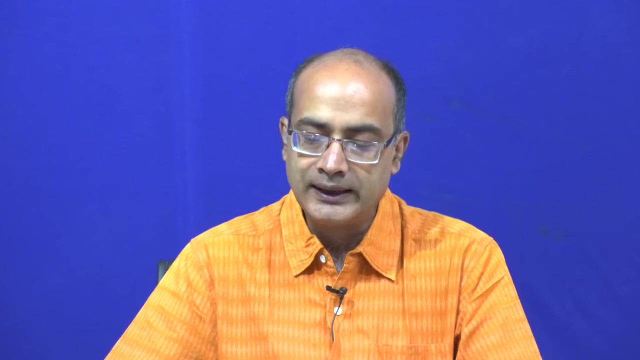 I do not think that you will have any difficulty in actually finishing that the question in time. We got one more question from Ashish Kumar Dhaka. Ashish Kumar Dhaka: He says how the morphological characteristics are used to use as a feature and classification. 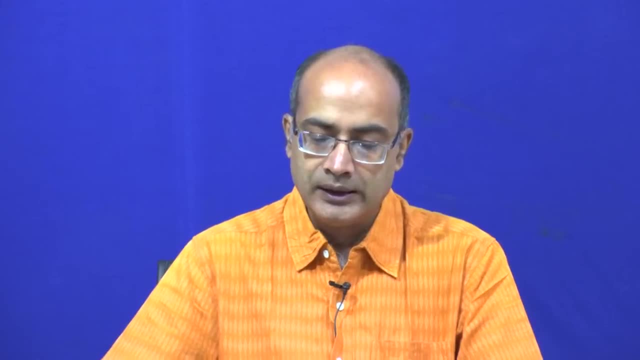 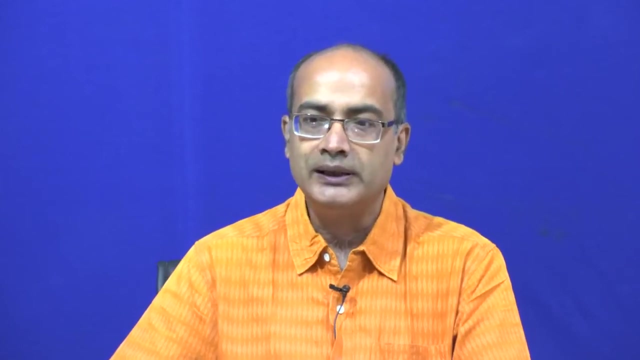 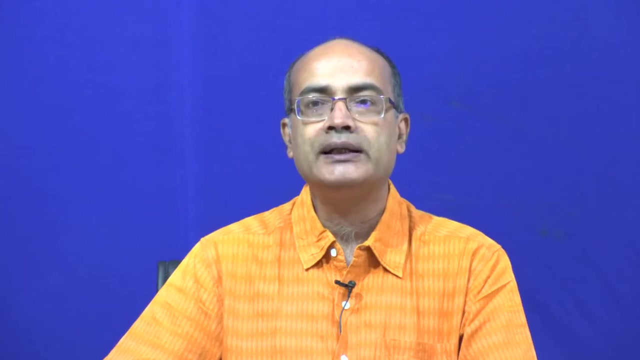 of ECG signal. That, in case of ECG signal, that we look at that, the different kind of characteristics, for example, that the first thing, first thing, what we look at that, what is the rate at which we are getting the ECG signal? 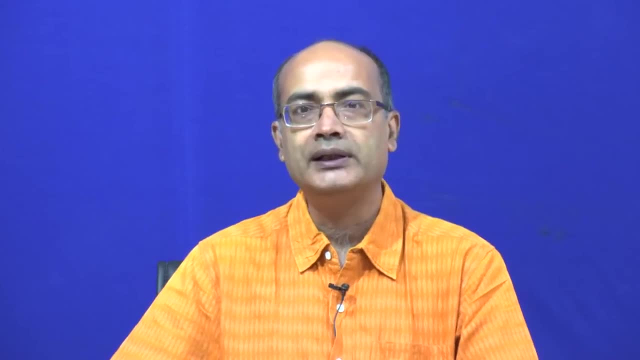 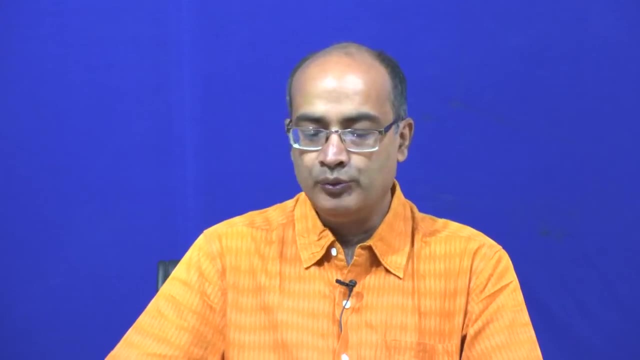 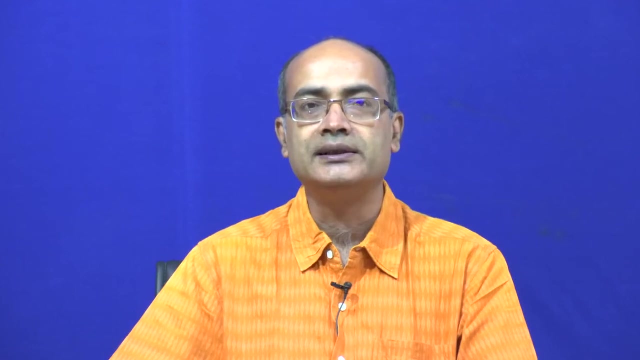 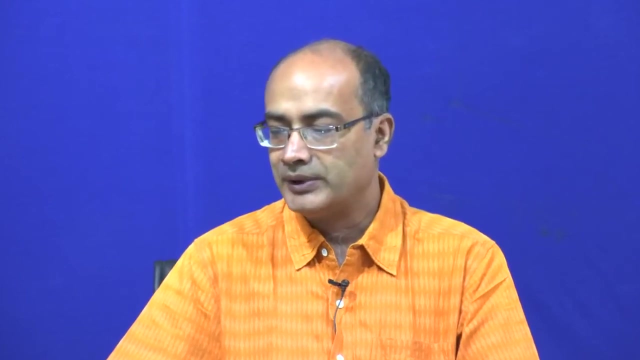 For that. we look at that when the beats are arriving and the interval between two beats, which we call as RR interval, we actually take that. that is the first signature for the ECG. Then we look at that. other characteristics. you know that the people have tried correlation. 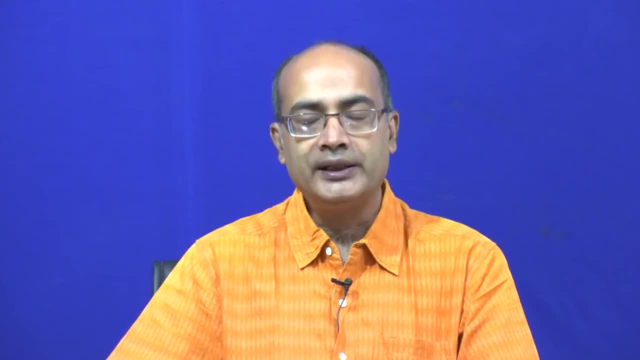 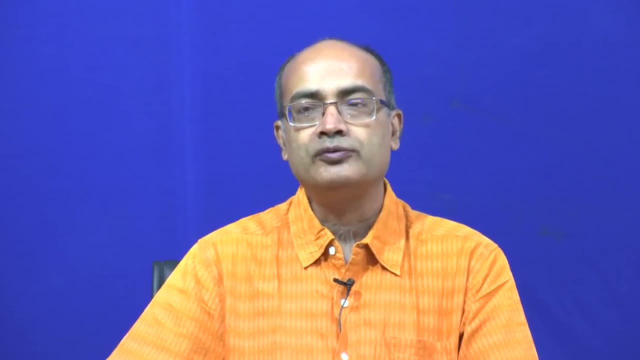 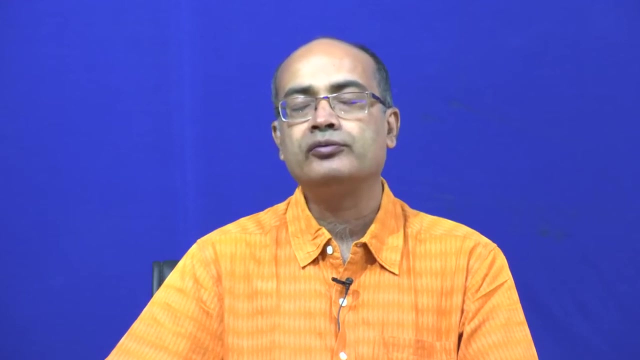 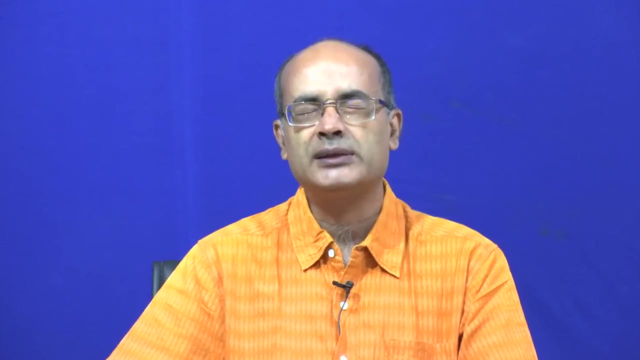 that is one. then due to ectopic beat, that the QRS complex may be jagged because of, say that, deprivation of the blood or supply of oxygen, Then due to that lack of blood supply, which we call as that infraction, and then ischemia, 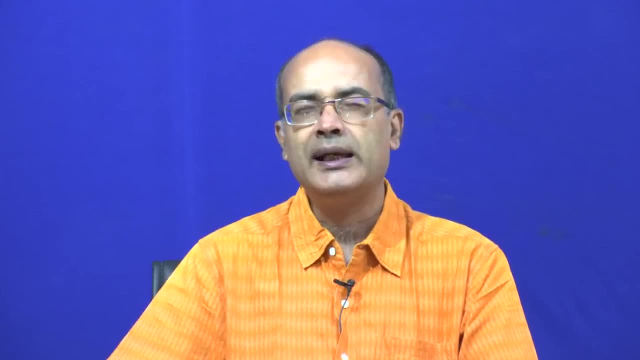 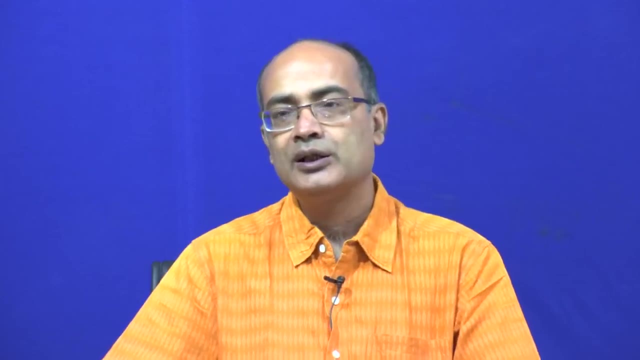 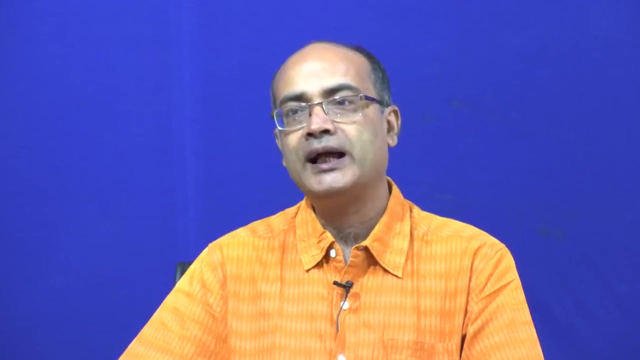 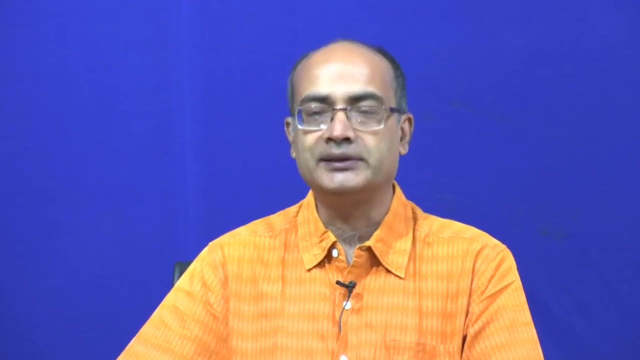 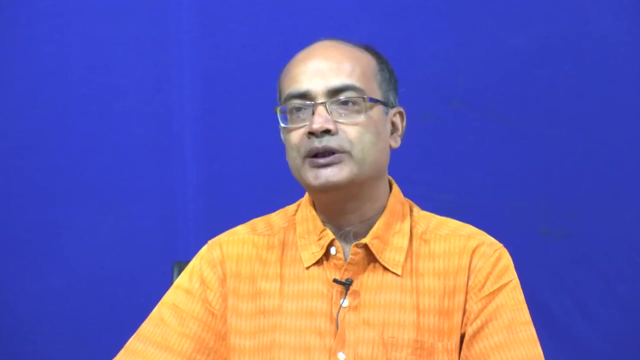 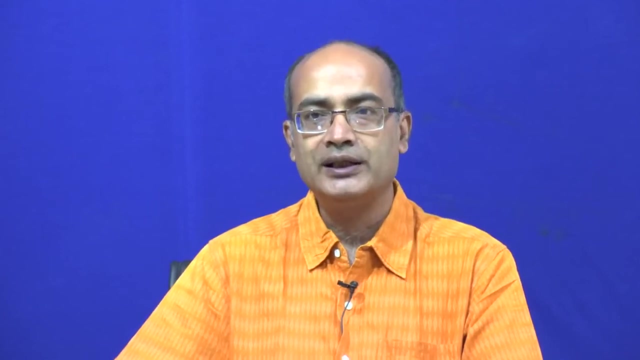 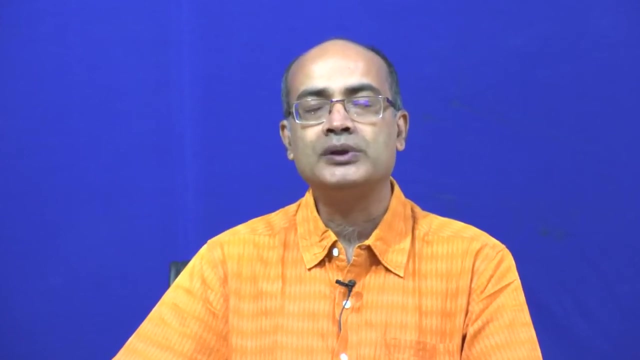 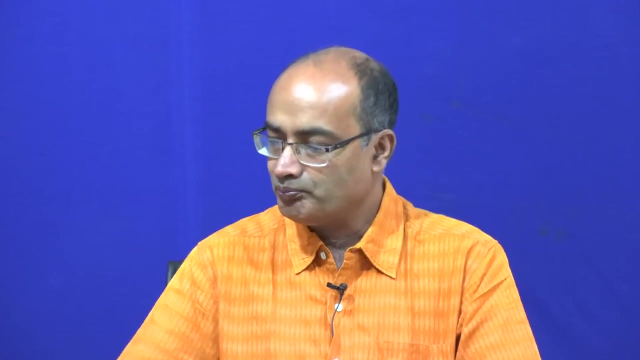 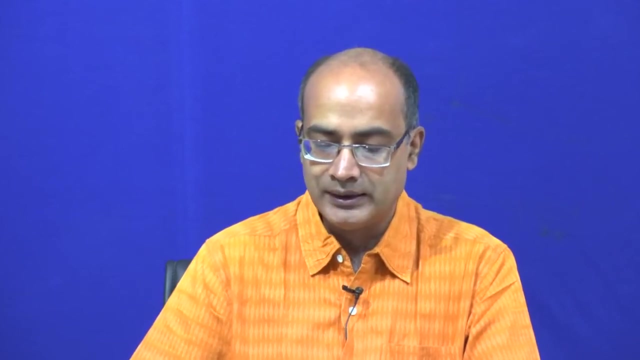 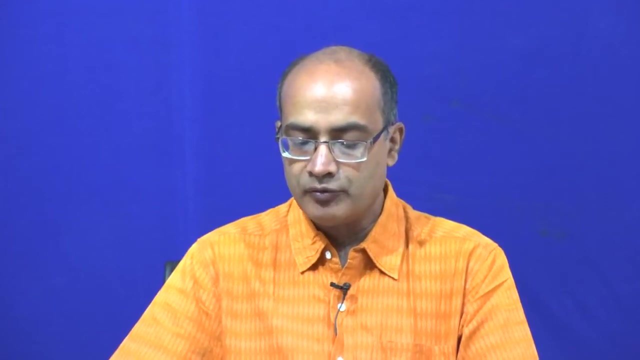 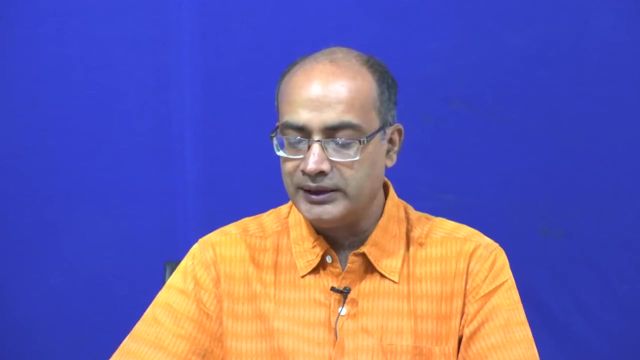 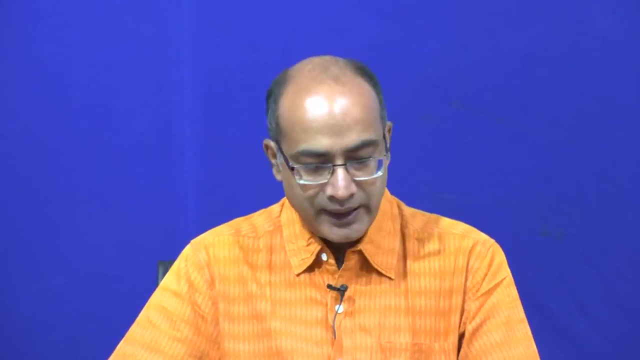 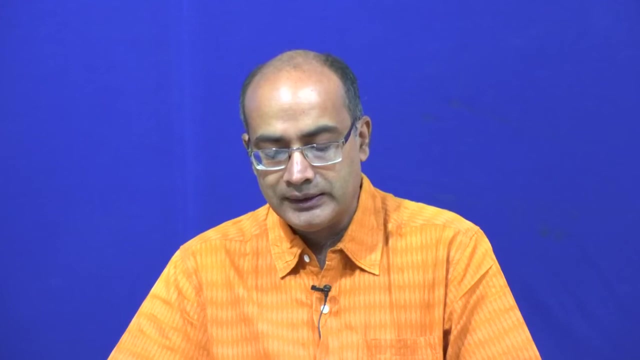 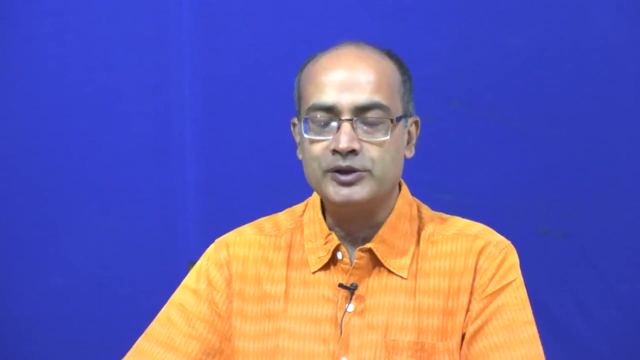 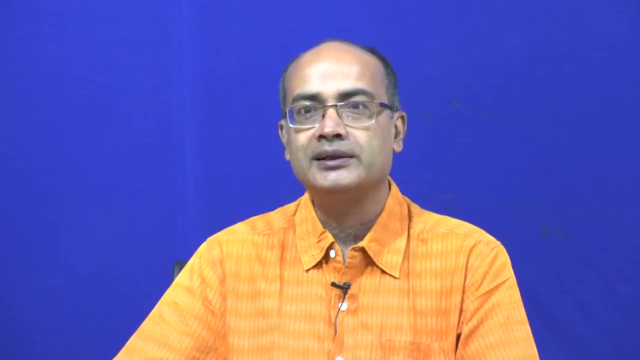 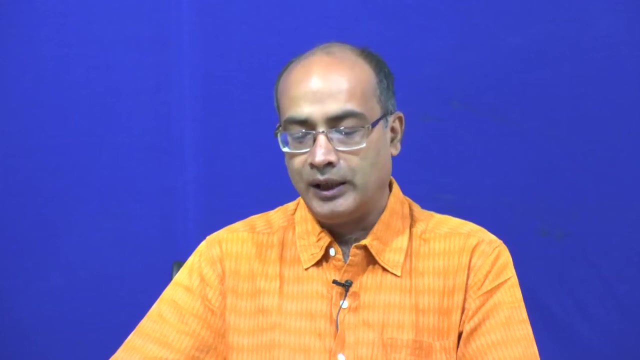 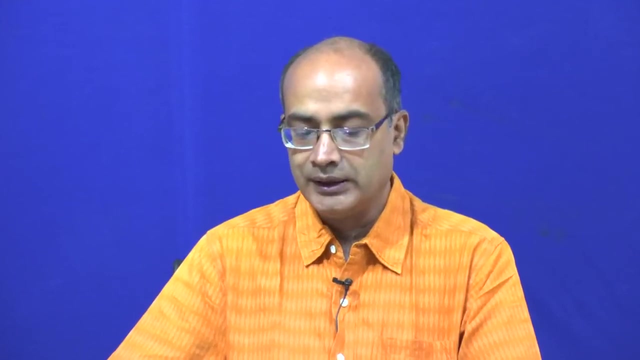 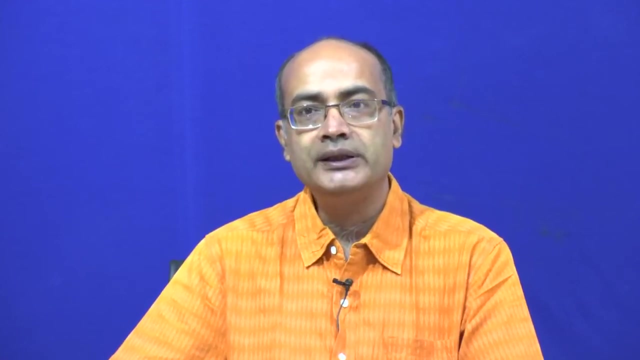 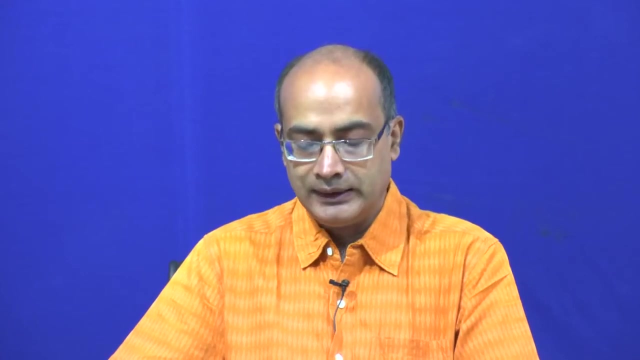 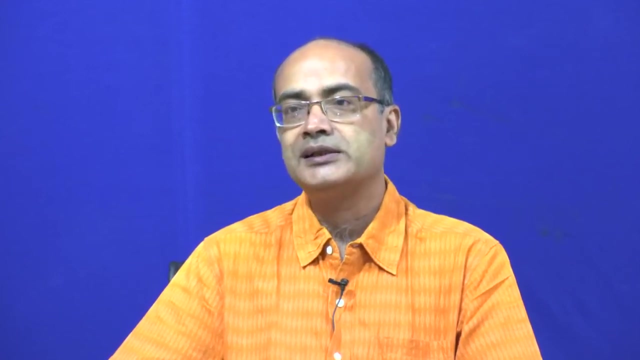 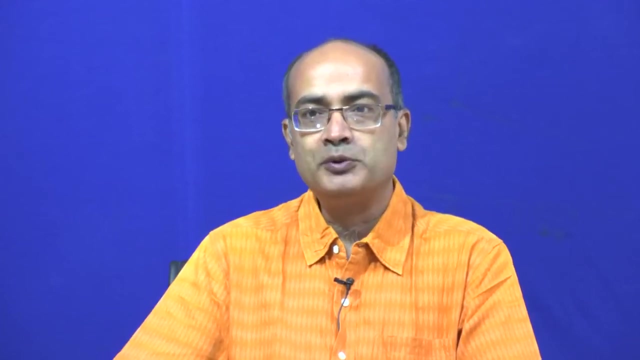 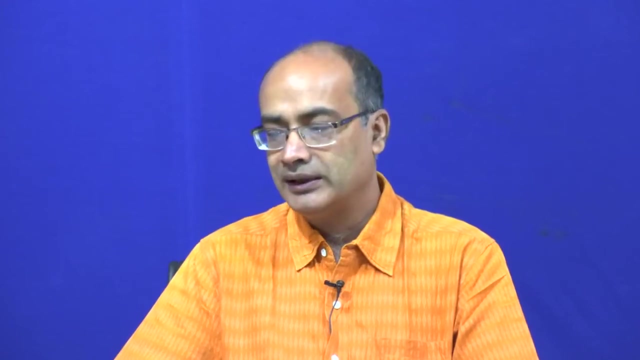 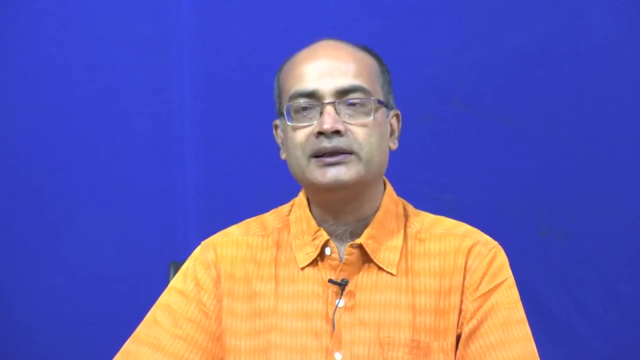 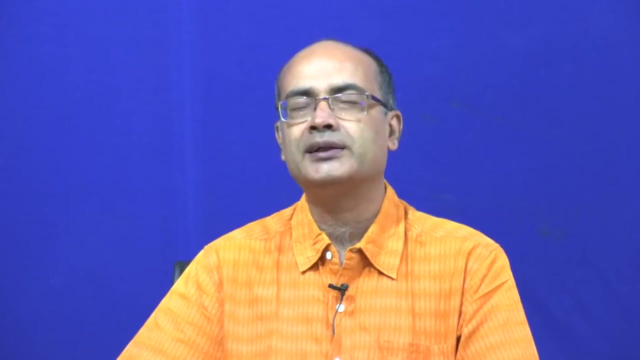 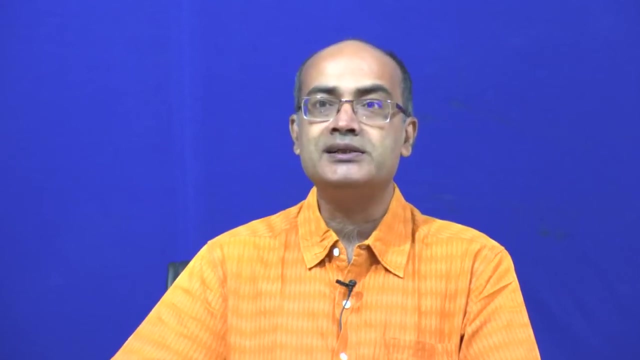 that in such conditions, we know, the ST segments get elevated or depressed. So all these changes we have quantified in a little different way. rather than trying to take that as a shape, we have derived it as a lump parameter. Why it is less in India. 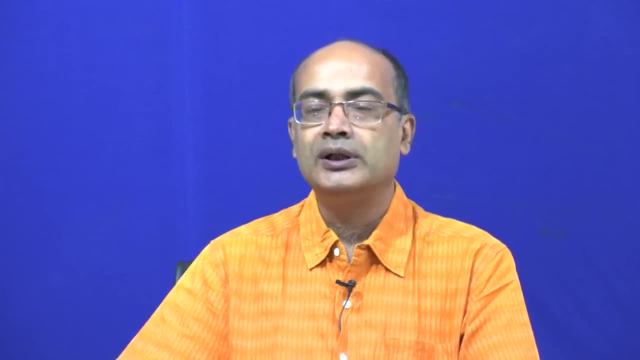 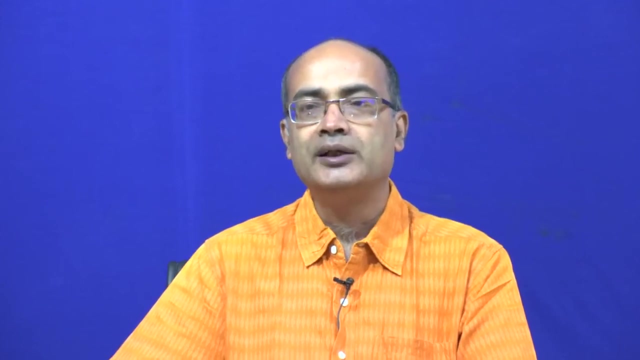 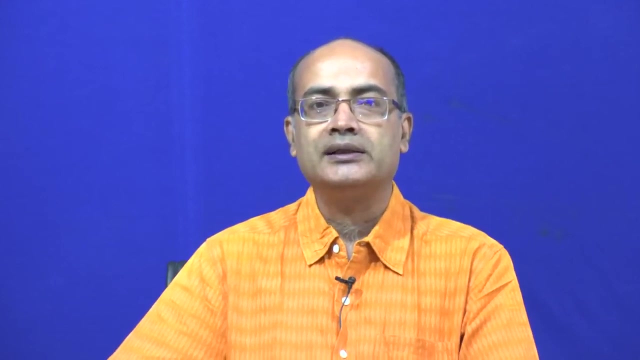 The first point, I would like to tell you that for the medical device there are some regulatory bodies you need to first take, actually, their approval, unlike other technologies- say, you make a new mobile phone or you have a new technology, that which is used for some kind of purpose. 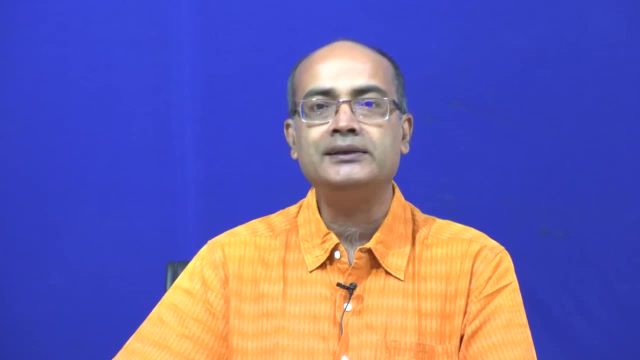 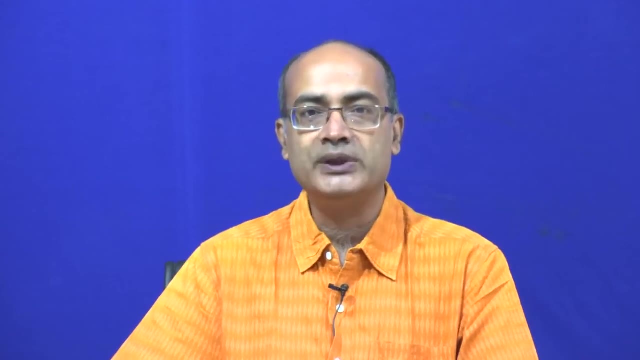 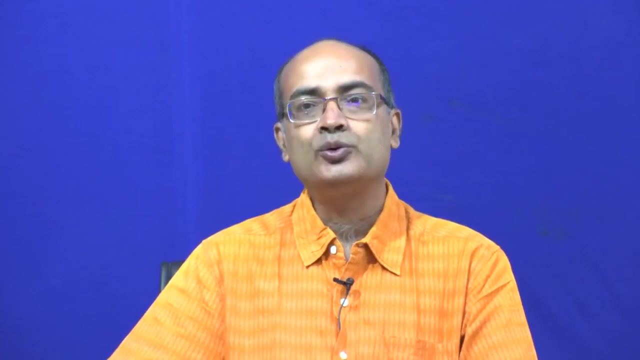 Unless there is a safety concern, you can directly take it for use. On the other hand, because you are talking about the human subjects, so safety is for utmost importance. so first you need to take it through the clinical trial and then only you can actually think of using it. 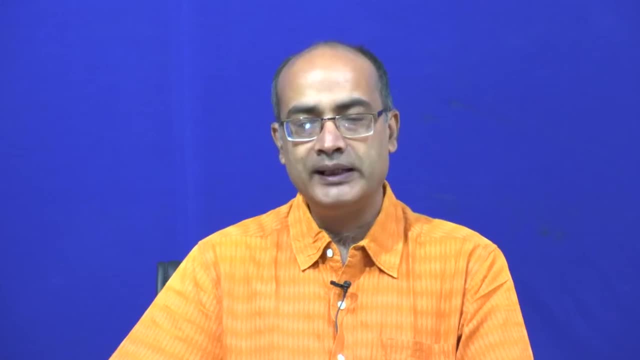 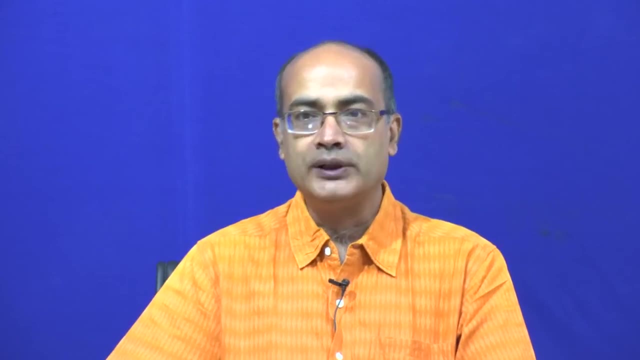 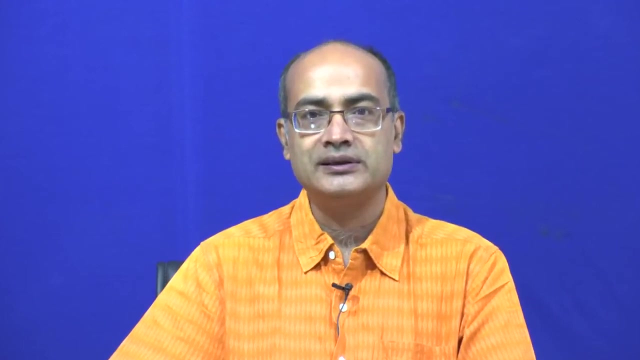 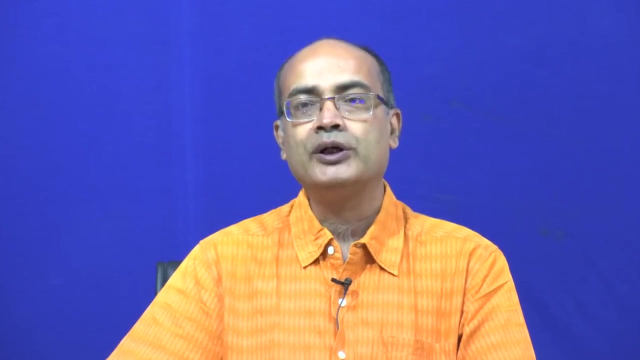 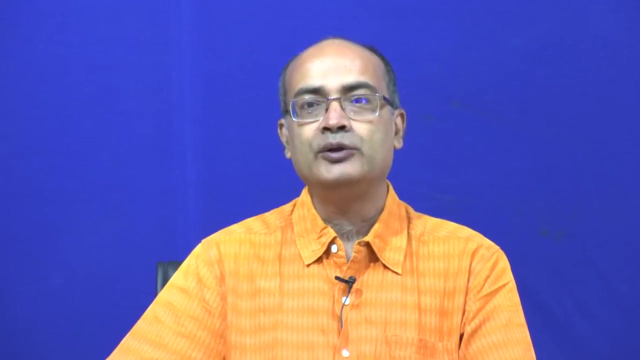 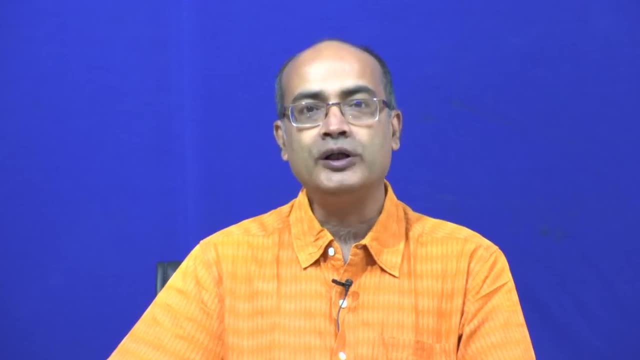 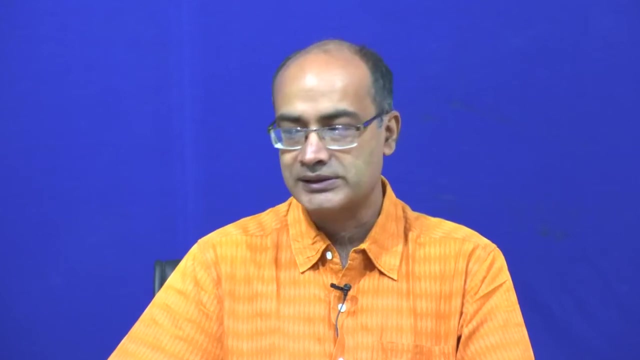 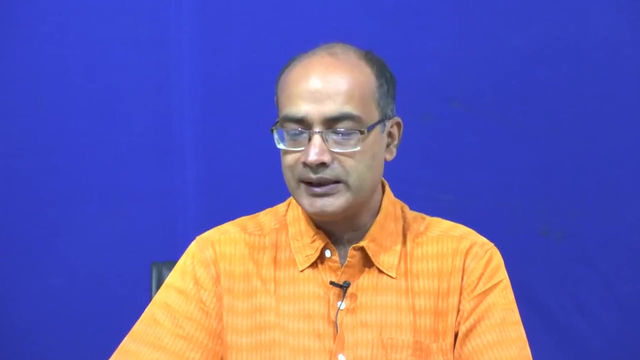 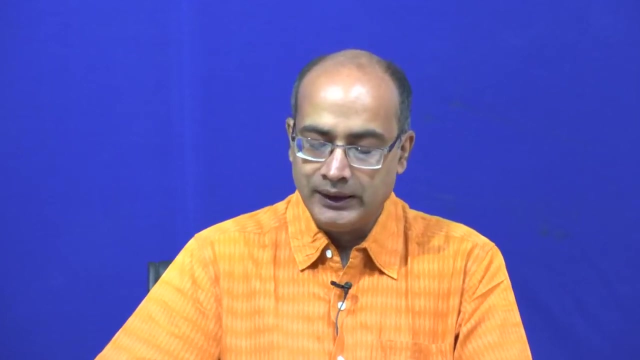 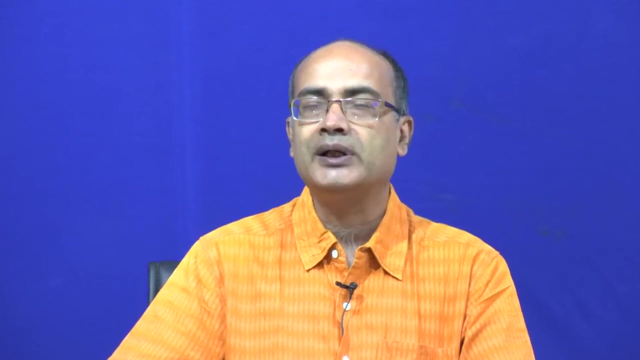 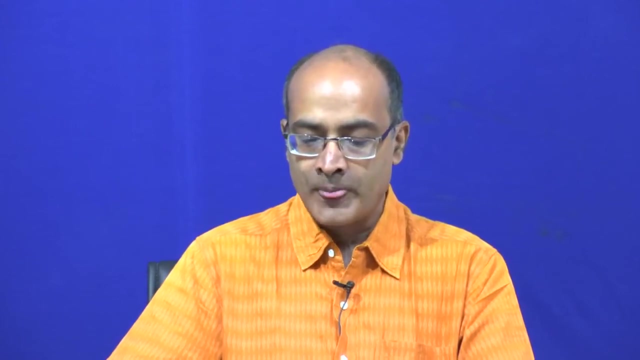 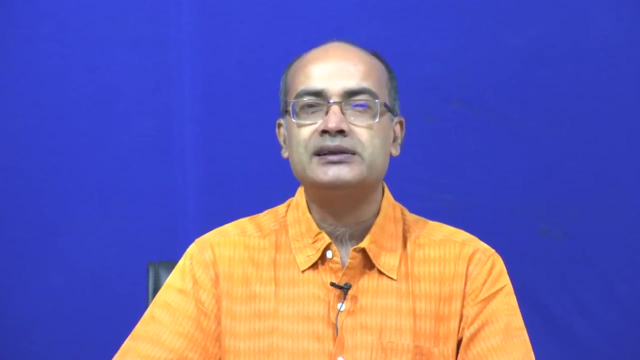 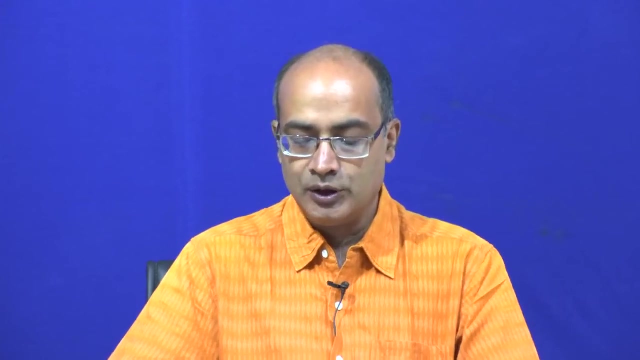 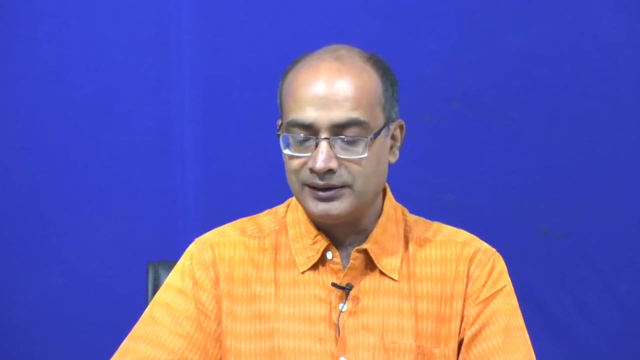 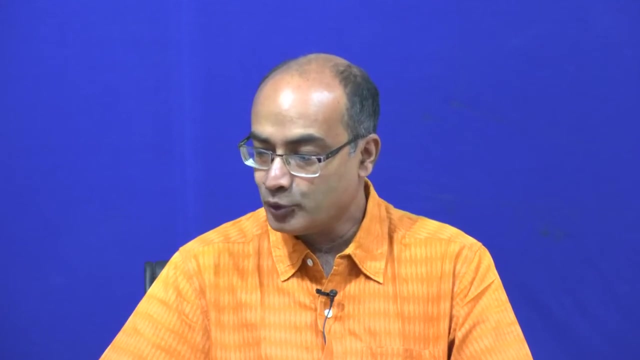 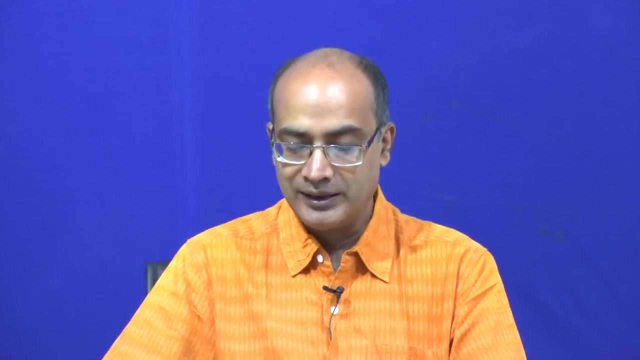 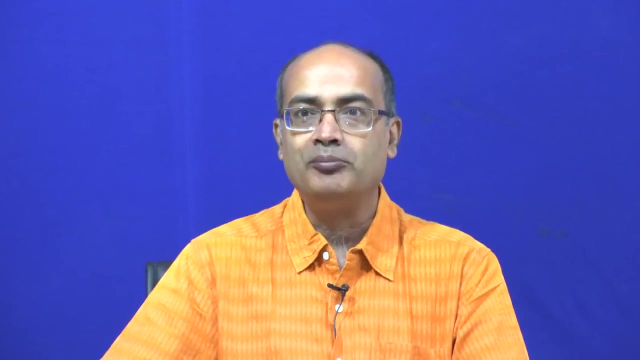 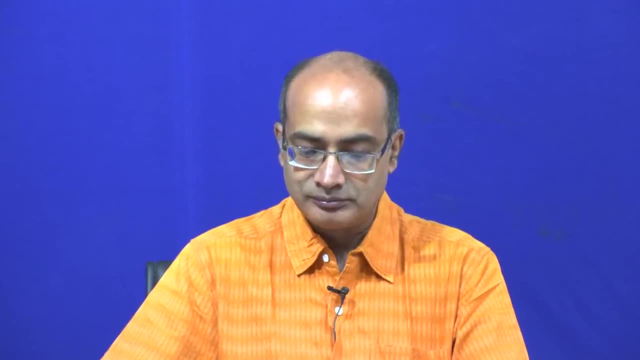 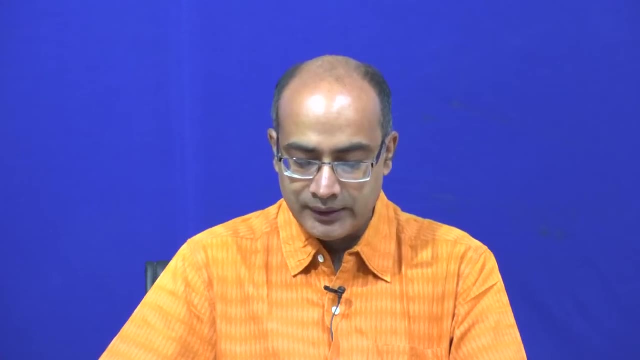 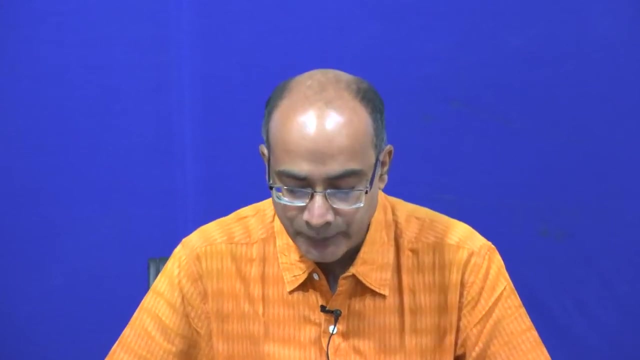 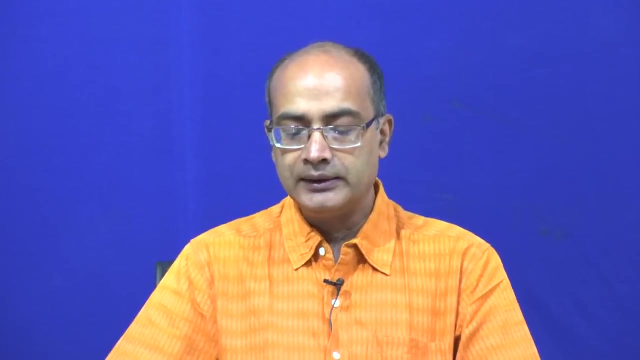 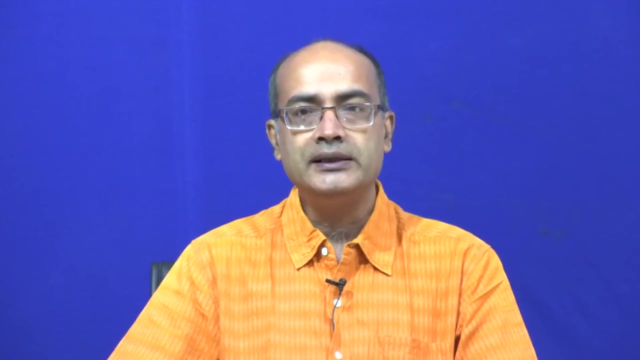 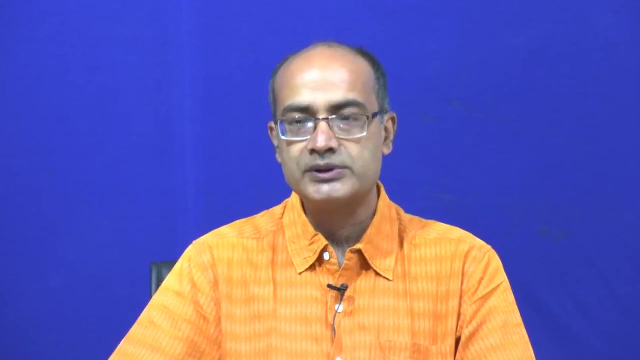 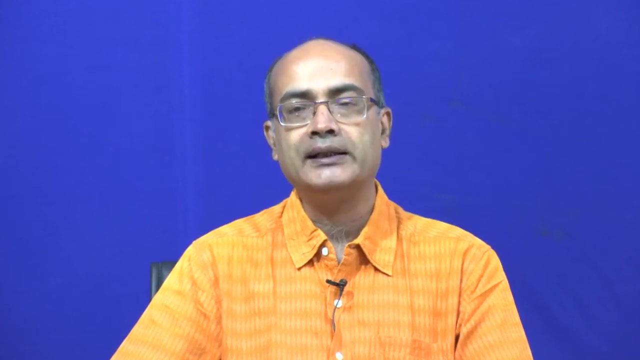 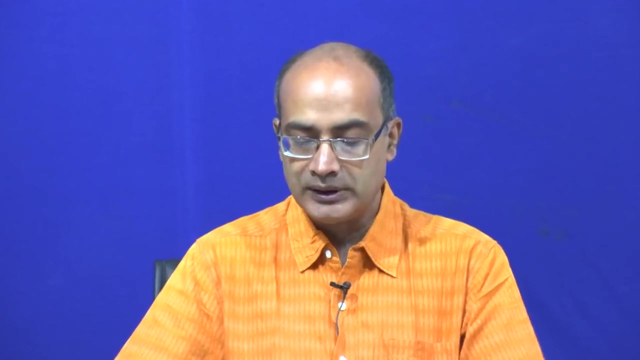 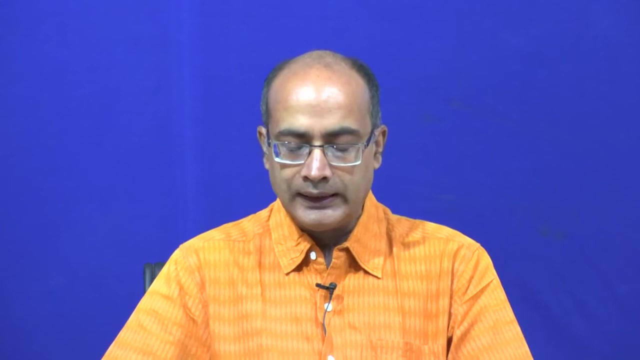 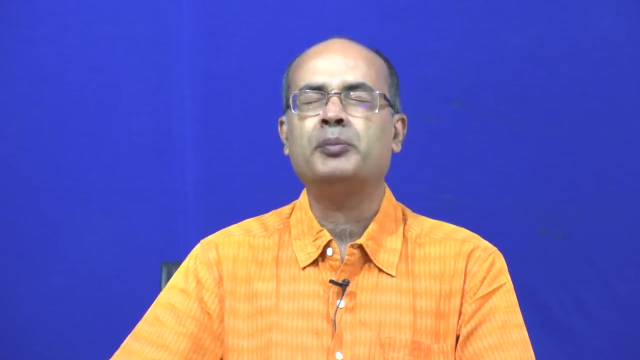 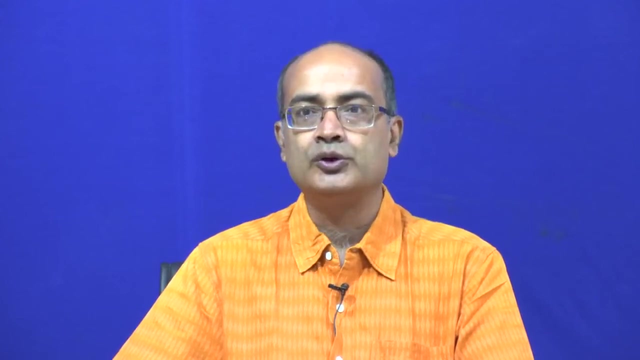 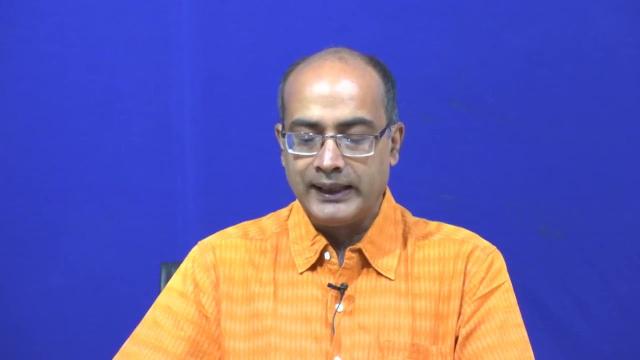 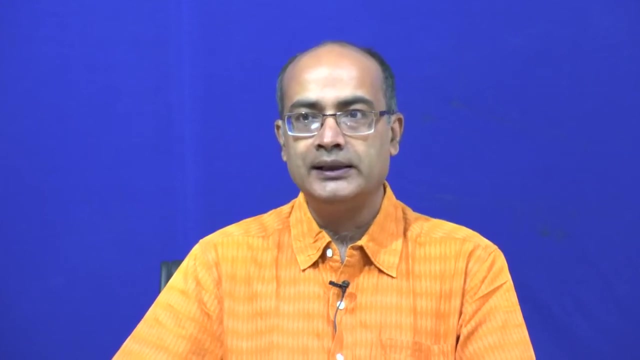 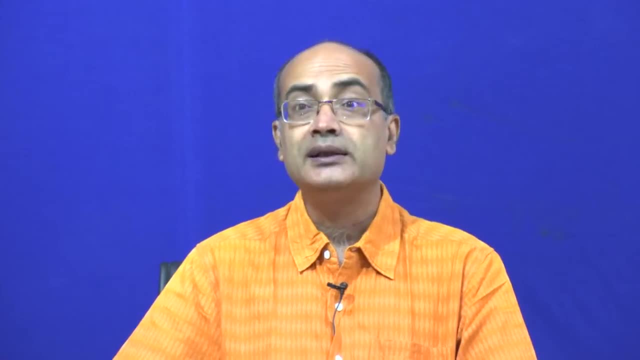 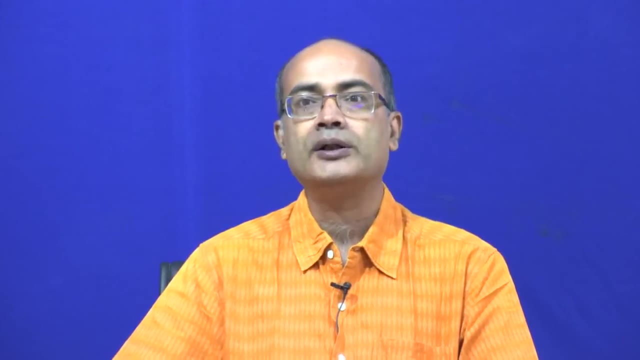 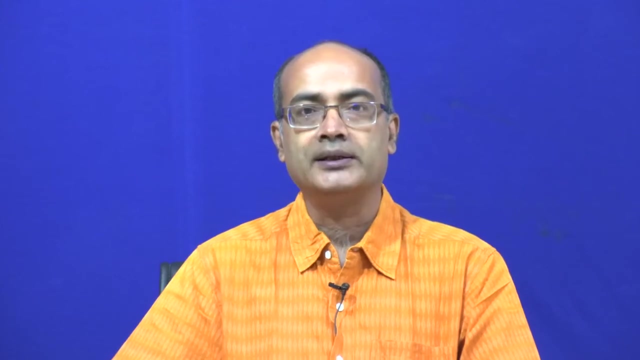 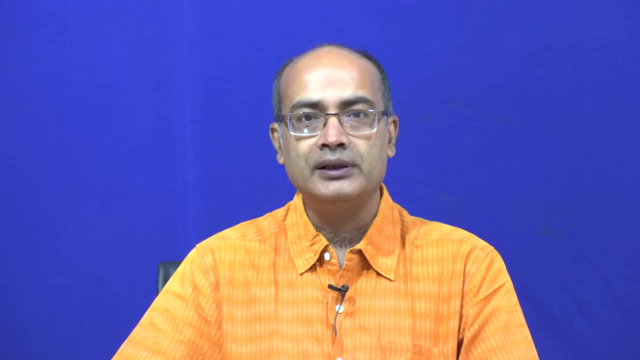 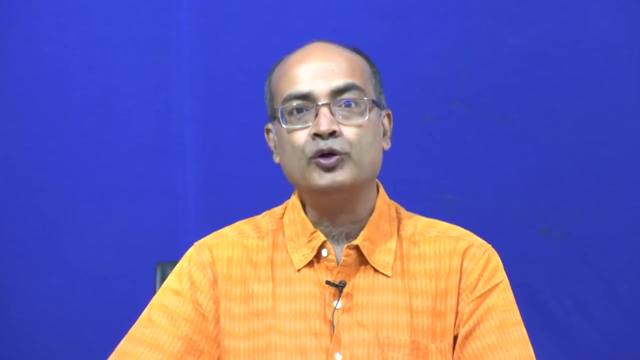 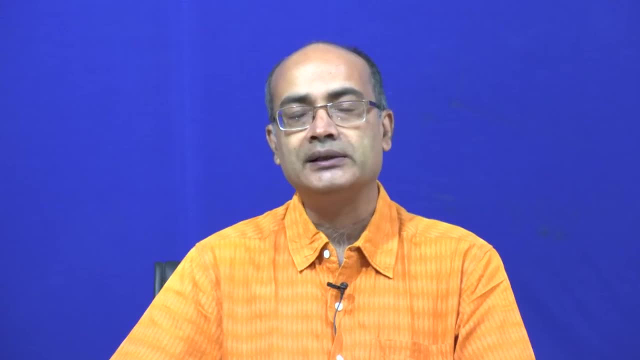 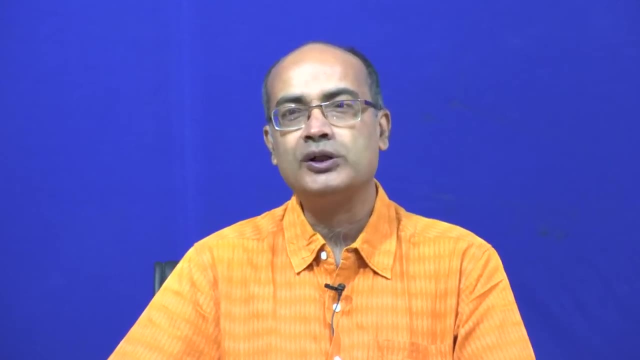 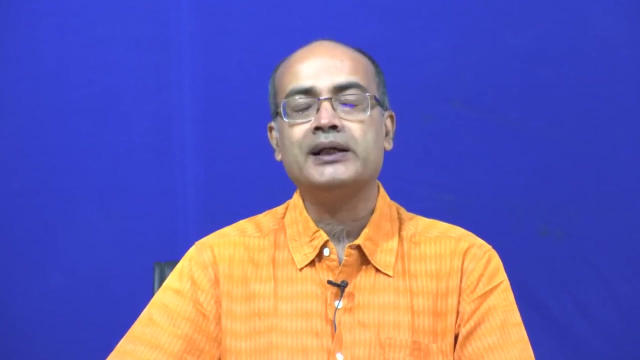 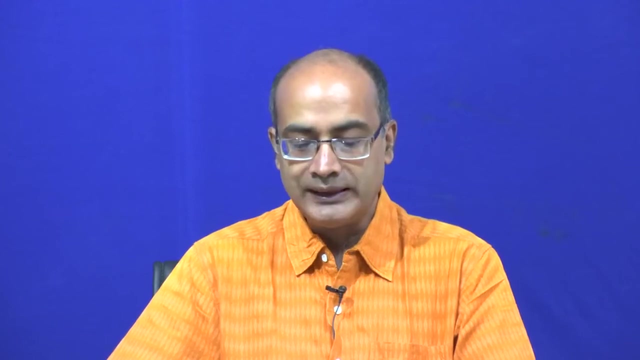 And there are different Japanese companies, that Fuji and all they are making actually equipments for some modalities, not for all, ok, And there are actually disruptions. new players are coming, for example that Samsung, now their R and D, they are working on that MRI and the CT scan machines. 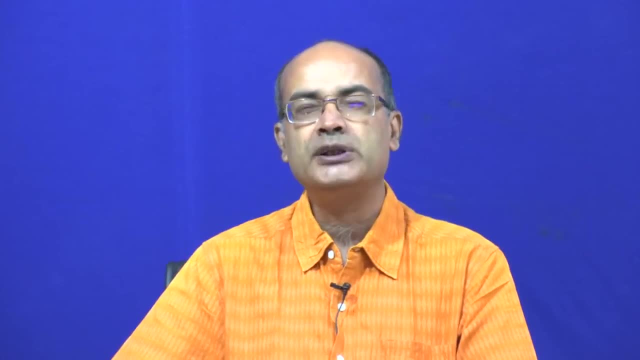 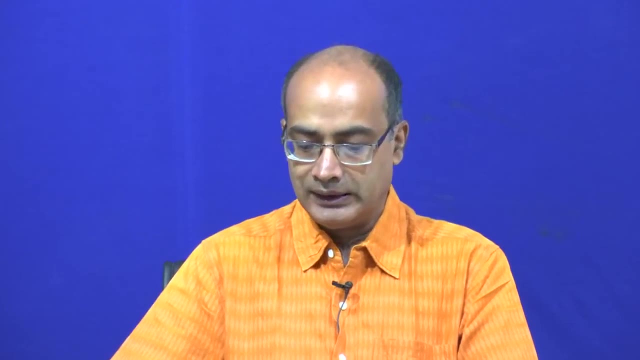 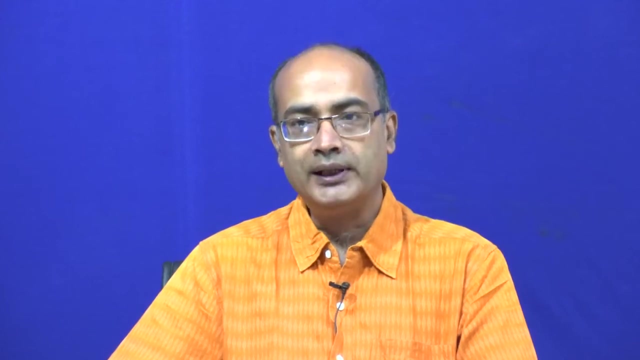 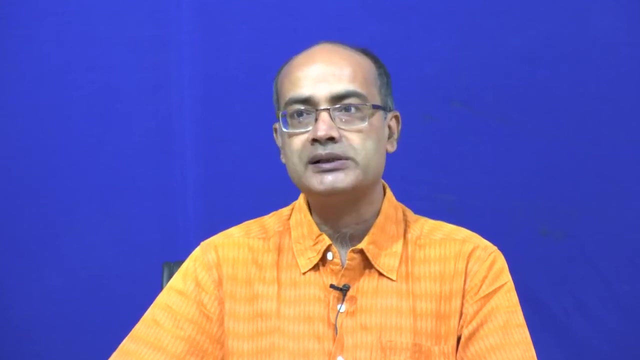 So they are trying to take that position as one of the big player in the world market, So that- and they are working from their country, that is, their base country is their South Korea as well- as they have a big lab in India, in Bangalore and Gurgaon, in other places- 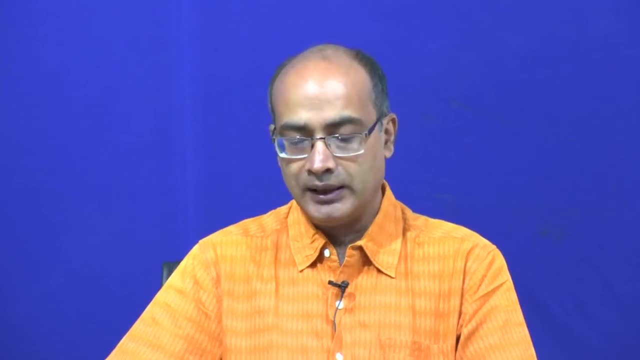 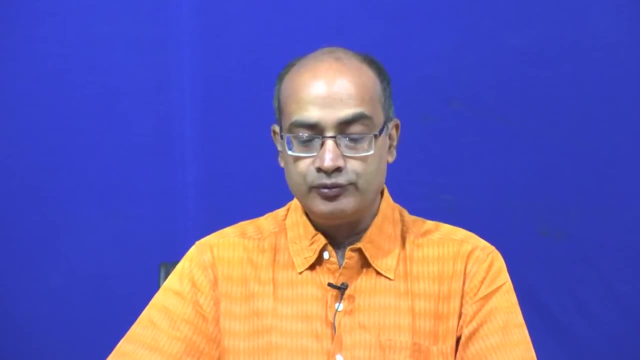 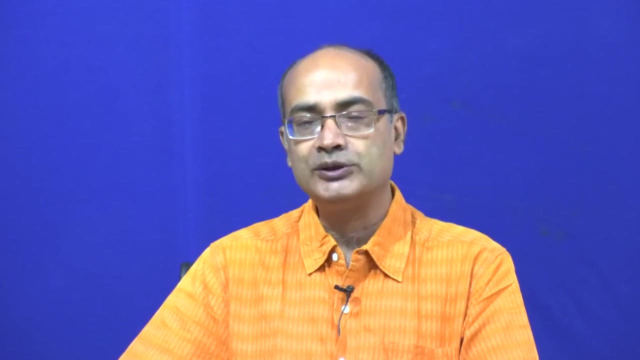 So they are also working from India And they are working for For these equipments like MRI and CT scan. And if any other actually business group they want to come, I think that first they need to absorb the technology. what is there in the market? Because for such a big machine, all the things, it is not actually easy to absorb, all of them. some of them need to be outsourced, may be sensor need to be bought from other company to develop that equipment And R and D would be required to create a differentiator. that when you try to compete. 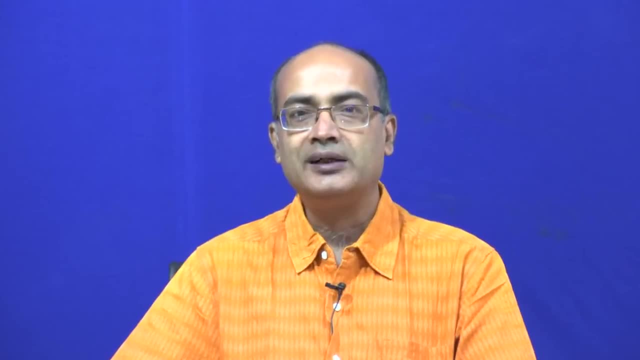 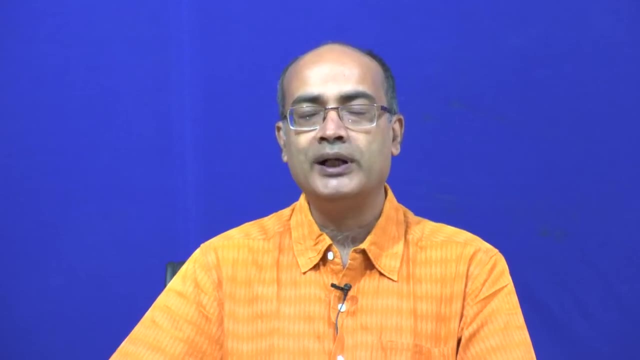 in the market, you will see that the products are coming with new features. For example, when you look for your new mobile, you look at the spec that: what is the size of the screen? what is the screen resolution? how good is a camera? 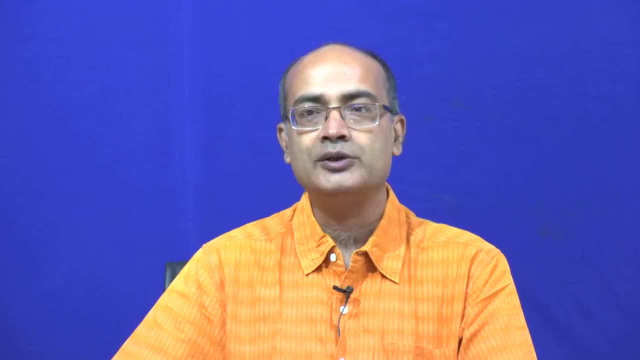 So every day the numbers are moving sharmin into values, so those map can also be given by this R and D, And so, as I just stated earlier, I used the familiar things, those of this, to type slur. we have known what it was there, So it is such common names. 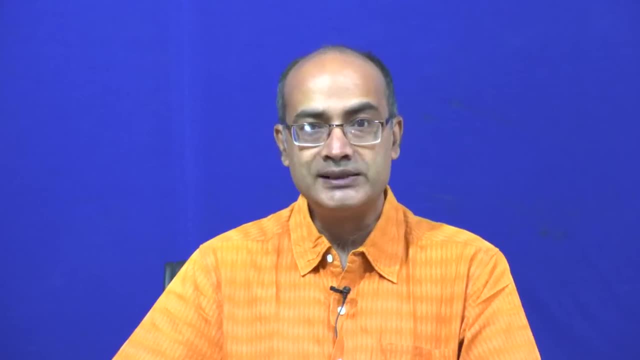 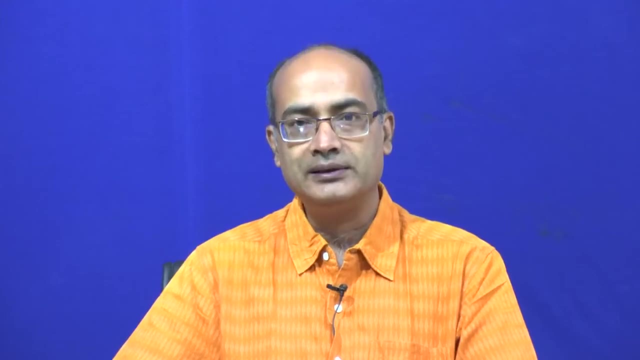 new features are coming in a new model. So when you change that model you need to have your R and D or you need to take it from that, the other R and Ds. you need to take that so that you can make add new features. 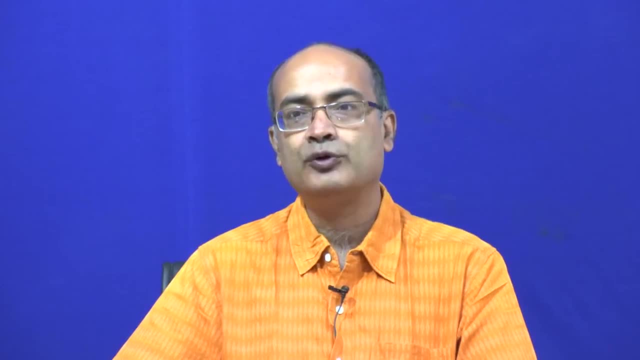 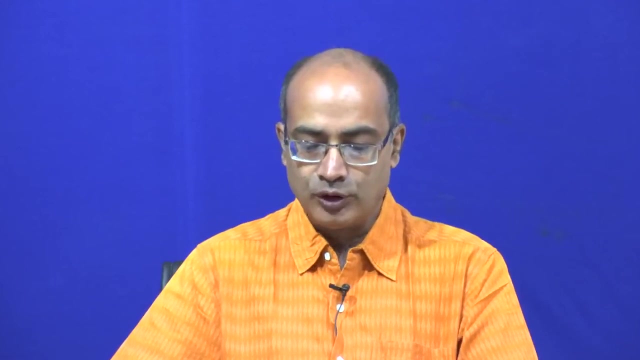 So R and D is primarily required for that, for new generation of the product, but as such, the base technologies of MRI, CT, all of them, they are standardized and for that you do not need to do the R and D for actually at least high, actually high end R and D for. 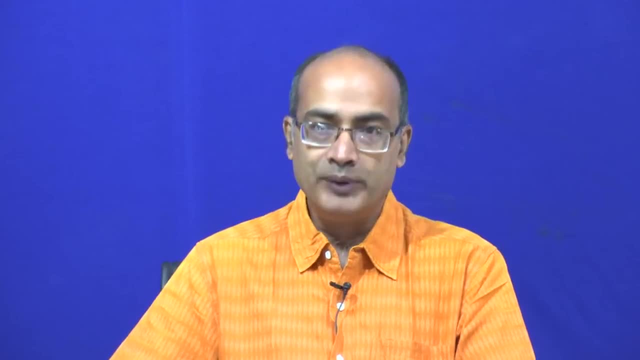 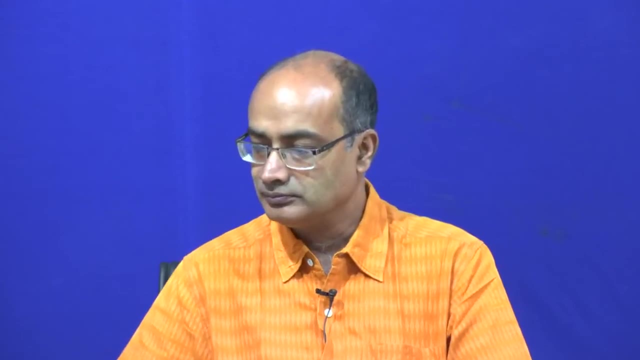 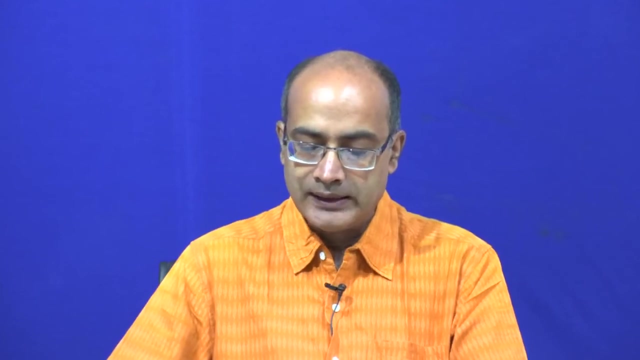 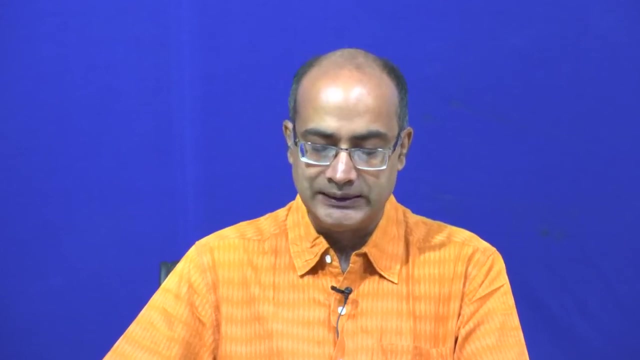 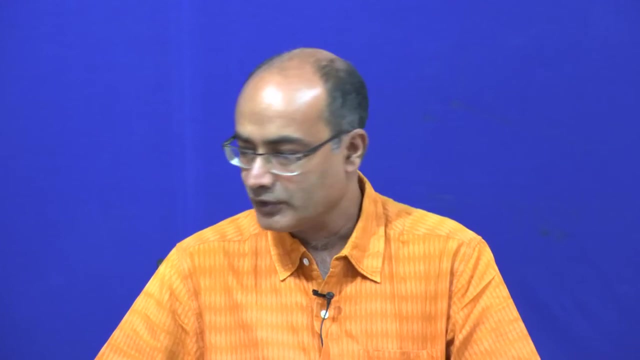 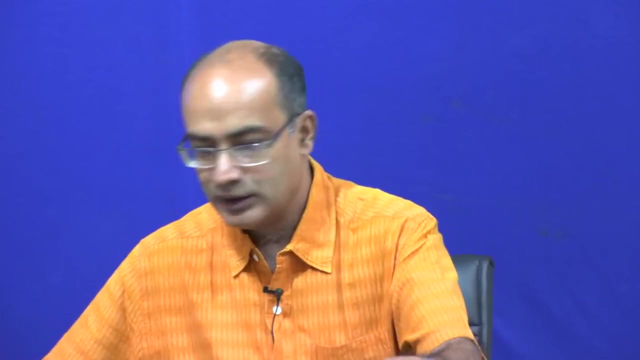 that ok, Though that- how to make the prototype and all that itself also would be a pretty good challenge. So thank you. Next question is from Rohit Apurva, why P and T waves are low frequency signal. ok, Let us look at that, the ECG signal. so what we can do that if we look at the ECG signal. 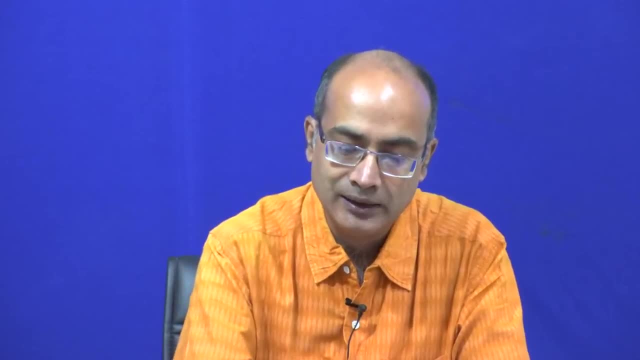 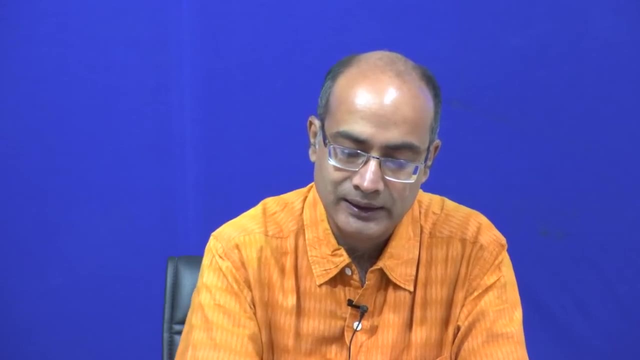 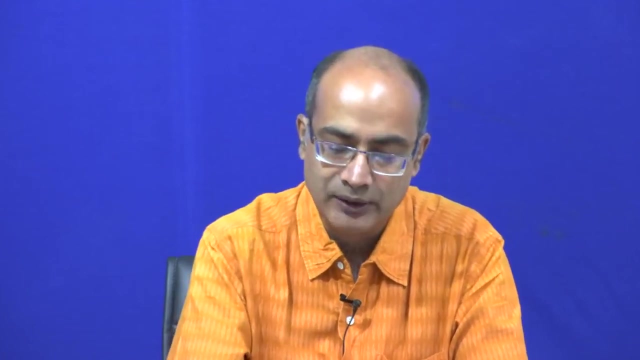 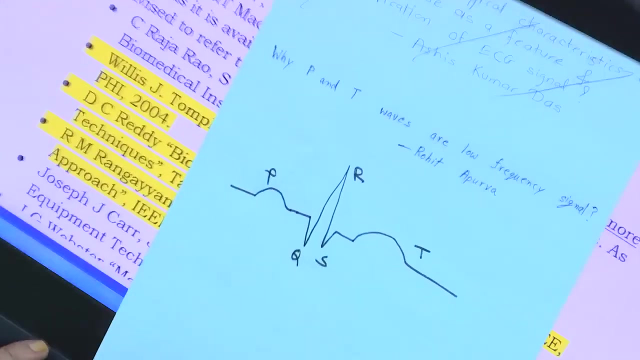 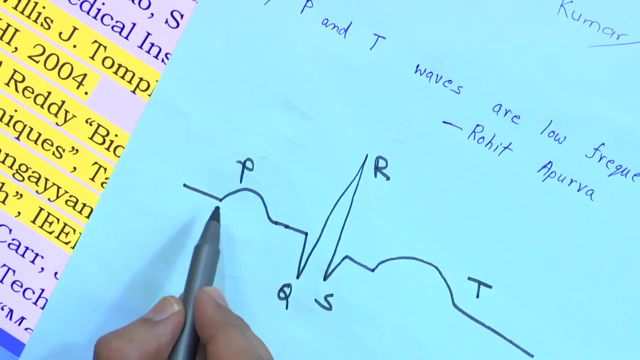 that this is P, Then followed by QRS, then T signal. this is a lead to signal we have taken. ok, So that here we have drawn that. now, if you look at that, what are the events going on? they are not there that there is a P that is signifying that start of the contraction. 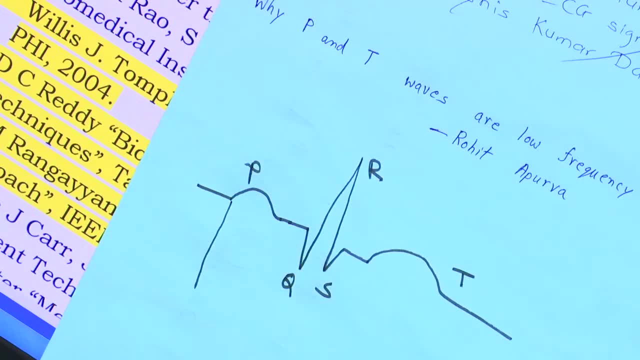 of the upper chamber or the atrium And atriums. if you look at that, they have very thin wall and have very low amount of muscle. Why that is so? If you look at the heart, that four chambers that they are, job is just accumulate upper. 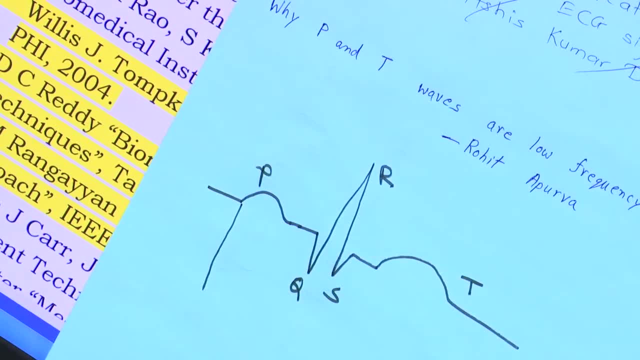 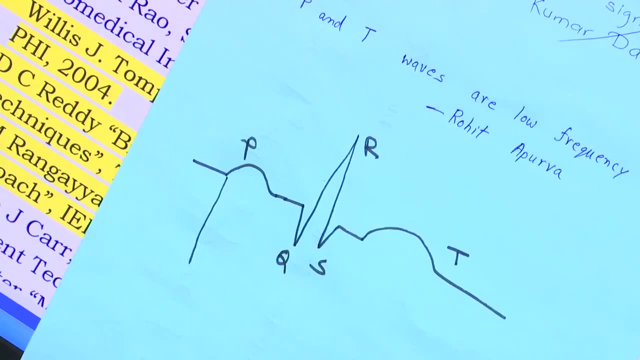 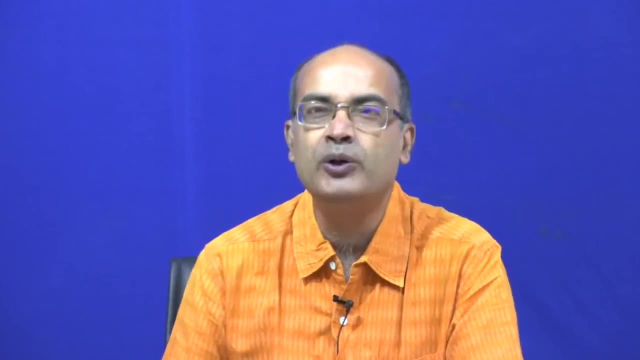 chambers. the job is to accumulate the, that blood which are coming from the vai yourmberine, That many of those are coming from that. four chambers and just it should have the pumping capacity good enough to pass it to the chamber just below it that is the ventricle. So there that is a need, that big muscles, so the activity of it is lower in magnitude. that is one part, as well as because they are slow, that low intensity actually activity. there is no special nerve fibers to distribute that signal so that they simultaneously get. 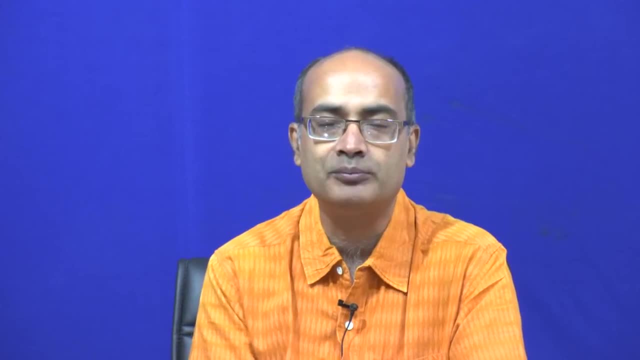 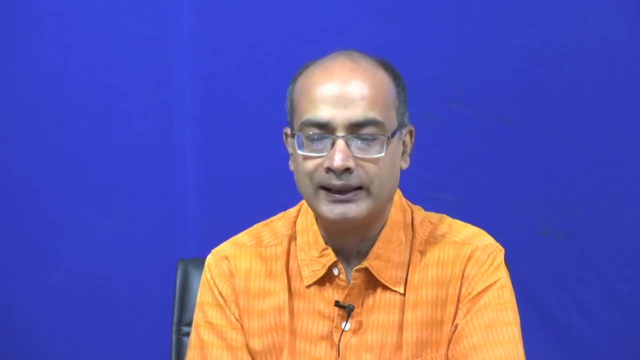 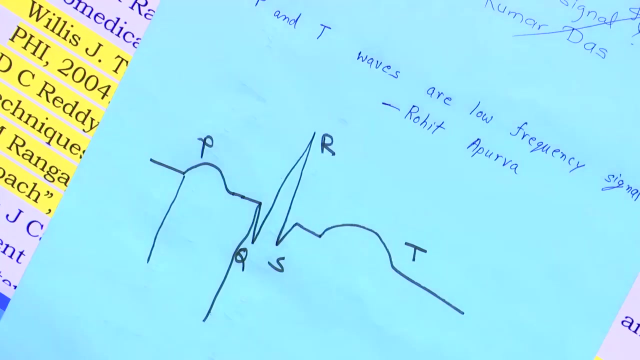 compressed all the muscles of the upper chamber, So the flow of the signal is also through slow through the muscle fibers. On the other hand, when it comes to the QRS complex, That after the AV node there is a network of actually that the nerve fibers that we 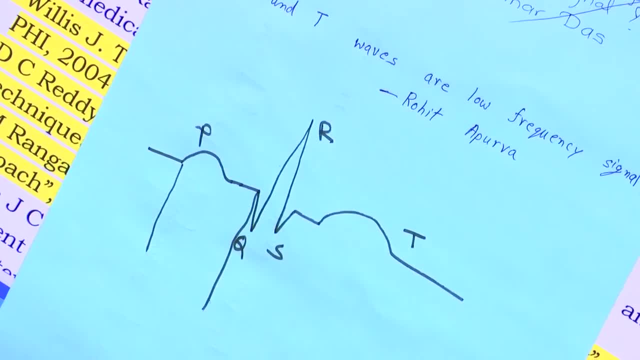 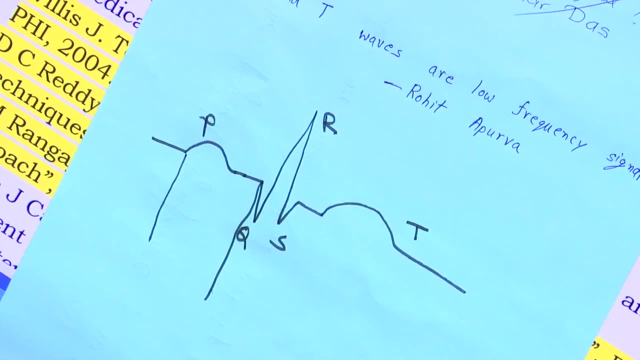 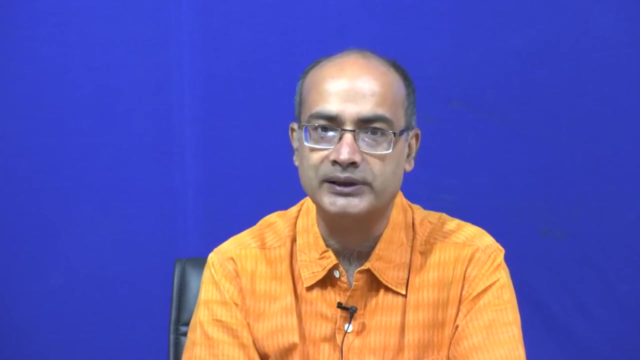 have the bundle and then bundle branch and then the parkergy fiber which distributes the signal in all parts of the ventricles and from there that the ventricles would actually compress simultaneously all parts of them. all on a sudden they start the compression So it becomes actually a much faster action. so that is why QRS complex is actually much. 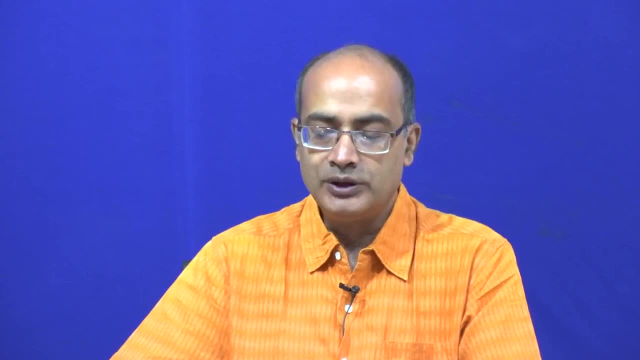 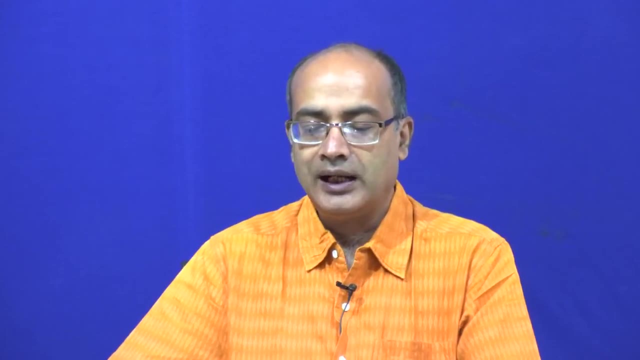 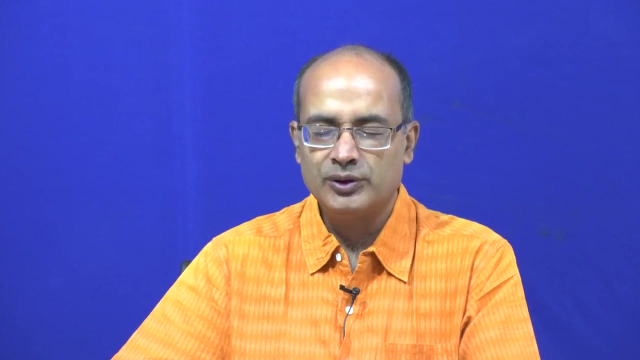 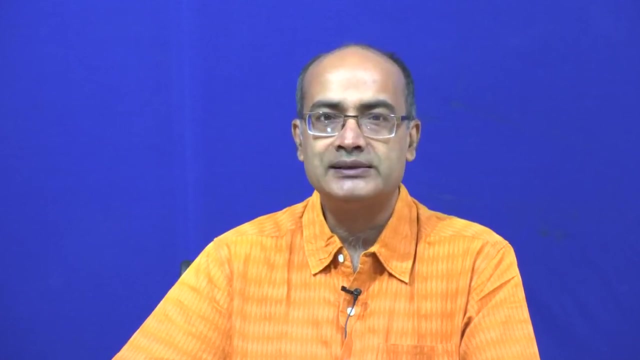 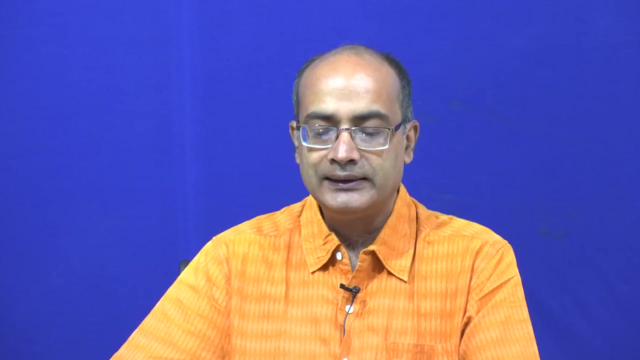 Just now we have told- taken up that example of EMG and we are explaining that how- that when we try to exert force using our muscle, that the activities will go up more and more time, that same muscle fibers should be excited and because of that that we will see that 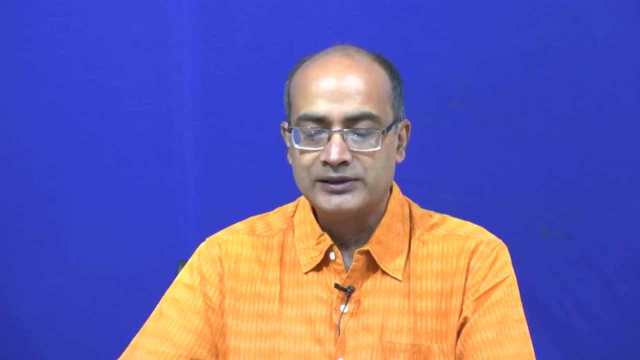 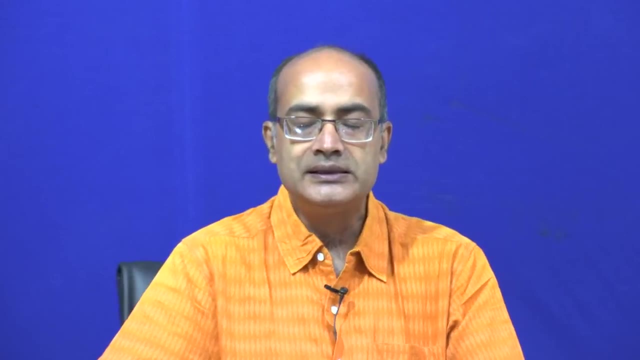 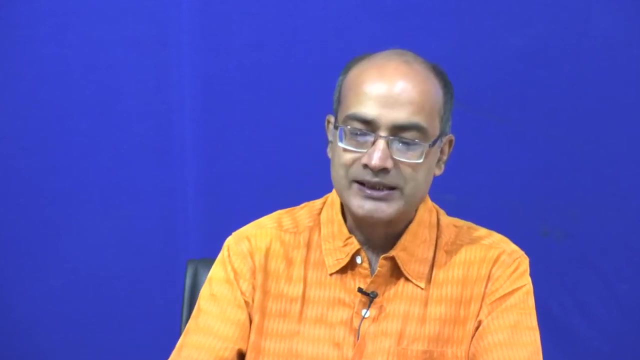 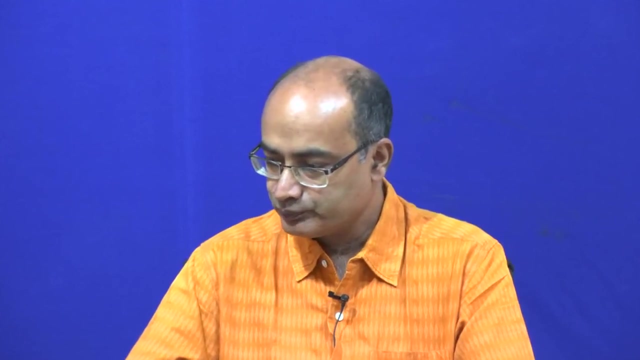 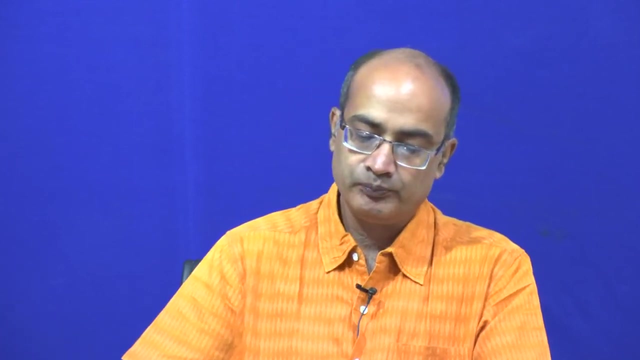 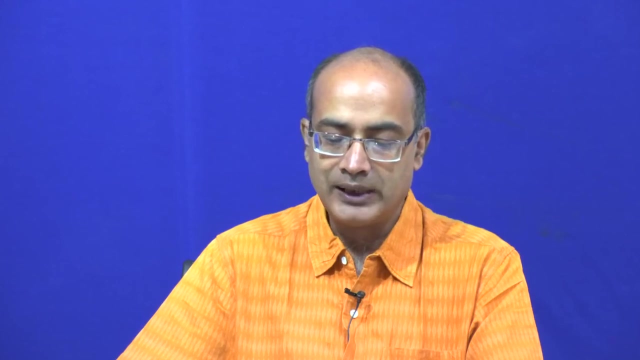 the turns count will change as well as the. as more and more muscle fibers are employed, then our- actually the intensity of the signal also will change. ok, So we just explain that. So I am just repeating that same thing. how can we determine fatigue of the eye? by analyzing? 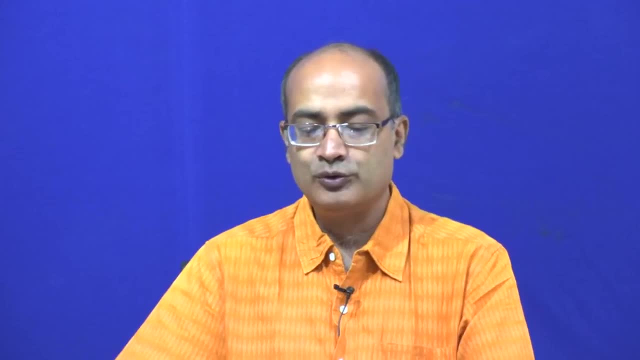 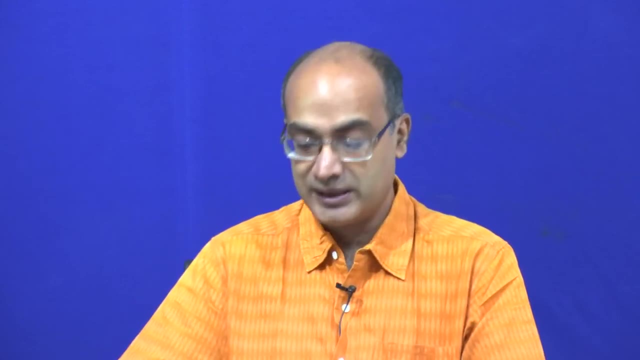 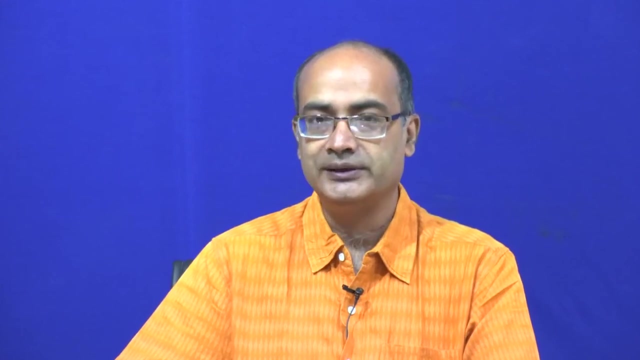 the eog signal. Ok, To do this, we need to look at the EOG signal. I have not worked with the EOG signal, but I can tell you the way that, how to proceed, the general way that, how to proceed with that. 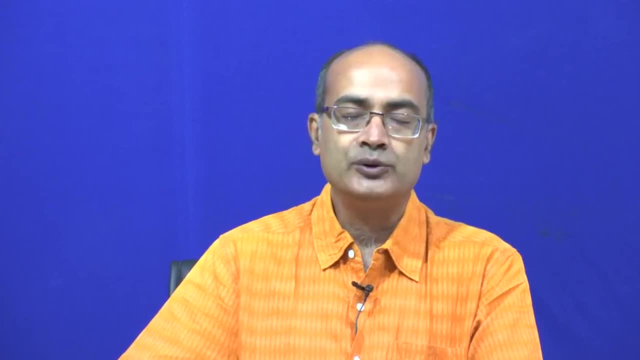 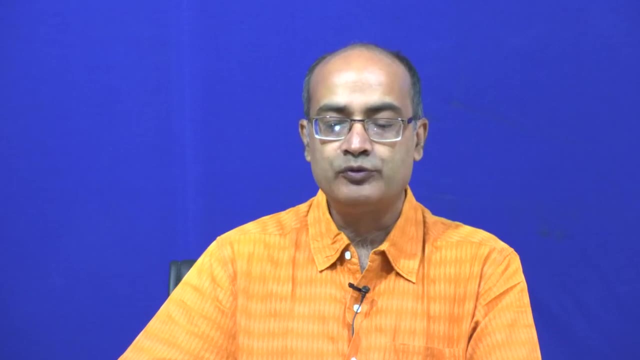 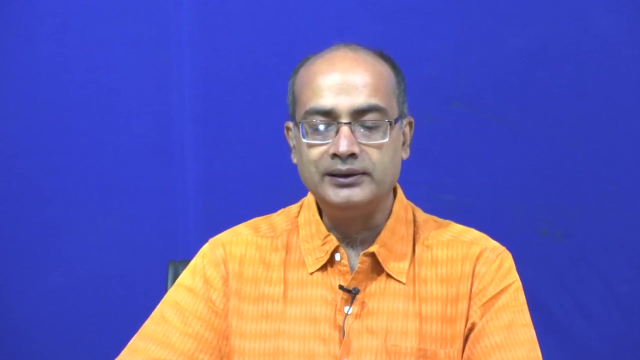 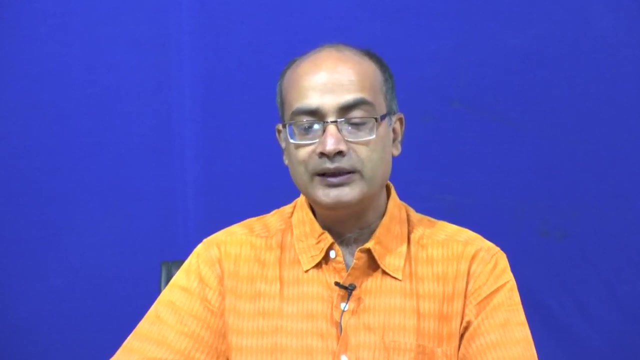 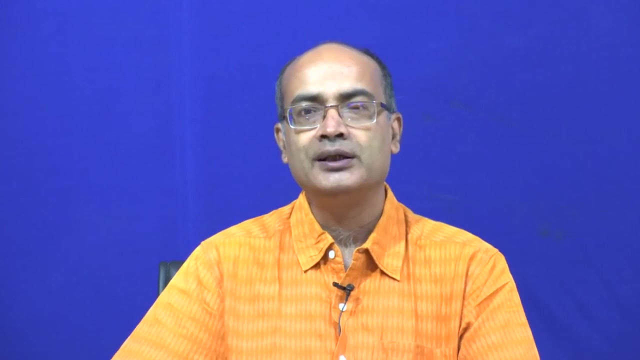 We should first look at the EOG signal, look at the nature of it and that first we should take from the normal subjects and see that how the signal pattern we get for normal subject in normal condition- Now when the fatigue happens, we need to see that changes. as human being we have much better. 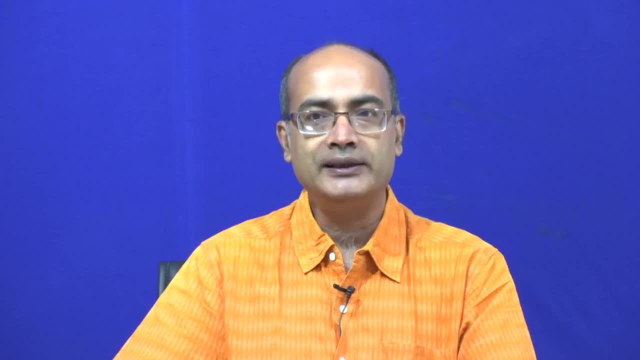 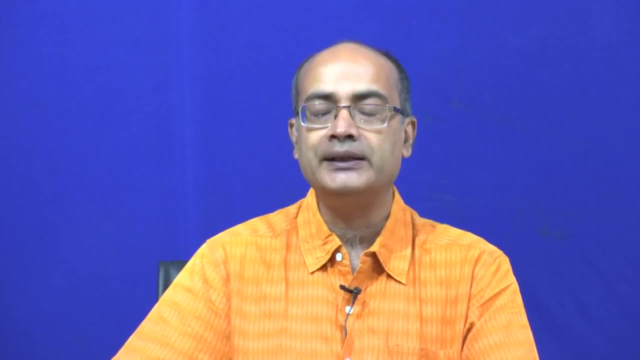 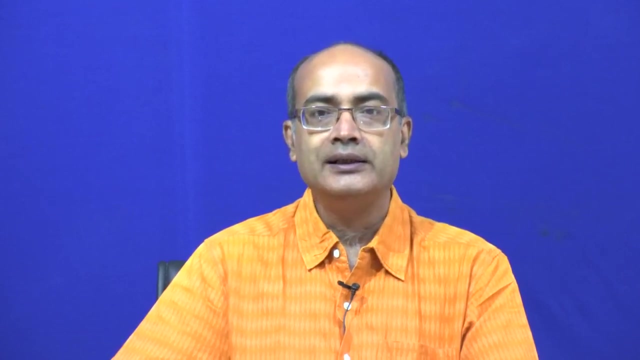 capability to look at the signal and find it out that what is the change. and I think to know that, To know more that what are the changes are happening in the signal, we should take the help of an expert and the clinicians or the doctors. they are the best people to help us.